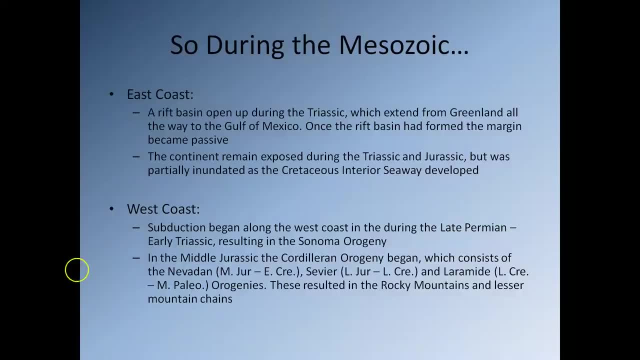 Cenozoic in the next lecture. All right, let's get going. So, during the Mesozoic, what was going on? Well, if you remember, on the east coast we had a big rift formed in the Triassic and that extended from Greenland all the way down to the Gulf of Mexico. Once the rift basin had formed the margin. 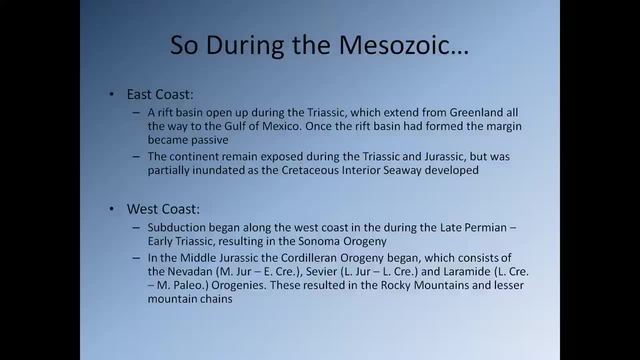 became passive. so, if you want the rift to become wide enough, the east coast of the United States- or east coast of North America, should I say, became a passive continental margin, just like it is now, and the continent pretty much remained exposed during the Triassic and Jurassic and portions 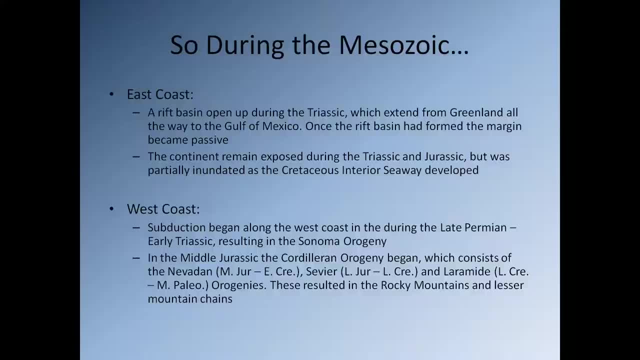 of it were not. So we're going to look at some of the things that happened during. the Triassic were partially inundated during the Cretaceous as part of the Zuni marine transgression. On the west coast, on the other hand, we had the beginning of subduction. Now the beginning of 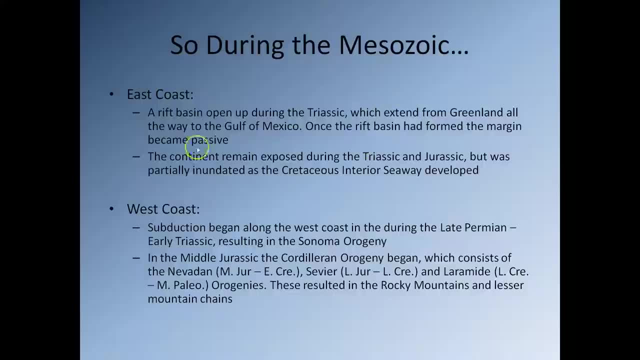 subduction was obviously associated with the start of rifting during the Triassic, because the rift that formed on the east coast started pushing North America westwards and obviously, in order to allow North America to move westwards, it had to override the oceanic crust of the Farrinham Plate. 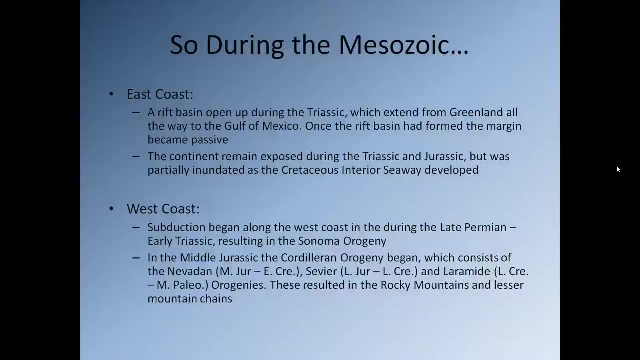 the Farrinham Plate was sitting to the west of North America during that time period. So as you're moving to the Mesozoic, we see the start of subduction. There's a little positive subduction in the late Permian, called the Sonoma Orogeny, but the main portion, the main part of the subduction- 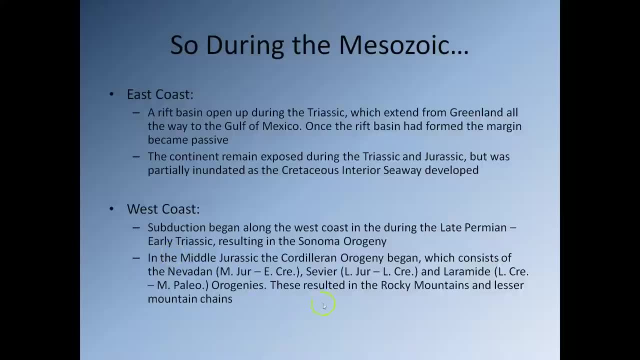 that occurs during the Mesozoic on the west coast is part of the Collierian Orogeny and of course that consisted of the Navardian, Sevier and Laramide Orogenies and once again that's caused by the North American Plate overriding the Farrinham Plate as North America gets pushed. 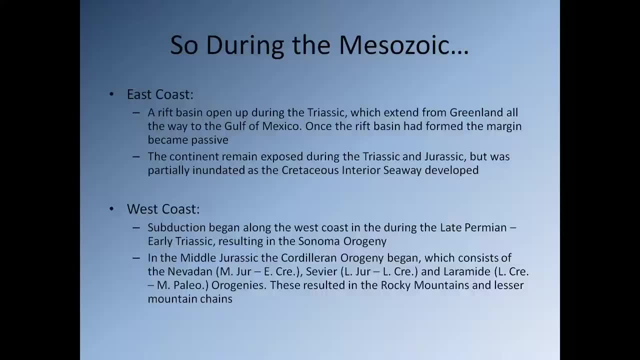 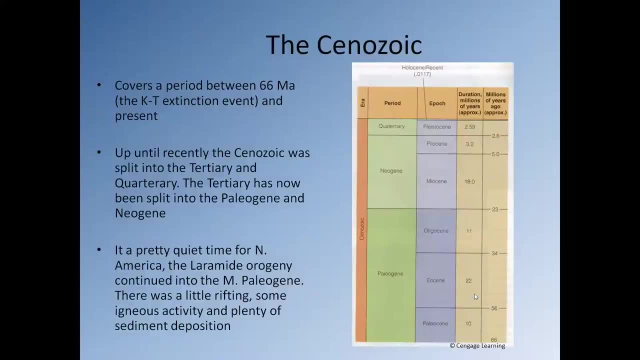 westwards. And of course this collision between these two huge chunks of crust resulted in the formation of the Rocky Mountains and a few other lesser mountainous chains. So the Cenozoic. so it covers a period between about 66 million years ago and the present day, So up until 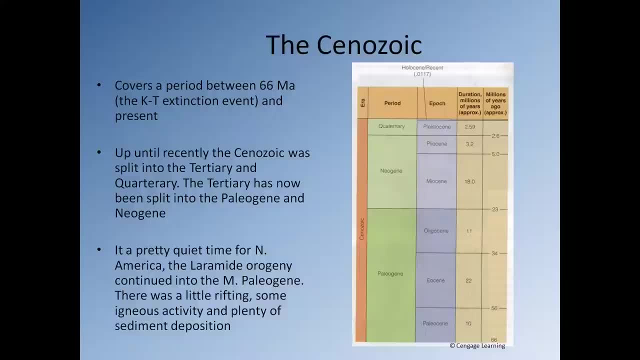 recently the Cenozoic was split into the Tertiary and the Quaternary. It says the Quaternary up here and the Tertiary was down here. The Tertiary has now been split into the Paleogene and the Neogene, So that's why it's called the Cretaceous-Tertiary boundary. 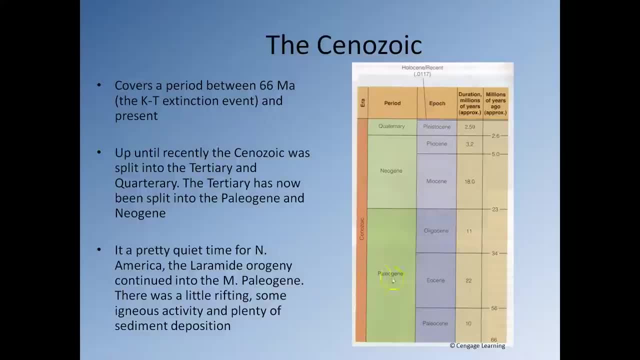 up here, but in fact the Tertiary doesn't really exist anymore because it's been split into the Paleogene and the Neogene. It's, on the whole, a pretty quiet time for North America. The Laramide Orogeny continues into the middle Paleogene around here, at which point it comes to a stop. 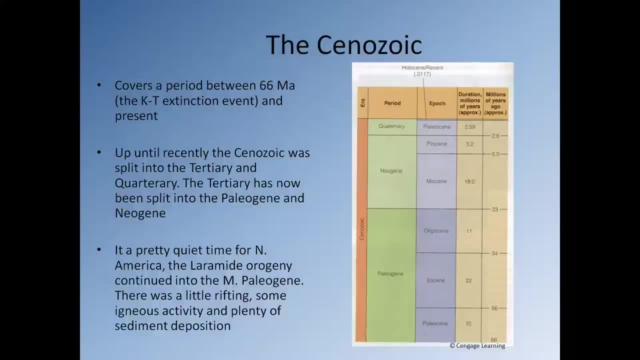 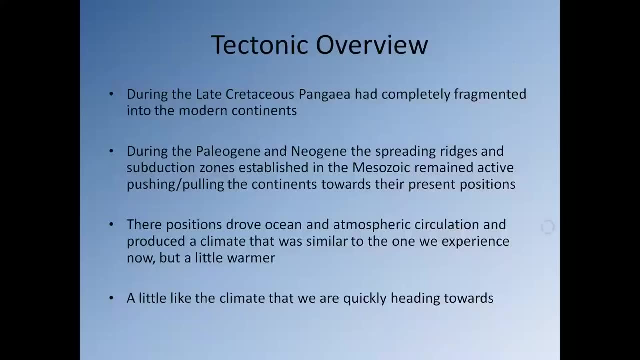 and there was a little bit of rifting, some igneous activity and plenty of sedimentary deposition, But on the whole, relatively calm for North America during this time period. So what's the tectonic overview? Well, during the late Cretaceous Pangaea had completely 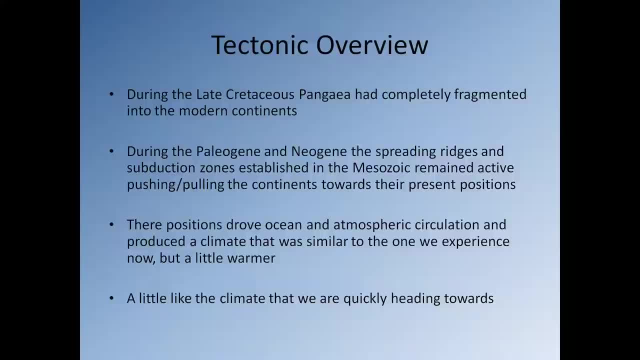 fragmented into the modern continents and during the Paleogene and the Neogene, the spreading ridges and subduction zones which were established in the Mesozoic remained active and of course, that meant they were pulling back. So the Paleogene and the Neogene were pulling back. 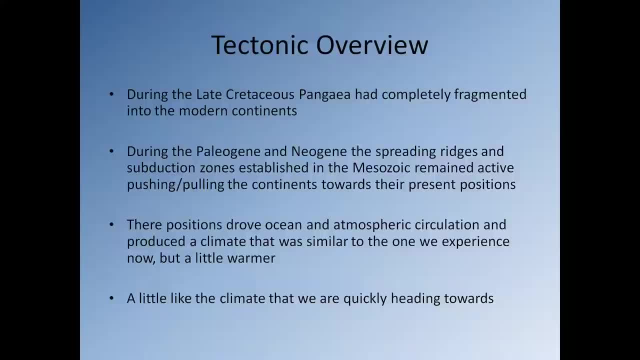 and pushing the continents towards their present positions. So throughout the, throughout this Cenozoic, essentially all the continents are migrating towards the regions that they are in now. So of course, as we already discussed, the change in the position of the continents drove changes in ocean and atmospheric circulation and of course this produced 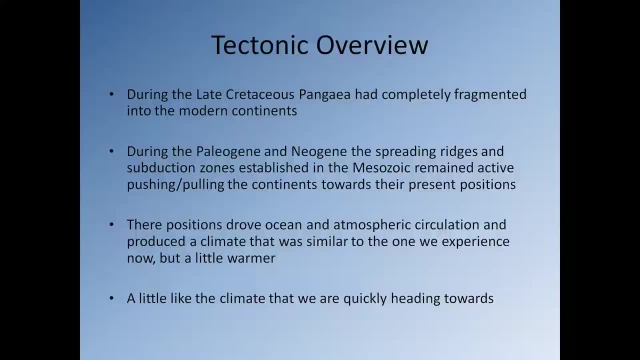 very substantial climatic changes, especially during the Cretaceous and into the Cenozoic, and essentially it means that during the Cenozoic the global climate would have been similar to the present global climate. however, it would have been warmer. So we would have expected, you know we could expect the same kind of patterns, you know. 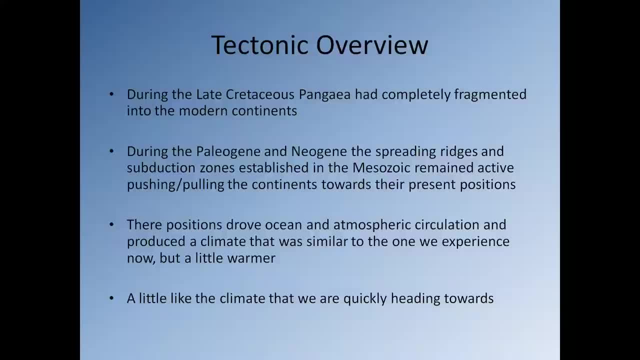 even the, you know high in northern and southern latitudes. we would expect- you know conditions, like you know- relatively cool. you know wet summers and relatively cold, wet or snowy winters, for instance. you know, whilst at the tropics conditions would remain tropical, However, the temperature would be a little higher during the Cenozoic and the Neogene. So we would expect the same kind of 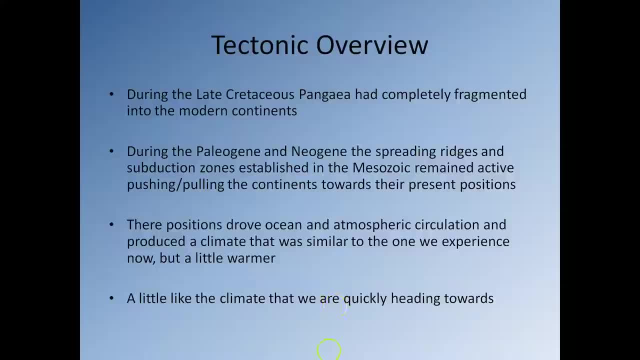 changes to occur in the Cenozoic and the Neogene, at least the early to mid Cenozoic. So the climate that would have been experienced during the Cenozoic is a little like the climate we're heading towards now, as global temperatures do appear to be on the rise. 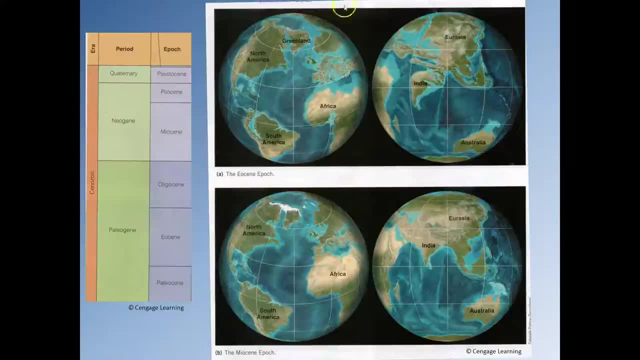 So this is the basic situation. so we have a couple of diagrams here. you can see that this is during the Eocene epoch, that's here during the middle Paleogene. We can see that the continents are, on the whole, approaching their current positions. Australia needs to come a little bit north. 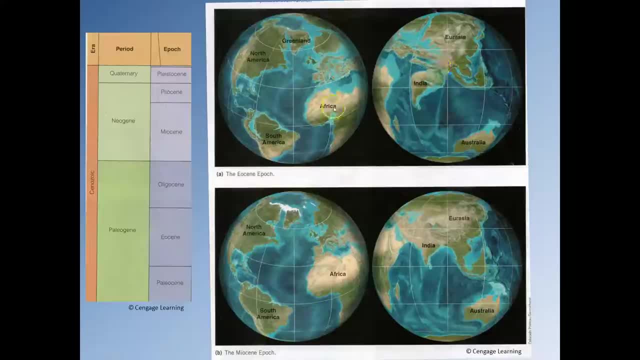 India has only just begun its collision with Asia. we can see that Europe still isn't fully formed yet we can see that all these little pieces of continental crust still need to go crashing into each other to actually form the main mass of continental Europe. We can see South America still. 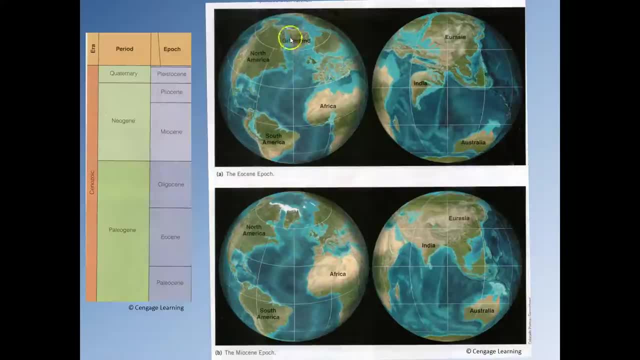 isn't joined to North America via Central America yet, and we can see that Greenland is maybe just about hanging on to the side of North America. maybe just What you'll notice, though, is everything is pretty much where we expect it to be, although when you look at the coastlines, let's look at North. 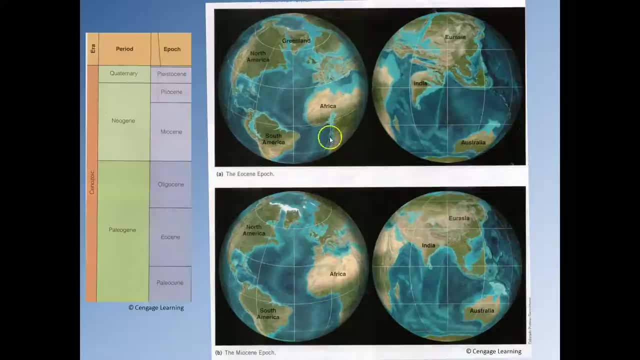 Africa. here, for instance, you can see that large portions of the coastline are inundated, and this is because during the Eocene epoch, as I said, that the global climate was still relatively warm. that meant there was no ice cover, either the North or the South Pole. this meant there was more water. 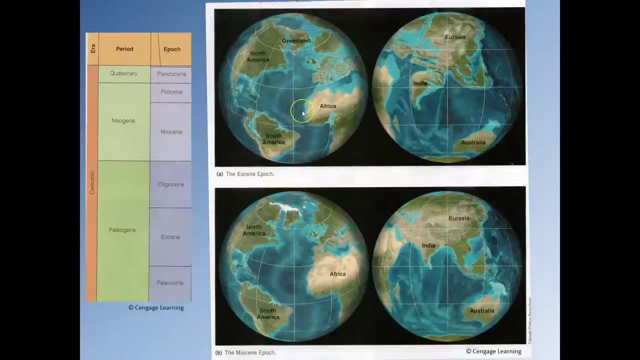 in the ocean basins and so coastal regions during this period- well, modern coastal regions, should I say- were inundated. By the time we get into the Miocene, that's, the lower to middle Neogene, we see that global sea levels have dropped because we start to see the formation of ice caps. that starts locking up. 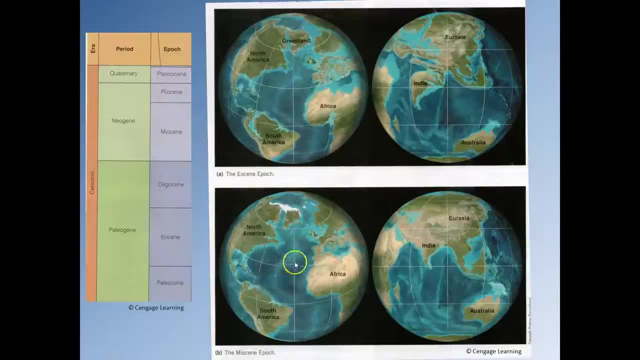 water, and so that means that water cannot return to the ocean basins, so global sea levels go down. You will also notice by this point that Europe is now nearly fully formed, so all these little pieces of continental crust here have now crashed into each other to form the main bulk of 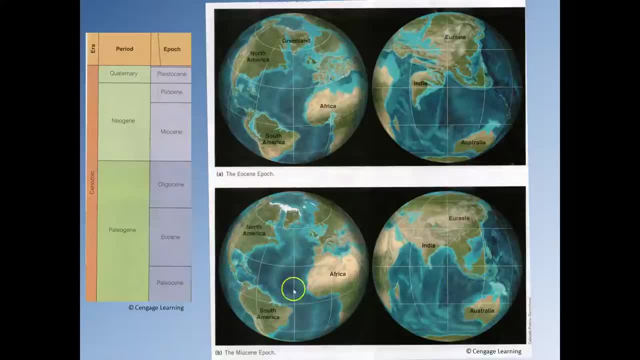 continental Europe and on the whole it looks pretty straight forward. you can see it: at the moment Indonesia is currently joined to Thailand here. that's going to change over time, and Australia is still working its way steadily north and it's nearly at its current position. 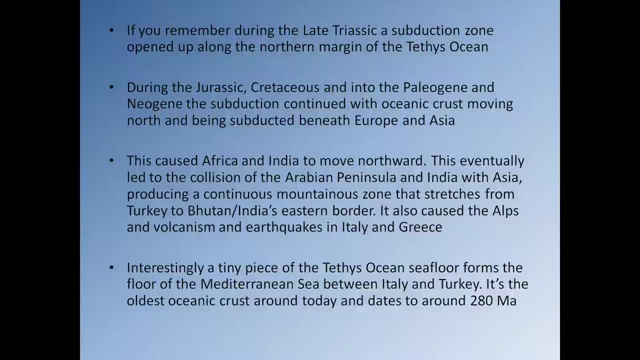 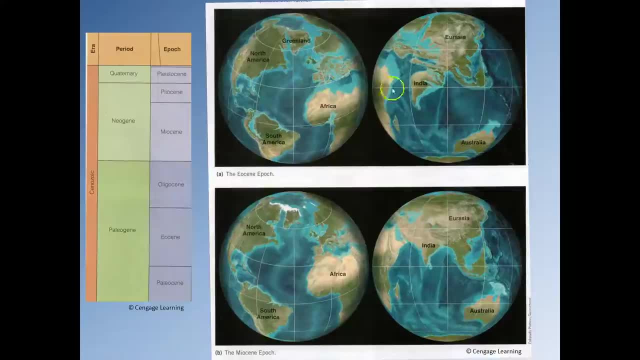 So, if you remember, during the late Triassic a subduction zone opened up along the northern margin of the Tephys Ocean. so, if you remember, the Tephys Ocean was a body of water about here where the modern Indian Ocean sits. So the subduction zone opened up along the northern margin and it took all this oceanic crust here. 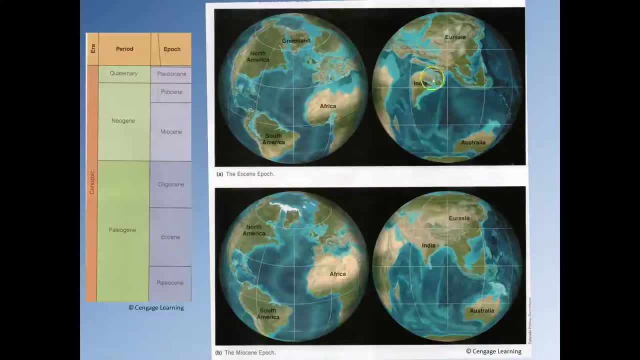 which was part of the Tephys Ocean Basin, and it began to subduct it in the northward direction underneath Asia, and, of course, one of the results of that was that India, which was sitting on this Tephian oceanic crust, was pulled north along with it, and eventually it ends up crashing into Asia. 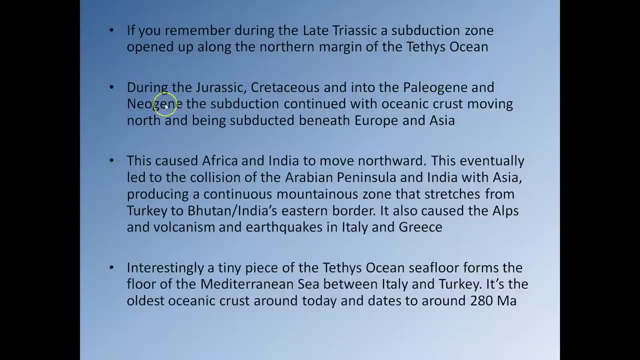 to produce the Himalayas. So during the Jurassic Cretaceous and into the Paleogene and Near-Gene as well, the subduction continued, with oceanic crust moving north and being subducted beneath both Europe and Asia. So this caused Africa and India to move in a northerly direction and this eventually led to the collision of the. 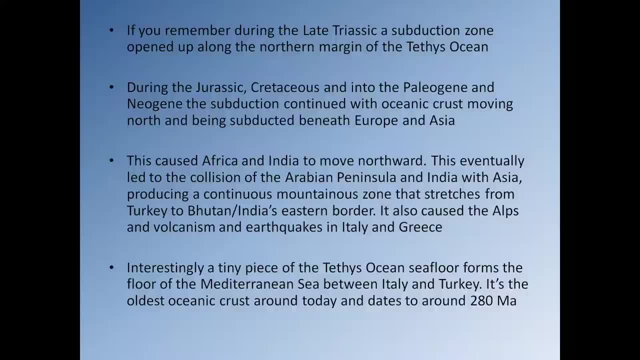 Arabian Peninsula and India, with Asia producing a continuous mountainous zone that stretches from Turkey to essentially India's eastern border. you know approximately where the Kingdom of Bhutan is located. So, in terms of what's going on in Europe, the movement of Africa northwards has been steadily causing a significant defamation along the 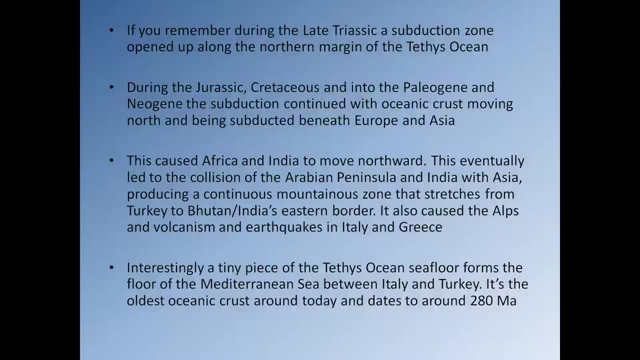 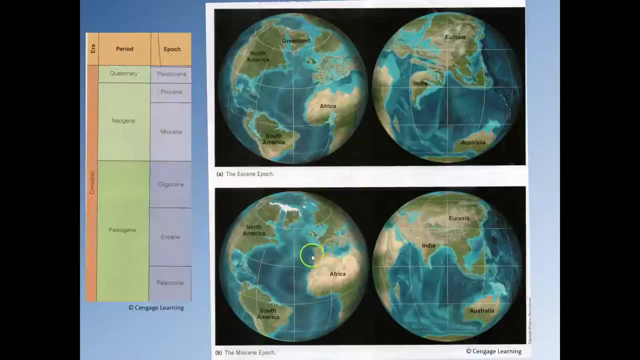 southern margin of Europe that, combined with the accretion of all these little pieces of continental crust here, led to the formation of a very large mountain range that goes across the entirety of southern Europe, which, of course, is referred to partially as the Alps. 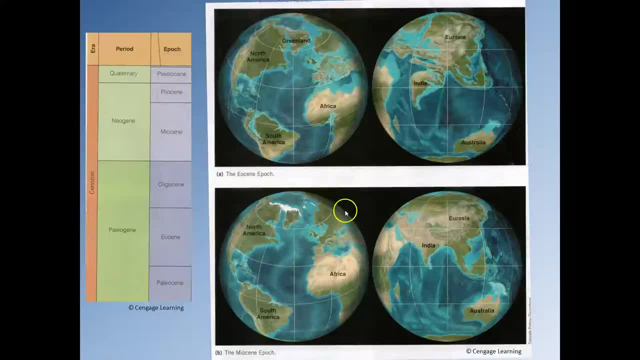 There are actually several little mountain ranges that make it up, But the end result is this subduction zone that comes all the way from, started all the way over here in Asia, came all the way through here, all the way along South Asia, all the way along the. 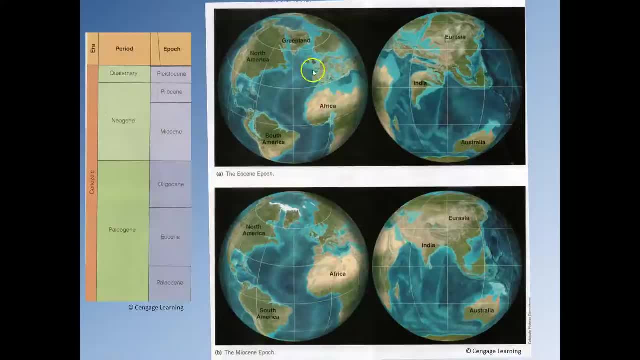 south coast of Europe resulted in the formation of a chain of mountains that goes from the Pyrenees between Spain and France all the way through Europe, into the Middle East and then into Asia, And, you can even argue, maybe down into Thailand as well. 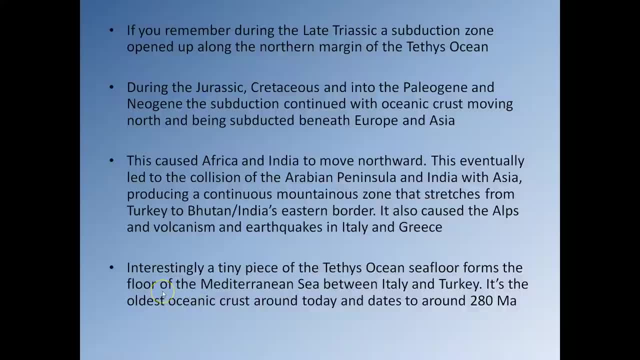 So, interestingly, there is a very, very small piece of this Teffian seafloor that's still around. it's the only bit that's left. It forms a small part of the Mediterranean Sea and it's stuck between Italy and Turkey. 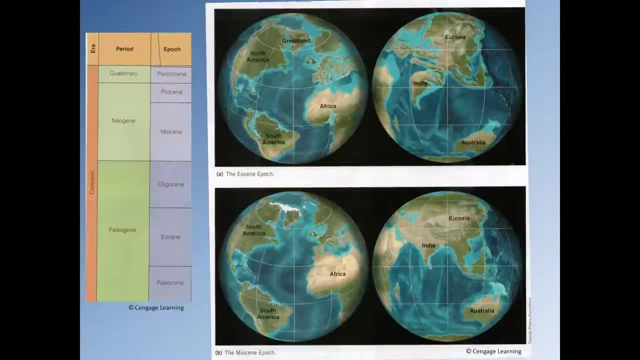 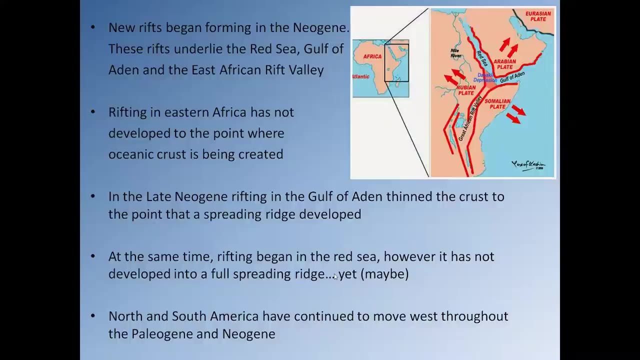 And it's the oldest oceanic crust around today and it dates to around 280 million years, so it's located approximately here. It will take a little bit. So do we see anything else going on in terms of large-scale structures? 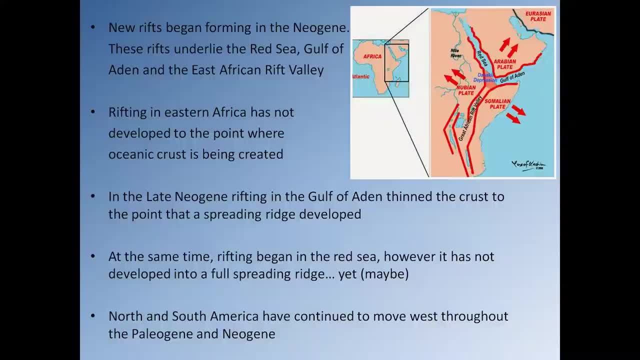 Well, yes, we see new rifts beginning to form in the Neogene, and these rifts underlie the Red Sea, the Gulf of Aden and the East African Rift Valley. So what we're seeing is in the Neogene, we begin to see the start of the formation of these three areas. 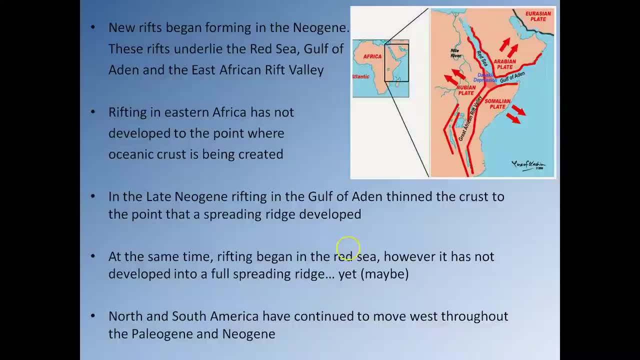 The Red Sea, the Gulf of Aden and the East African Rift Valley. So the Red Sea is located here, the Gulf of Aden is located here and the East African Rift Valley is located here, And so, of course, this is the result of the movement of the Somalian Plate away from Africa. 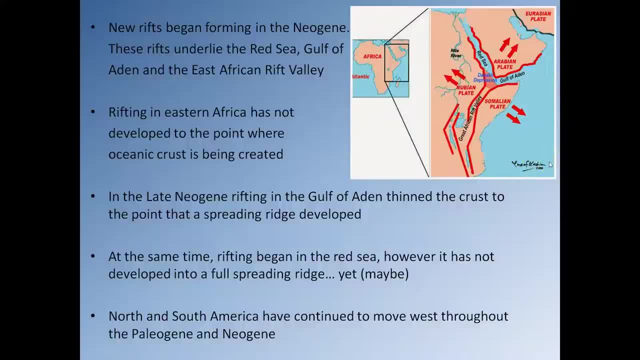 The Somalian Plate is currently trying to move off. It's trying to move off into the Indian Ocean in an approximately eastward direction. It's also the result of the opening up of rift valleys here and here. So the Arabian Peninsula is being pushed this way. 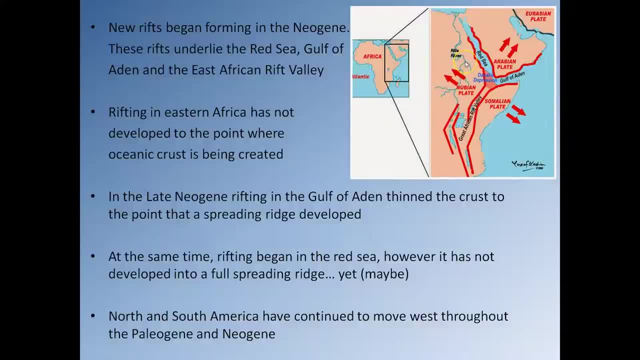 The Red Sea opening up is trying to push Africa eastwards. Of course it's not going to win And in the case of the Gulf of Aden, we have a fully formed rift that's pushing the Arabian Peninsula northwards And that's also helping to push the Somalian Plate southwards, or more accurately, southeastwards. 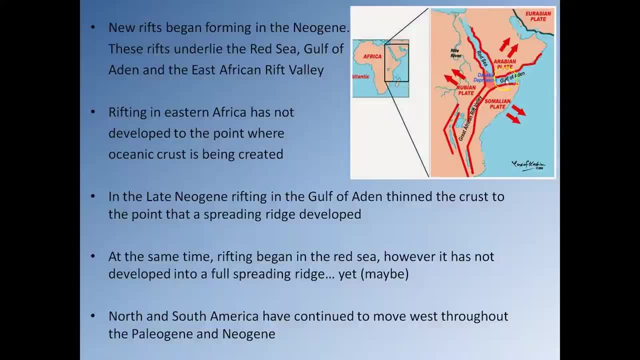 So it's the formation of the Gulf of Aden Rift that seems to do most of the damage. So as the Gulf of Aden Rift opens up, it applies a northerly push to Arabia. Now, remember, Arabia is already moving north-northeast. 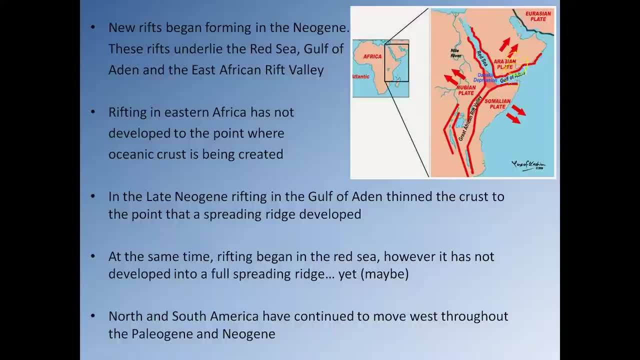 And so the formation of the Gulf of Aden also gives an additional northerly push, And so that's causing the Arabian Peninsula to begin to essentially pivot- The pivot's around here- and it's causing the southern and eastern portion of the Arabian Peninsula 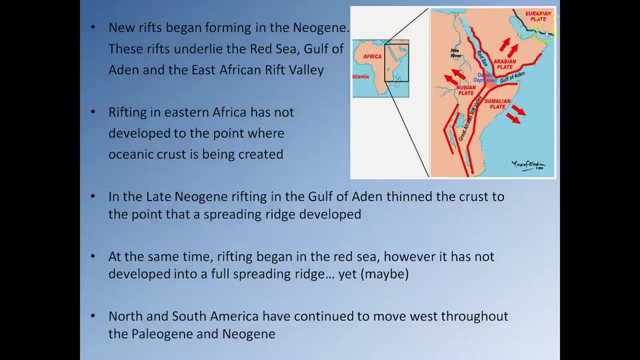 to move up in this direction, They'll eventually crash into the area which is now modern-day Iran, And this movement of the Arabian Peninsula being pushed up this way obviously puts this region across here under extension and leads to the formation of a rift valley which we see as the Red Sea. 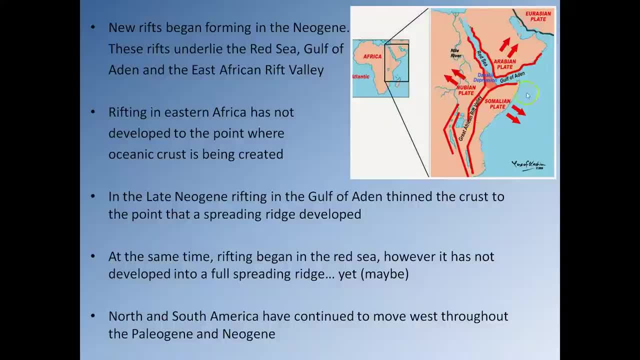 Now, also because the Gulf of Aden is pushing on this portion of the African Plate southwards, obviously it begins to make the Somalian Plate want to move southwards And, of course, as it begins to push the Somalian Plate in the southward direction, 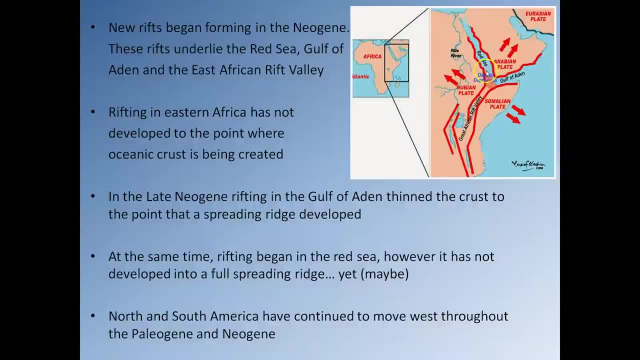 it starts to put the area across directly behind the Somalian Plate under extension and that leads to the formation of the East African Rift Valley. So both the Red Sea and the East African Rift Valley are generally formed in response to the formation of the Gulf of Aden and the spreading that it produces. 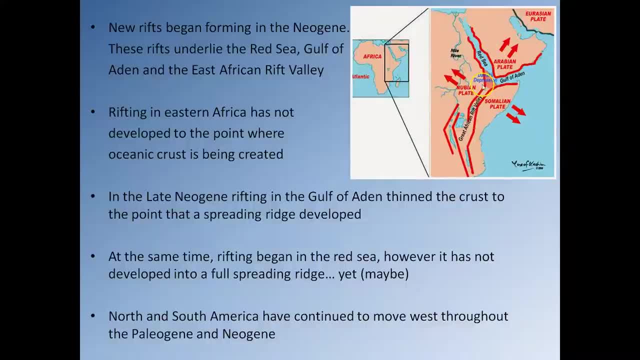 So, in the case of the Red Sea and the East African Rift Valley, they're not fully formed rift valleys yet. They're not fully formed rift valleys yet There isn't, you know, new oceanic crust being formed. However, in the case of the Gulf of Aden, it's a fully mature divergent plate boundary. 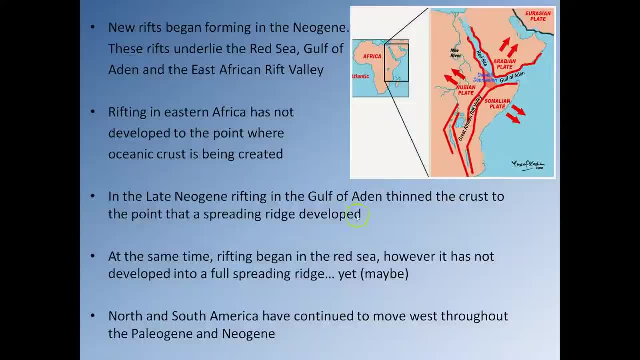 where new ocean crust is being produced. In terms of what's happening with North and South America during this period, we see that North America and South America have continued west throughout the Paleogene and the Neogene, doing pretty much what they're doing now. 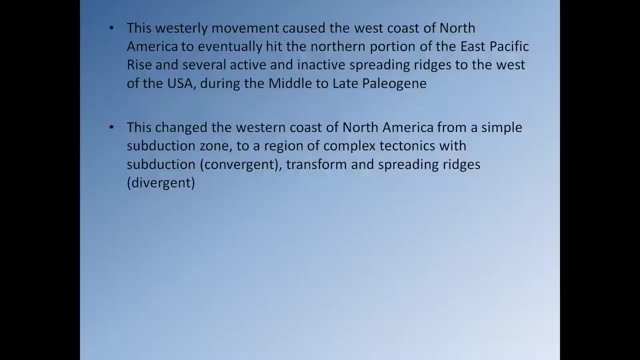 So this westerly movement of North America and South America of course eventually led, in the case of North America, to the northerly portion of North America hitting the north portion of the East Pacific Rise. So the East Pacific Rise is a divergent plate boundary that sat off the west coast of North America. 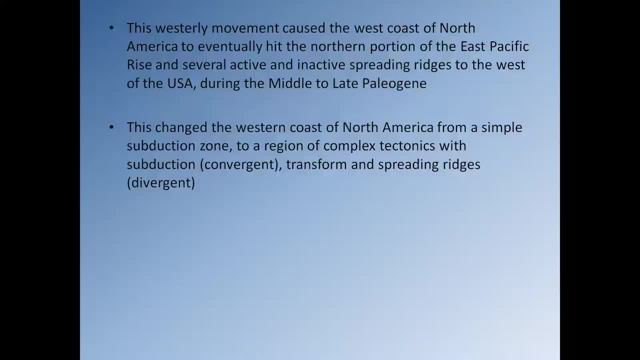 and that's where the Farallon Plate, or new crust to make up the Farallon Plate, was being formed. However, eventually, North America kept moving westwards and eventually it began to subduct that spreading ridge down into the mantle underneath North America. 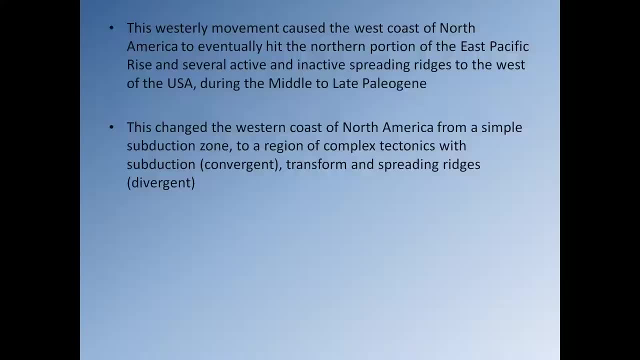 And, of course, this led to a very significant shift because it meant that we no longer had subduction taking place on the west coast because the divergent plate boundary was gone. It meant that we instead shifted to a regime that led to transform plate tectonics. 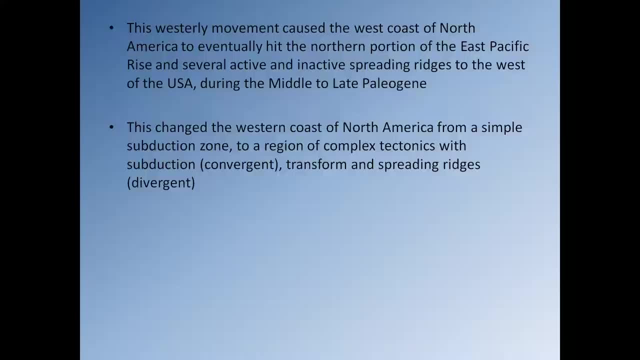 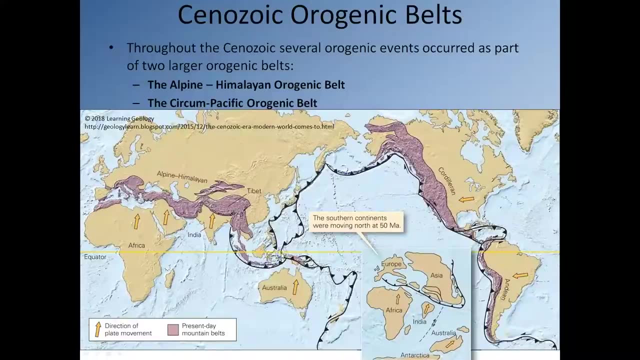 and the formation of the San Andreas Fault, And you'll see that summarised in a few diagrams in a few slides' time. So, yeah, Alright. so in terms of the Senazerc Orogenic Belts, what's going on? 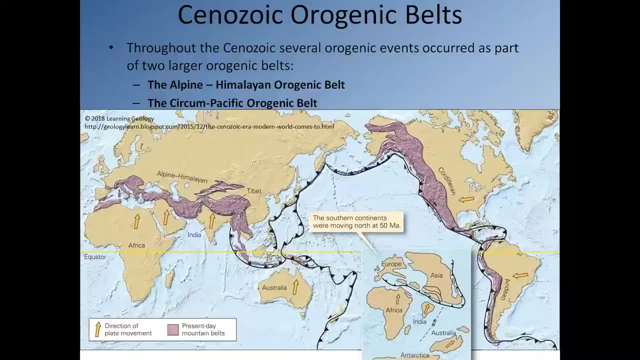 So throughout the Senazerc there are several orogenic events or mountain building events that occur as part of two broad orogenic belts. The first one is the Alpine Himalayan Belt and of course, as I said, that stretches from the Pyrenees over here between Spain and France. 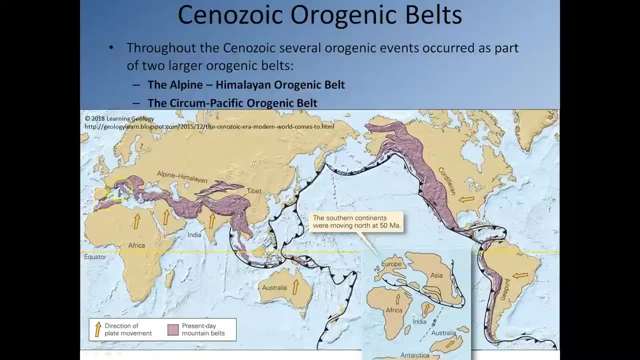 you have the Atlas Mountains over here in northwestern Africa. it goes through central Europe, into the Mediterranean, into the Middle East via Turkey, through Iraq, into Iran, into Pakistan and of course then into the Himalayas. You know, you've got the Tibetan Plateau. 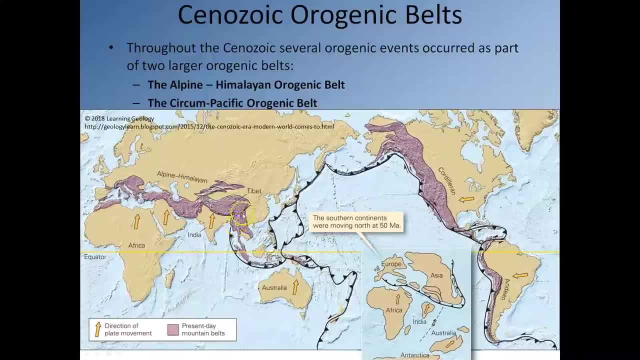 And of course it also comes down in a weaker form down here, into Thailand and then into Indonesia, And you can claim that all of this belt of mountains here is essentially the result of the subduction zone that ran all the way along here. 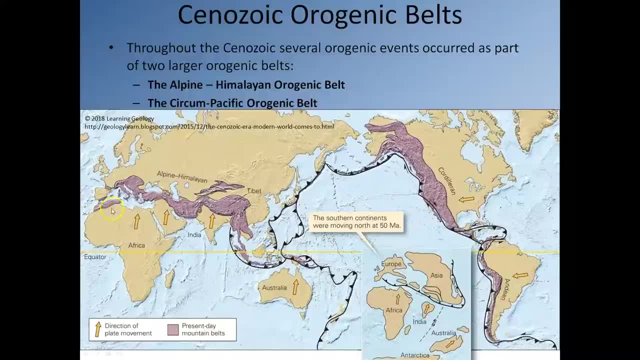 And of course that led to the subduction of the Tefes Ocean Crust underneath Europe and North America, the movement of Africa northwards and the movement of India northwards. So that's one of the belts. The other belt is referred to as the Circumpacific Orogenic Belt. 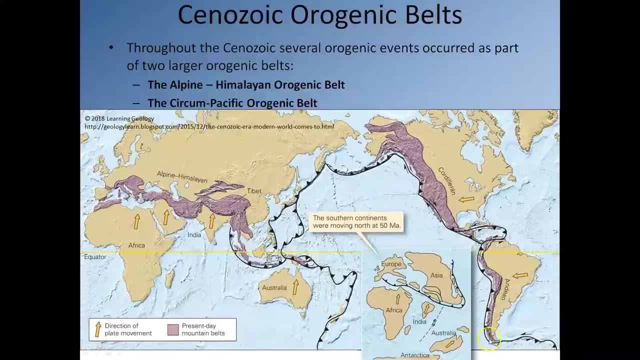 and that stretches all the way from the southern tip of South America up through South America, through Central America, into North America, across the Aleutian Island, Arc, and then down along the east coast of Asia, so down through Japan, and then it diverges here. 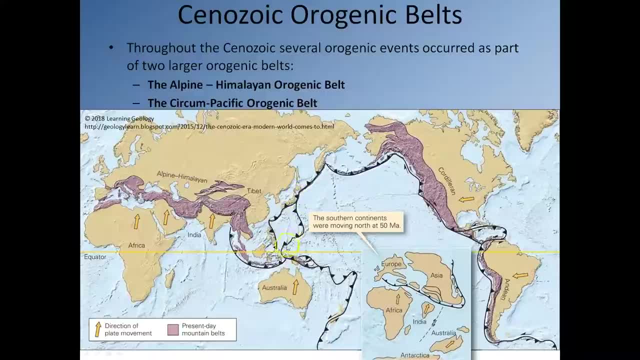 one limb going down into the Philippines, one limb sitting off into the middle of the Pacific Plate, Then it comes down here through Papua New Guinea and then comes around via Tonga, Fiji and then eventually down towards New Zealand. And so, once again, this is the result of large-scale subduction. 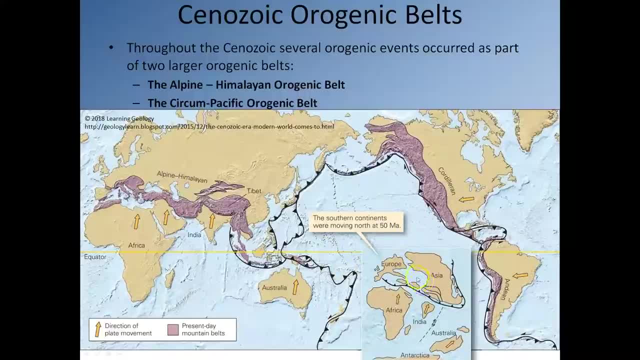 as the Pacific Plate is moving in approximately north-westward, north-slash-westward direction And of course, that's making the Pacific Plate subduct underneath North America up here and Asia over here. OK, in terms of what's happening in the case of South America. 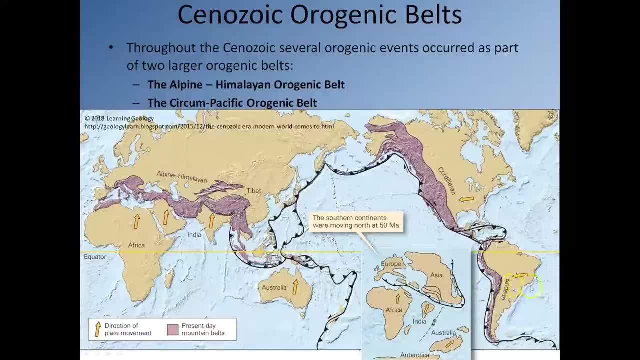 we have the Nazca Plate over here. That's subducting westwards underneath South America And in terms of North America, because the Pacific Plate is moving in a north-westward direction. it means the Pacific Plate has to move past the North American Plate. 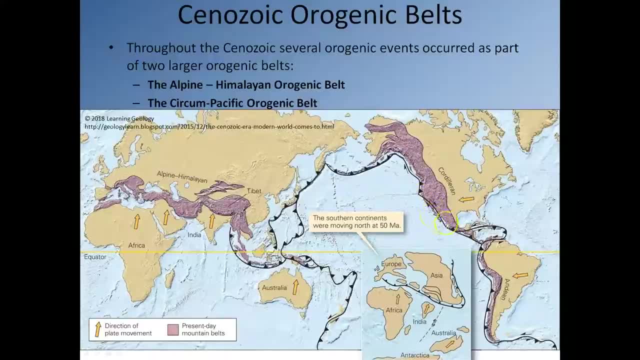 That leads to the formation of the San Andreas Fault here and the formation of the Queen Charlotte Fault here. They're both transform faults, So that's essentially where the Pacific is just moving past North America, And so this is why we have to have this shift from subduction. 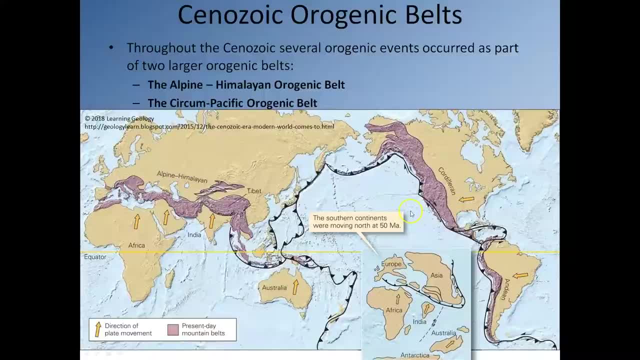 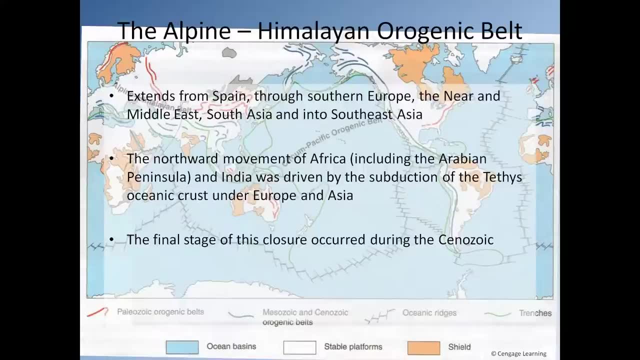 to transform plate tectonics, which will be described in greater detail in a little while. So, in terms of the Alpine Himalayan Arginine Belt, it extends from Spain through southern Europe, the Near and Middle East, South Asia and into Southeast Asia. 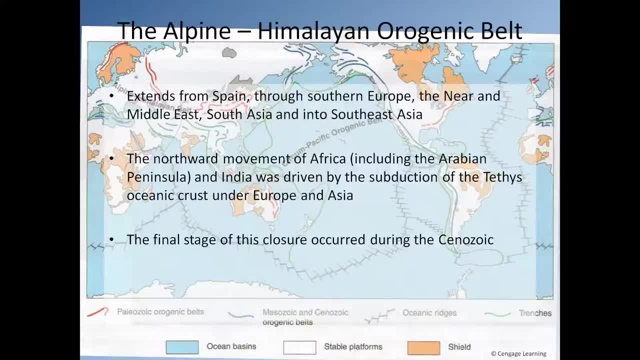 So it's a very substantial belt. So, of course, it's the result of the northward movement of Africa, including the Arabian Peninsula and India, And this was driven, of course, by the subduction of the Tephys Oceanic Crust under Europe and Asia. 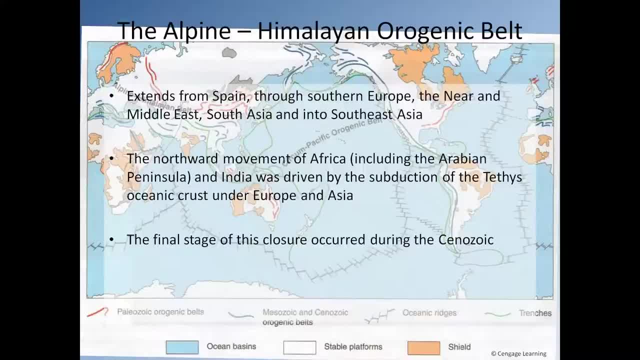 So the final stage of this closure occurred during the Cenozoic. You could argue it's still going on now because Africa hasn't actually finished crashing into Europe. Eventually, Africa will completely crash into Europe and the two continents will suture together to form one landmass. 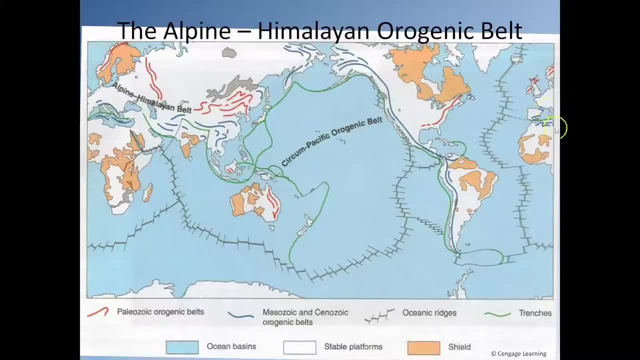 And so you can see, this is the belt here. So here's Spain and France over here. You can see, the belt goes all the way from here, all the way through southern Europe, into the Middle East and then into, of course, the area we would refer to. 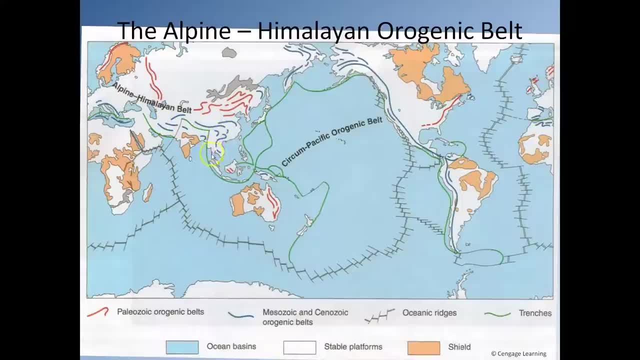 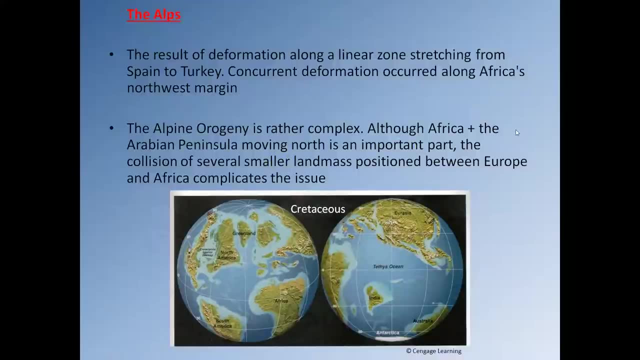 as the Tibetan Plateau and the Himalayas, and then down into Thailand and down into Indonesia. So let's talk about the Alps. So the Alps are the result of deformation along a linear line stretching from Spain to Thailand, Turkey. give or take a little bit. 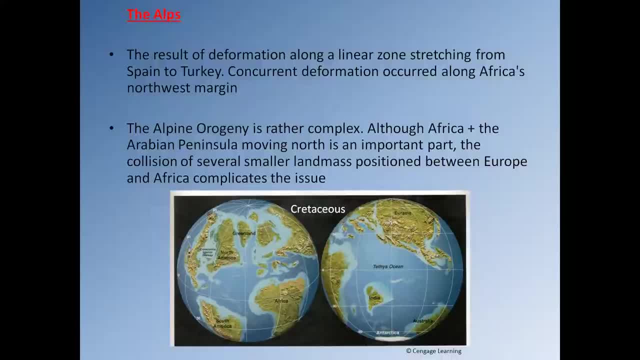 So we get concurrent deformation occurring along Africa's northwest margin. So, of course, as Africa moves northwards, the south coast of Europe begins to experience compressional forces. Now Africa begins to apply compressional forces onto the south coast of Europe. 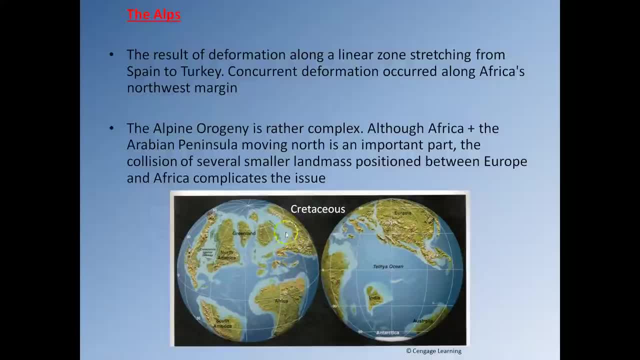 but of course it also works the other way. As Africa moves closer to Europe, Europe also begins to apply compressional forces onto the north coast of Africa. So this means we get deformation on both sides of this basin as it begins to close. 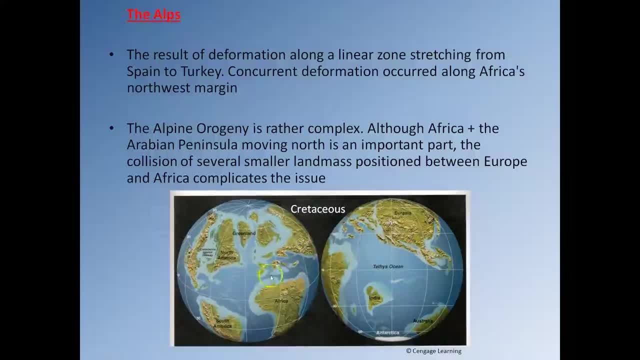 Most of the damage is done in Europe. However, in Africa we do get a little bit of deformation associated with Africa's steady northward movement. Now, the reason that the Alpine Orogeny is rather complex is, Excuse me. Let's try that again. 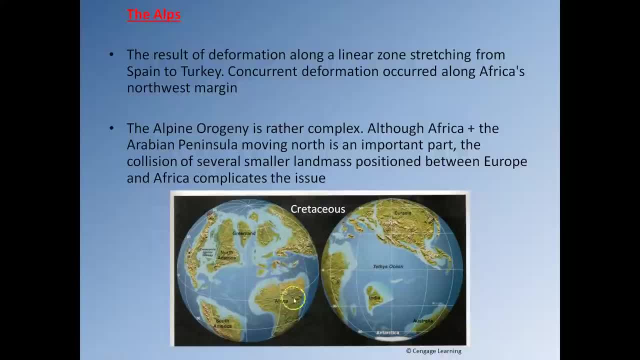 So, as you can see, we have lots and lots of little pieces of continental crust situated between Africa and what is now modern-day continental Europe, And as Africa moves northwards, it's going to push all of these pieces of continental crust into the main mass of Europe. 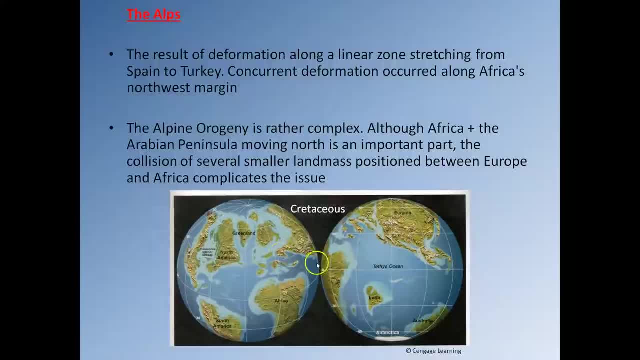 Of course. don't forget there's a subduction zone running along here. It's going to take all these pieces of continental crust and smash them into the bottom of Europe. That leads to the formation of multiple small mountain ranges which are all combined together into the Alpine Orogeny. 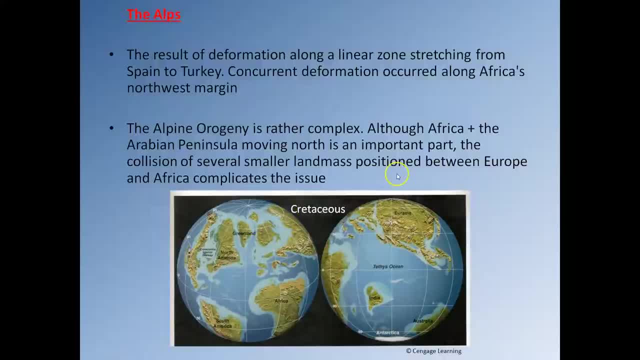 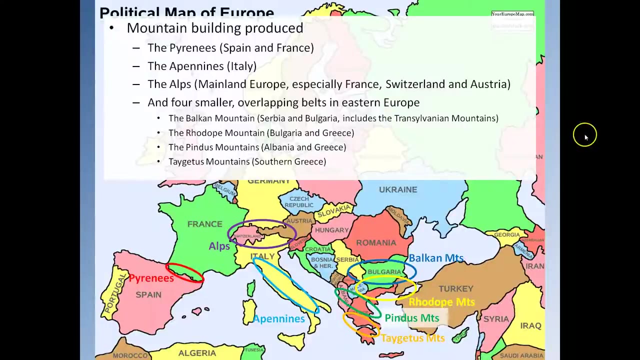 So it's a rather complex orogeny. So, although Africa and the Arabian Peninsula moving north is the important part, the collision of several small land masses positioned between Europe and Africa helped to make the Alpine Orogeny extremely complicated. So let's just actually go through some of these small collisions. 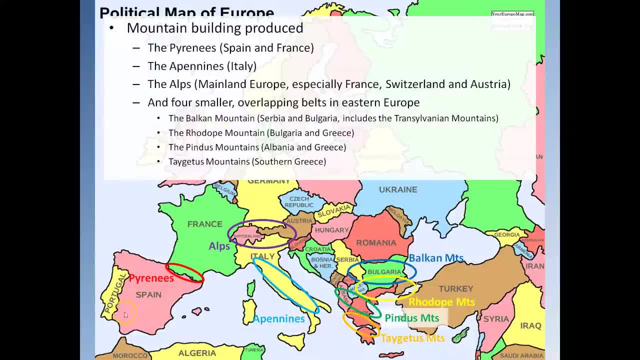 So, obviously, the one we've discussed so far is, of course, the Pyrenees Mountains. That's where Spain hits France, creates a mountain range that's marked out here in red. We obviously have the formation of the Alps themselves. 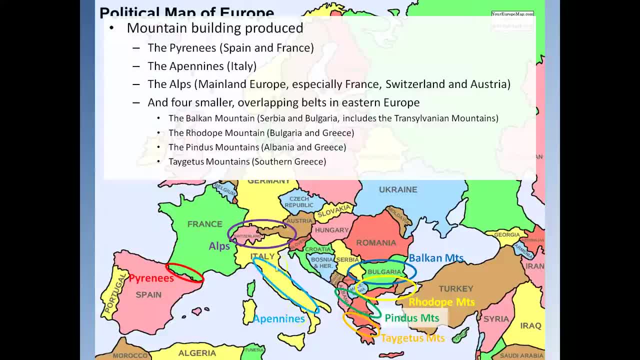 We have several pieces of crust that make up modern-day Italy, hitting southern Europe. That leads to the formation of the Alps, marked out here in purple. We obviously have the formation of the Apennine Mountains, which run down the length of Italy. 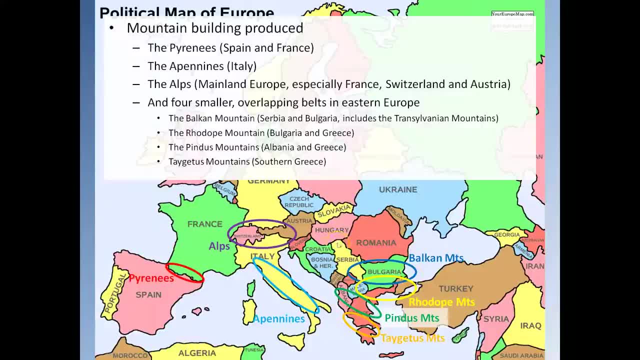 That's also related to several small collisions. And then over here in southeastern Europe we have multiple impacts forming both the Balkan Mountains, marked out here in blue, the Rodent Mountains, marked out here in yellow, the Pindus Mountains in green. 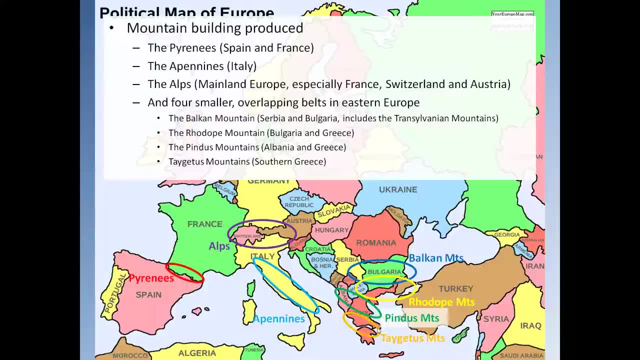 and the Tagentis Mountains in orange, And each one of these small mountain ranges is combined together to form the Alpine Orogeny, and they are the result of little pieces of crust hitting the south coast of Europe, one after another, after another, producing small mountain ranges. 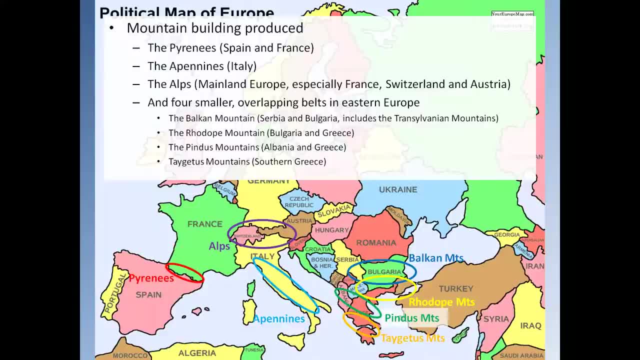 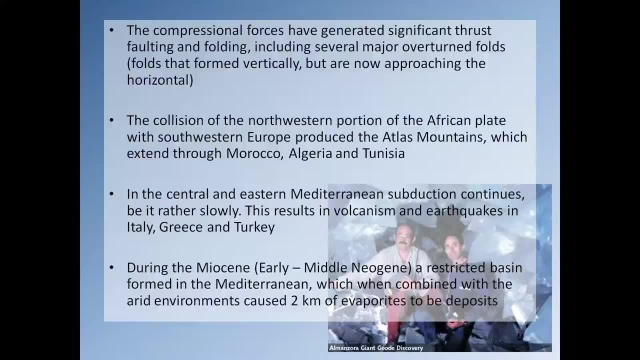 as I said, which are combined to give us the Alpine Orogeny. So the compressional forces have generated significant thrusting and folding, including several major overturned folds. those are folds that were once upon a time vertical and have now been pushed to near horizontal. 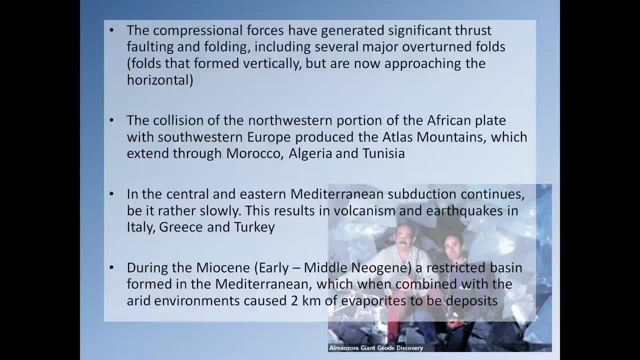 So that's essentially a reflection of the forces involved. So essentially, when you compress a piece of rock, initially the fold will stand upright. As you push the piece of rock further, the fold will begin to move until it becomes overfolded. 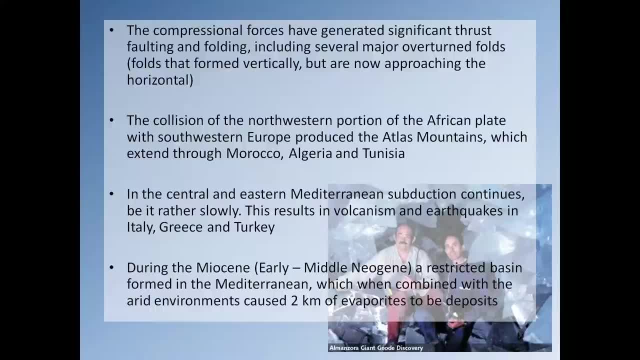 and then eventually, as it heads towards the horizontal, it will become recumbent, And so the fact that we have several major overturned folds, that tells us that these compressional forces have been going on for a very long period of time and it ended up with these folds being pushed to near horizontal. 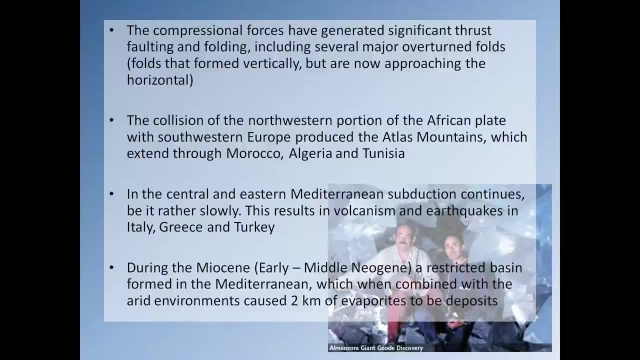 So the collision of the northwest portion of the African Plate with southwestern Europe produces the Atlas Mountains in Africa, and the Atlas Mountains extend through Morocco, Algeria and Tunisia. In the central and eastern portions of the Mediterranean we get subduction continuing even now, although it is rather slow. 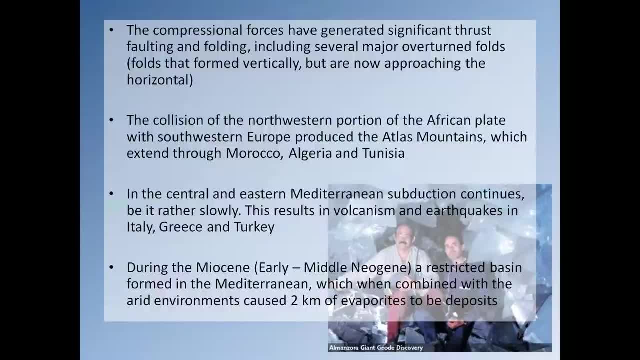 and it's a little bit chaotic. but the presence of these subduction zones does help to explain why we have volcanism and earthquakes in countries like Italy, Greece and Turkey. So during the Miocene, that's the early to middle Neogene. 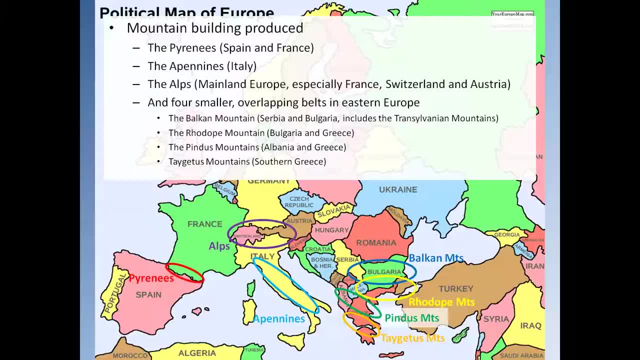 we actually see, the Mediterranean becomes a restricted basin. so the Strait of Gibraltar here, which separates Spain from Africa, essentially closes up, cuts the Mediterranean off from the Atlantic over here, and so the Mediterranean becomes an isolated body of water, and so obviously the Mediterranean is quite a warm area. 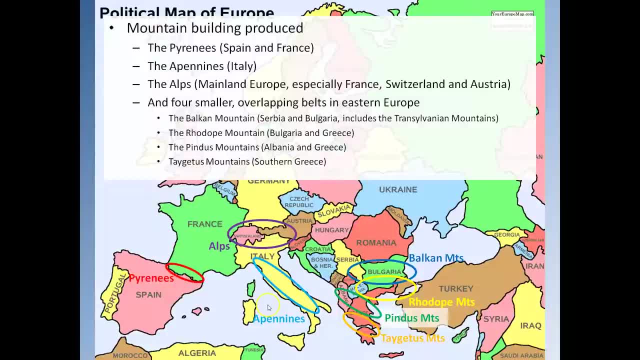 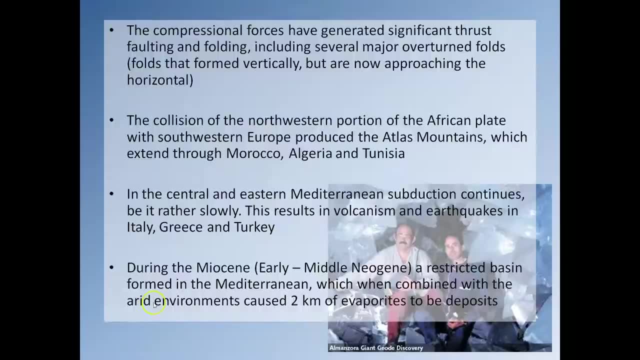 there's large-scale evaporation and it leads to the formation of very, very large sequences of evaporite minerals, and the thickness of the layer that forms is somewhere in the region of about two kilometres, and there's a picture back here of a couple of scientists. 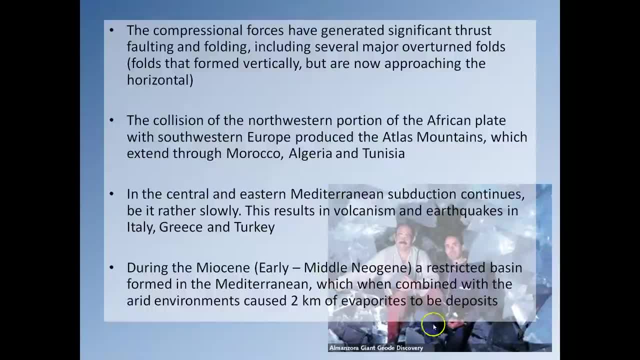 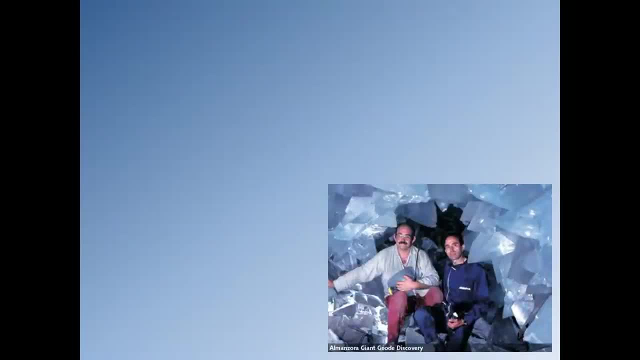 sitting within a huge geode which was formed by the evaporation of all this seawater and you can see these huge crystals of gypsum within the geode and that's been formed as part of this essentially evaporation event during the Miocene. 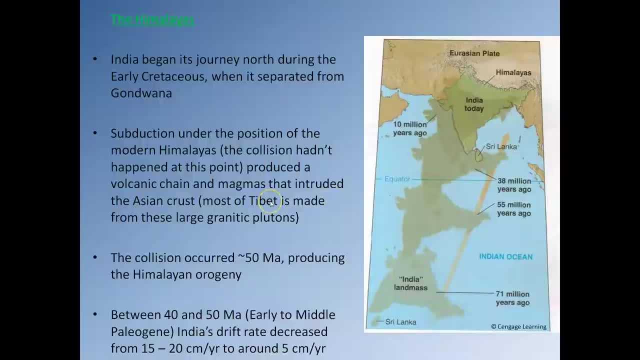 Alright, so we've been going for 20 minutes, so let's pause here. so get up, have a walk around, go and get a drink of water and come back in a couple of minutes, please. So the Himalayas. 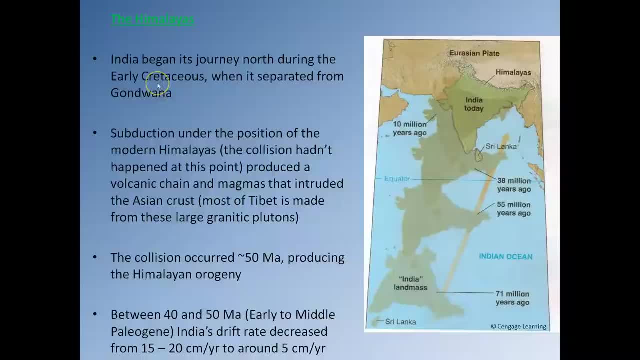 So India began its journey north during the early Cretaceous when it separated from Gondwana. So once India separated off and was its own little continental landmass, it began a northerly movement and that was the result of a subduction zone sitting along here. 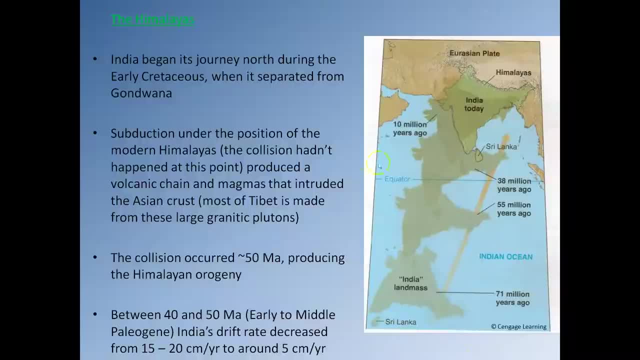 in now what is modern-day South Asia, and that was pulling the Teffian Ocean Crust, located down here to the south, in a northward direction, and it subducted underneath Asia and, of course, as part of that process, it pulled India in a northerly direction as well. 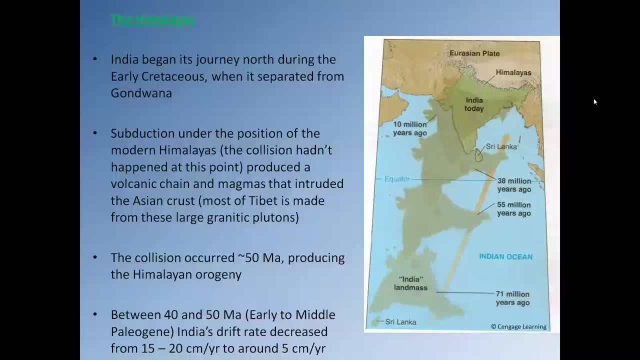 So subduction under the position of the modern-day Himalayas. so remember, at this point we're talking about 71 million years ago, so India's all the way down here, nowhere near Asia at this point. So, of course, what we do have, though, is we have the subduction. 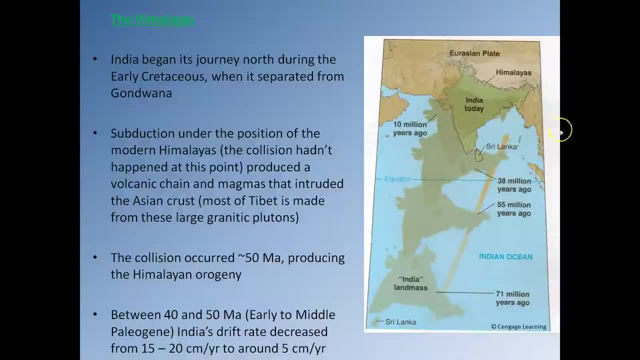 of the Oceanic Crust, the Teffis Ocean under Asia, and that's going to produce a mountain range somewhat similar to the Andes, And so you have an Andean-like mountain range running along the south coast of India and that, of course, that mountain range would be full of volcanoes. 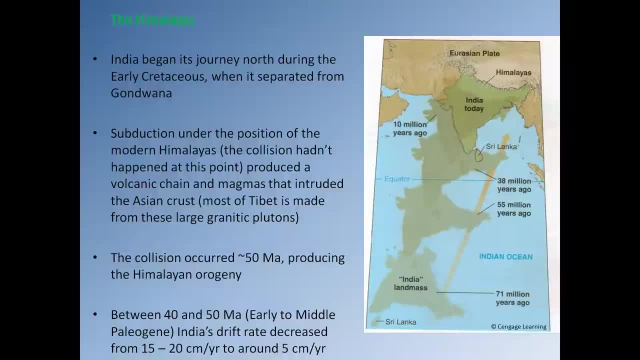 you would have had a volcanic chain associated with it and obviously you'd need large bodies of magma within the mountain range to feed those volcanoes, so there would have been huge intrusions as well within that mountain range as well, And of course, a good example of that is the country of Tibet. 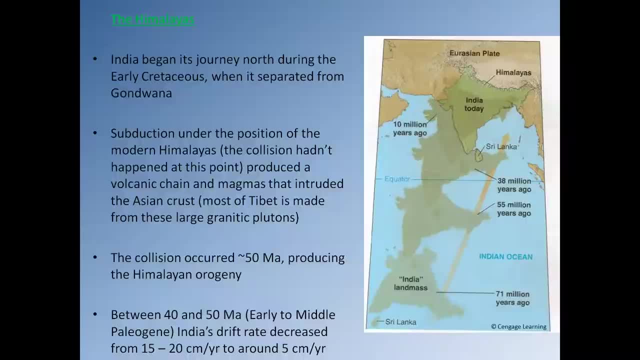 which is mostly made up of very, very large granitic plutons, which is mostly related to this stage of the subduction process or this stage of the northerly process of the movement of India. So in terms of the collision between India and Asia, 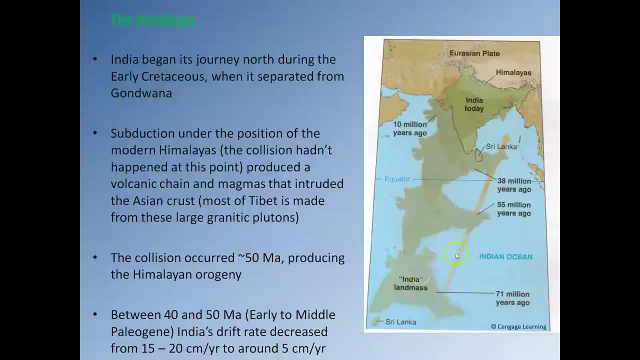 it began approximately 50 million years ago. Now, if you look at this diagram here, you're going to see that India 50 million years ago was actually somewhere around here. it's nowhere near the south coast of Asia. However, what you have to bear in mind is: 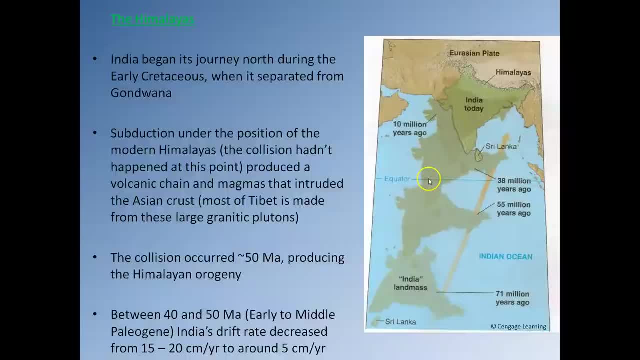 this is the modern shape of India. India 55 million years ago- or 50 million years ago if you take it a little bit- would have had a lot more continental crust along its northern margin and there would have been a whole pile of sedimentary rocks. 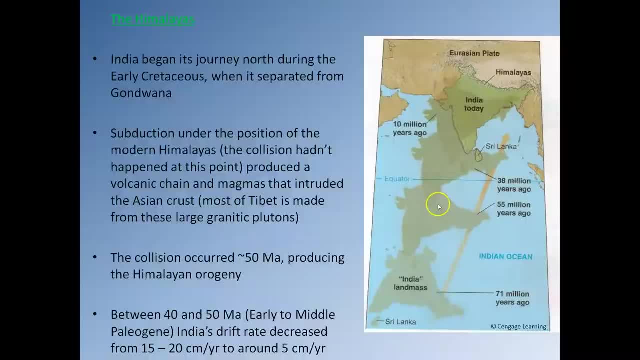 that were being scraped off as part of the subduction process, And that means this area here would have been a mess of sedimentary rocks, so marine sedimentary rocks and this continental crust here along the northern margin of Egypt. When I say Egypt, I mean India. 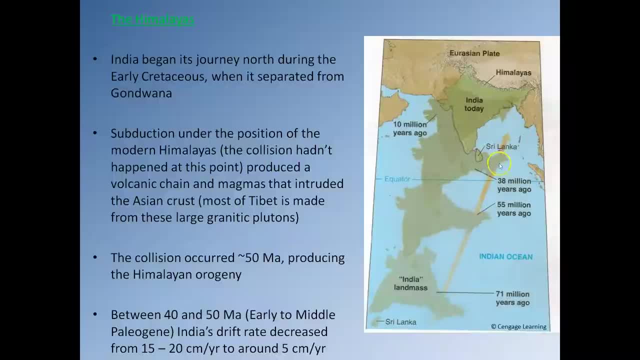 And so that would have meant that around 50 million years ago, we would have seen the first signs of the compressional forces associated with the northerly movement of India and its eventual collision with Asia, Even though modern day India, ie the country of India in its modern day shape, 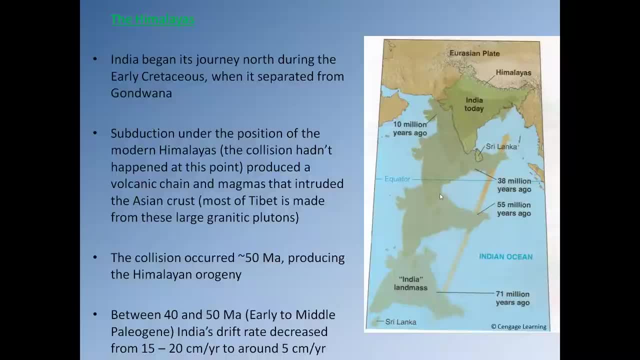 would have been all the way down here. So between about 40 and 50 million years ago, that's the early to middle Paleogene. India's drift rate decreases from about 15 to 20 centimetres per year to 5 centimetres per year. 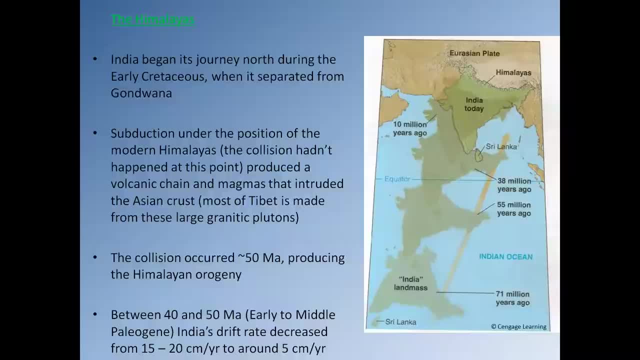 That's a very good indication that India is beginning to interact with Asia. So before that time, 50 million years ago, it was just the tephys oceanic crust subducting underneath Asia, and of course that's a rather straightforward process. 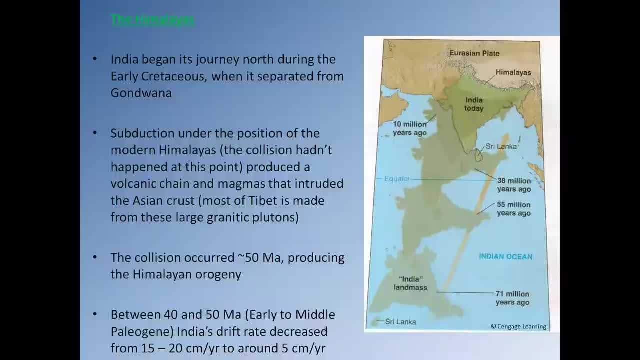 Oceanic crust like that is old and cold and heavy so it subducts underneath the light, warmer crust of the continent relatively easily, Around 40 to 50 million years ago. we see that rate of subduction slow down because now we have the buoyant. 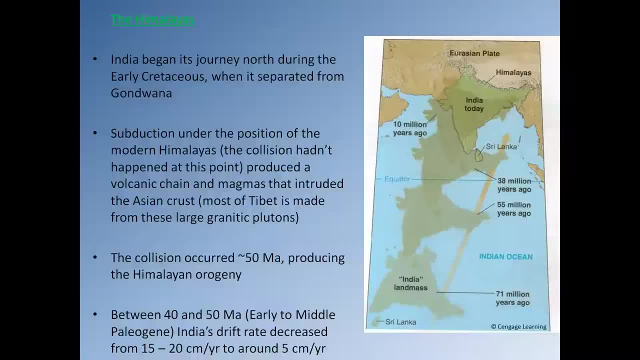 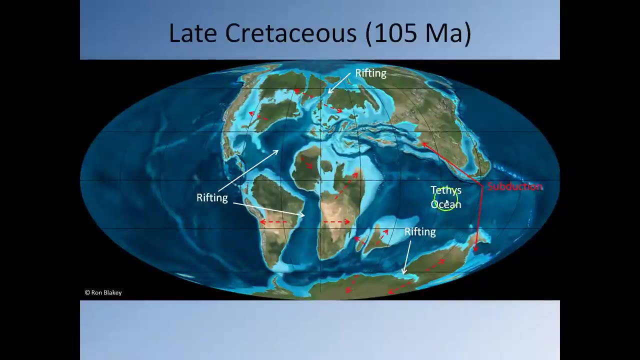 warm continental crust of India beginning to interact with the warm, buoyant continental crust of Asia, And so of course that makes subduction of the oceanic crust attached to India a lot more difficult. So this is our situation in the late Cretaceous. 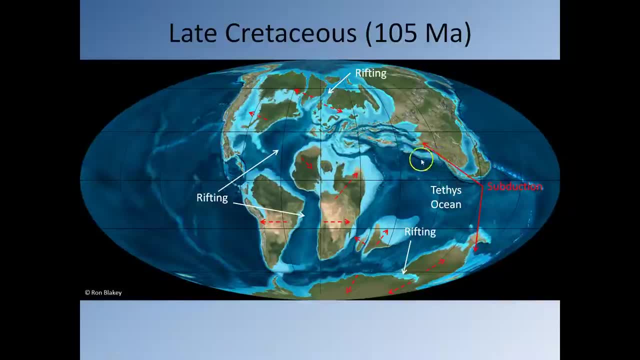 Here's the subduction zone, starting all the way over here in Southeast Asia, running up along the south coast of Asia and all the way along the south coast of now what is modern day Europe? And, of course, subduction of all of this oceanic crust here and here. 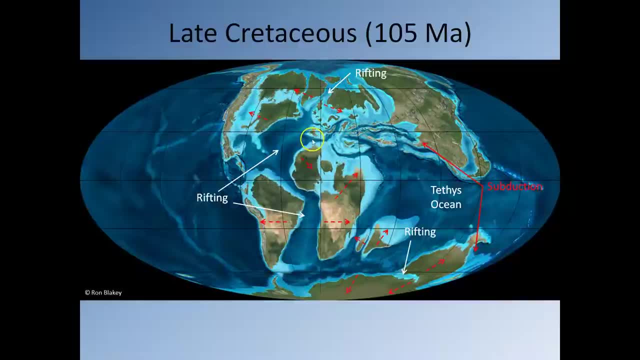 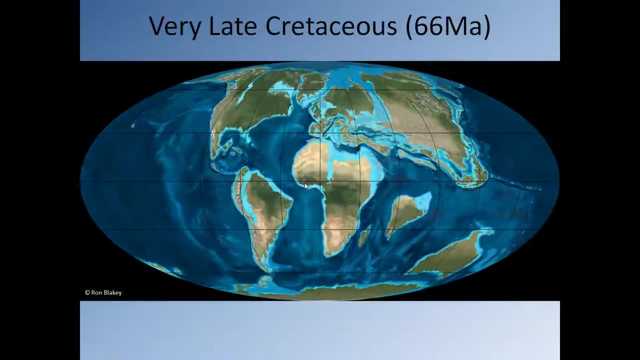 northwards, underneath Europe and Asia of course, pulls Africa northwards and India northwards as well. By the very late Cretaceous of course, we can see that we've had several small impacts here, A lot of these little pieces of continental crust. 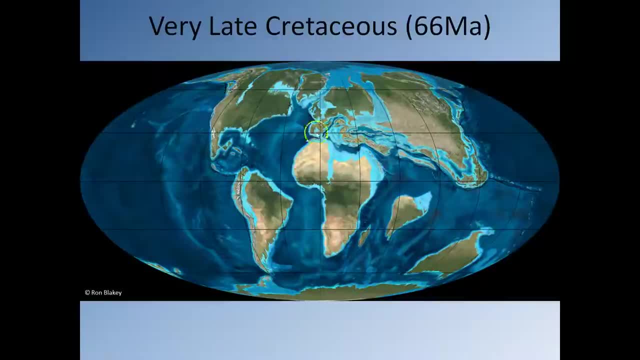 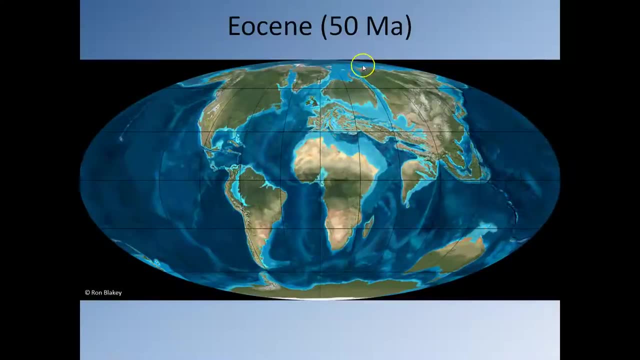 are beginning to accrete to each other to form what will become the main body of Europe. Africa's moving north India is now moving north By 50 million years ago. you can see the northern edge of India is beginning to interact with the south coast of Asia. 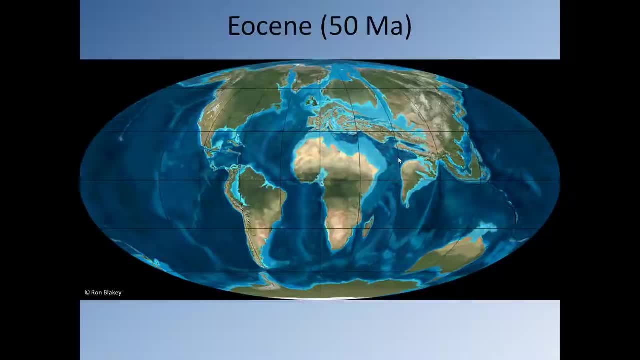 So this is where we start to see the early stages of the formation of the Himalayas and this is where we see the rate of drift, so the rate of northerly movement of India beginning to slow down because this continental crust here is interacting with the continental crust of Asia here. 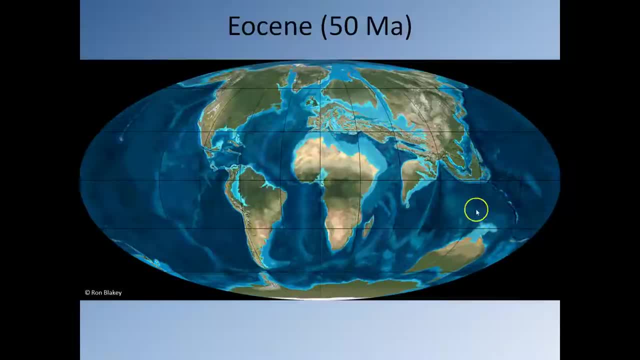 In terms of the other continents, you can see that Australia is getting relatively close to its normal position. Antarctica is exactly where it is now. South America and America and North America- they're drifting westwards and they're heading towards each other as well. 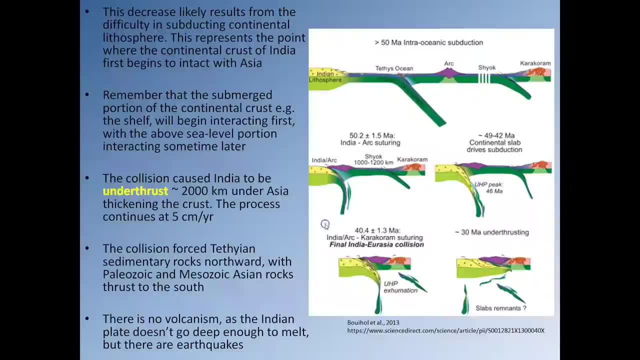 and pretty much everything looks about right. So, as I was mentioning, this decrease in the rate of subduction is the result of the difficulty of subducting the continental lithosphere, which is part of India. So if we look at the diagram here, 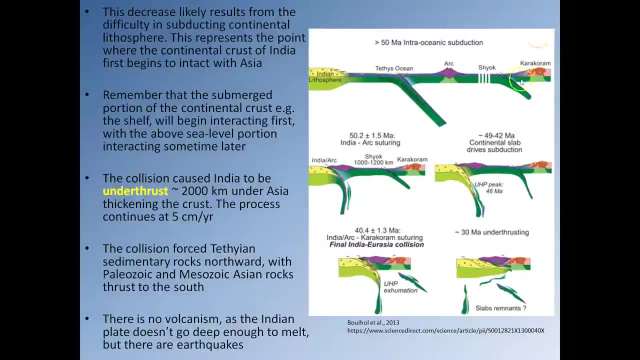 this diagram here summarises the Himalayan orogeny, So we can see initially Asia's over here and India is down here. This is essentially before 50 million years ago. So we have all this Teffian oceanic crust in between. 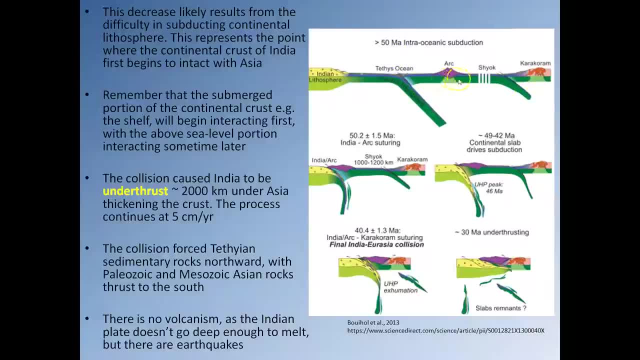 and we get the formation of a subduction zone underneath Asia here. So we have all this oceanic crust here subducting underneath Asia and there's also some evidence to suggest actually there was another subduction zone which formed a big island arc right between Asia and India. 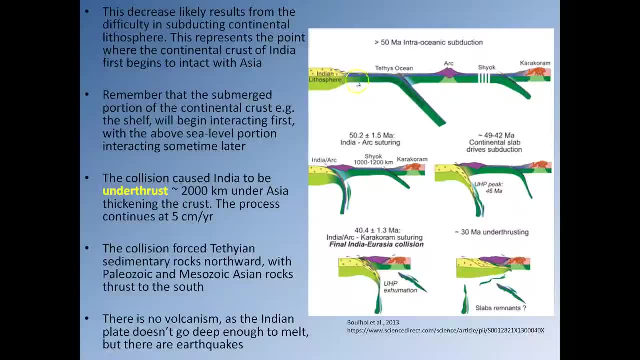 And so, over time, what happens is, India is obviously moving northwards due to this subduction zone. here, This island arc is also being pulled northwards towards Asia due to this subduction zone. here, However, this subduction zone is working more quickly. 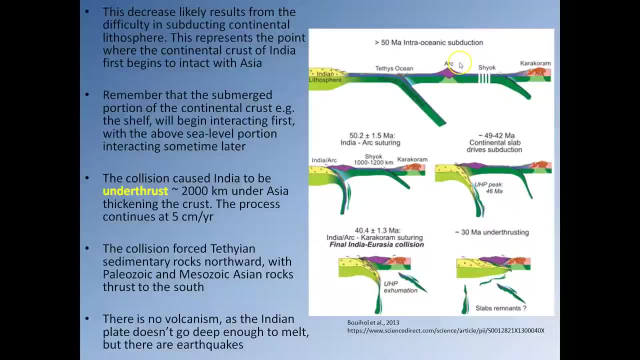 and eventually India crashes into this island arc here, So this subduction zone stops working. when that happens, Then this subduction zone becomes dominant, and so that means India and the island arc which is now attached to it steadily move northwards and they eventually crash into Asia. 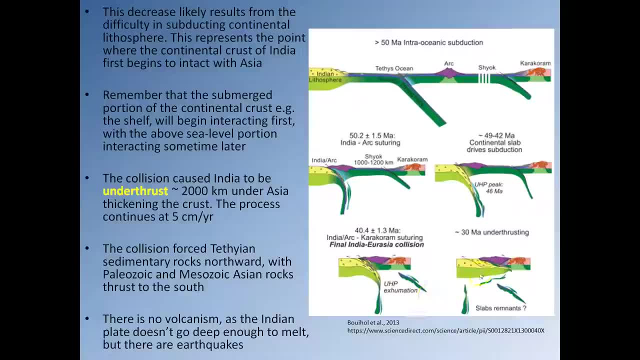 leading to the formation of the Himalayan mountains. It also leads to India being partially thrust underneath Asia, So this is called under-thrusting. So you can see this is the continental crust of India. here You can see, by the time the collision actually occurs. 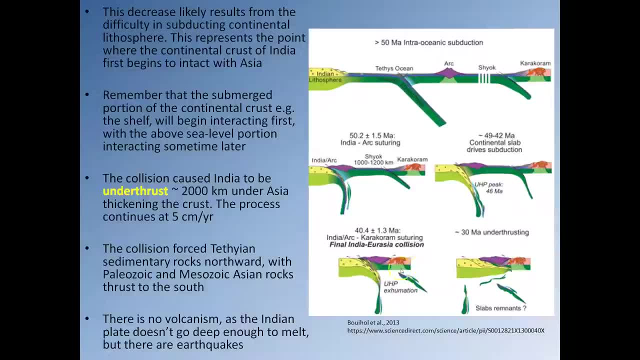 the continental crust of India actually gets pushed underneath the continental crust of Asia, And that's still happening now. So we need to remember that, in terms of the collision itself, this purple area here consists not only of this island arc, but it also consists of all of these oceanic sediments. 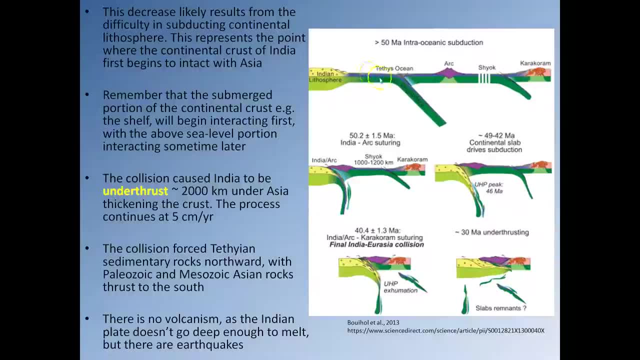 that were on the floor of the Teffis Ocean here, which were scraped off, and they all got mashed together to give us the modern-day Himalayan mountains, of course, along with the pieces of continental crust from India and Asia that were also added. 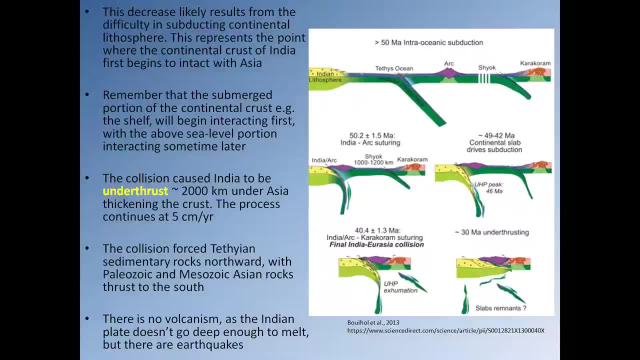 combined with that island arc and all those marine sediments to give us the modern-day Himalayas And a good example of exactly just how powerful that process was, if you ever decide to climb to the top of Mount Everest. when you get to the top, 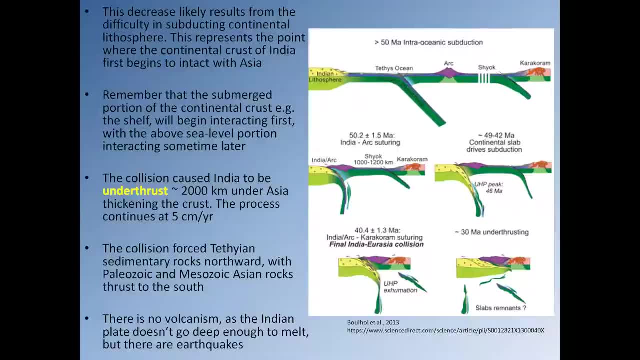 you will discover that at the top of Mount Everest there is actually a fossiliferous limestone. So, right at the top of Mount Everest, the rock you will come in contact with is a sedimentary rock which once upon a time formed on the sea floor of the Teffis Ocean. 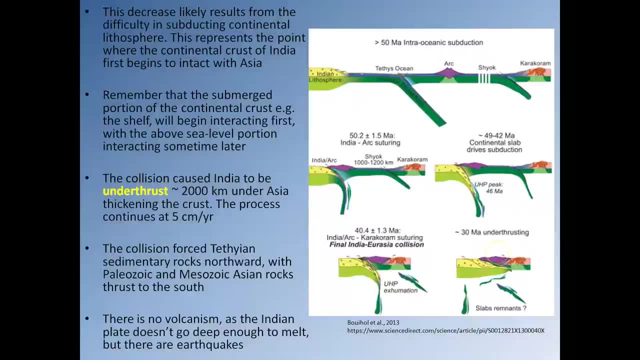 So that shows you just how high these rocks can be pushed. So, as I was saying, the collision itself caused India to be under-thrust underneath Asia by approximately 2,000 kilometres, So there's approximately 2,000 kilometres worth of Indian continental crust. 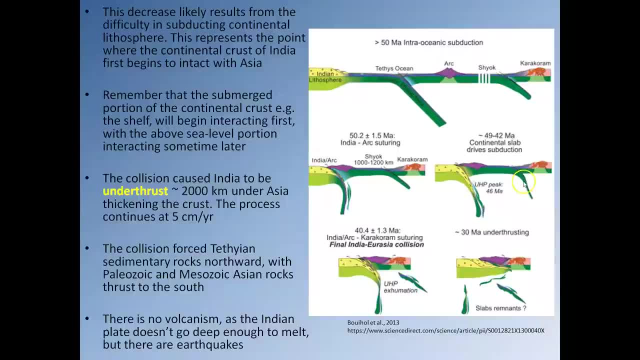 which has been pushed underneath Asia. So the collision forced Teffi and sedimentary rocks northwards and on the other side it pushed Paleozoic and Mesozoic Asian rocks southwards. And, of course, the collision of these two sets of thrusts. 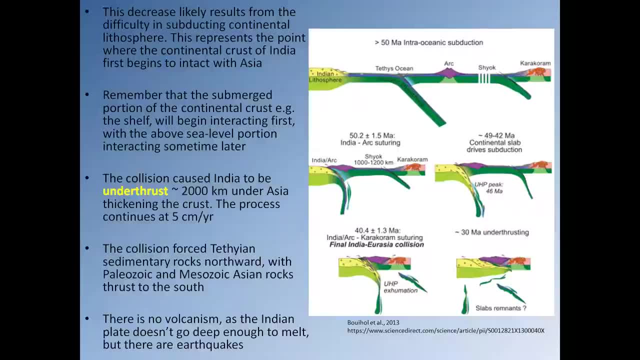 running in opposite directions leads to big sheets of rock piling up one on top of another, and of course, that gives us a huge mountain range which we see as the Himalayas. Now, once the subduction stops, of course, there is no material diving down into the mantle. 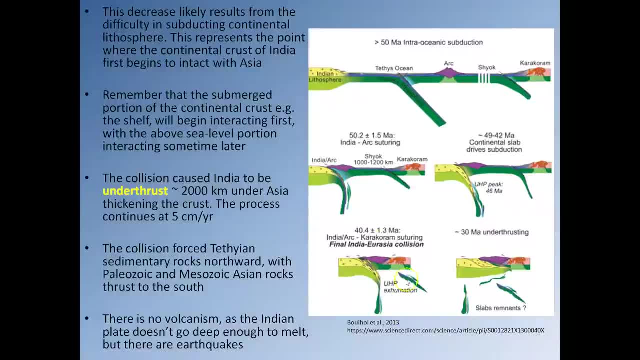 so that means there's no more melting, And so that means once this collision occurs, it means volcanism very quickly begins to stop because there's no new magma being created. And so obviously that stops volcanism Now because of course, 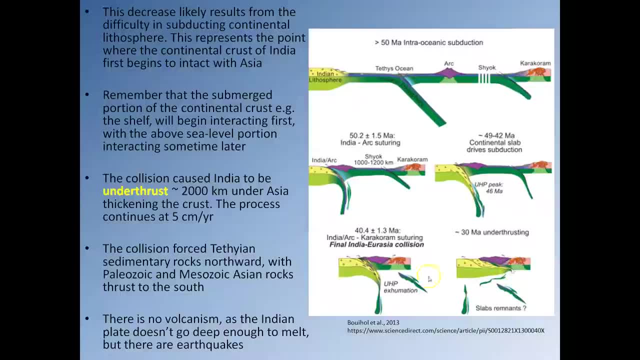 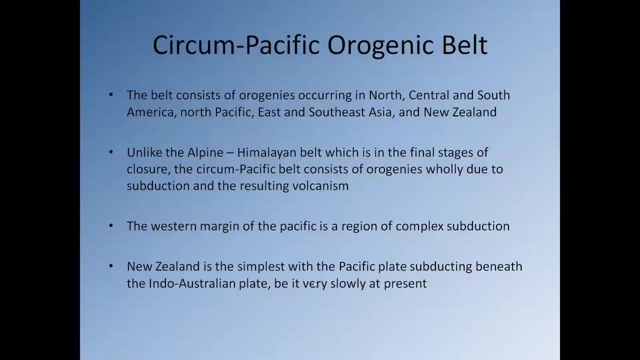 we do have these two large pieces of crust still banging into each other. it does, however, mean this area is extremely prone to earthquakes. OK, so what about the Circumpacific Orogenic Belt? Well, the belt consists of orogenies occurring. 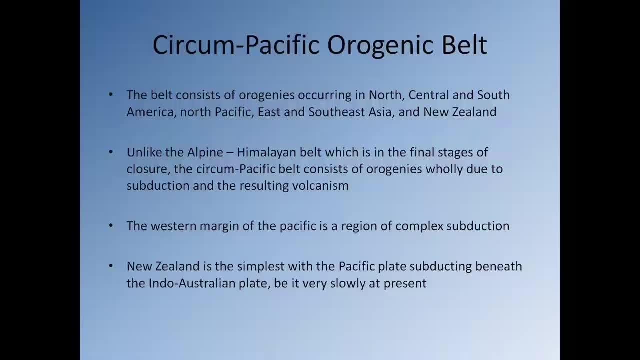 in North, Central and South America, the North Pacific, East and Southeast Asia and New Zealand. So, unlike the Alpine and Himalayan Belt, which is the final stage of closure, the Circumpacific Belt consists of orogenies wholly due to subduction and the resulting volcanism. 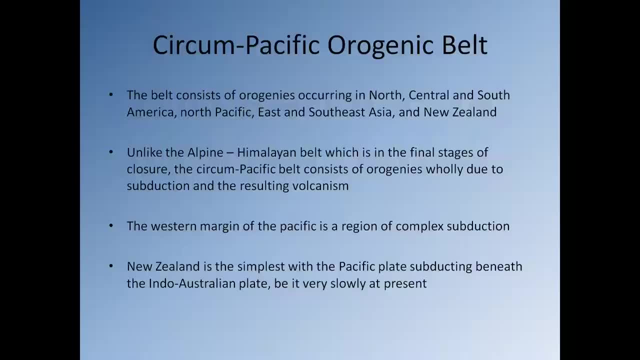 So the western margin of the Pacific is a region of complex subduction with. So yeah, New Zealand is the simplest, with the Pacific Plate subducting beneath the Indo-Australian Plate, be it very slowly. So in terms of you know, New Zealand, 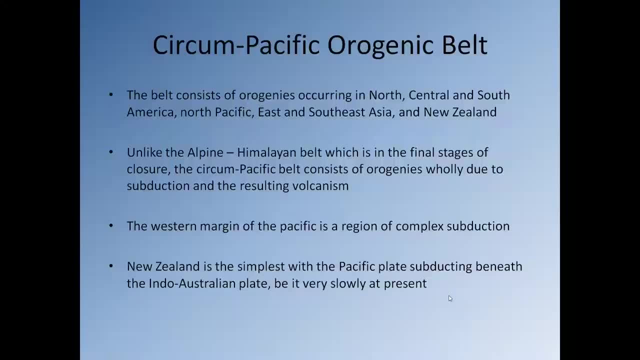 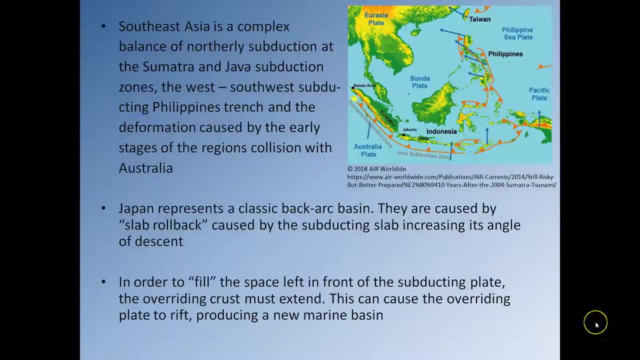 it's a relatively straightforward subduction zone. You have an ocean-ocean subduction zone there. nothing particularly special going on Now in Southeast Asia, as you can see from this diagram, here the situation is considerably more complicated. So we have northerly subduction along this trench here. 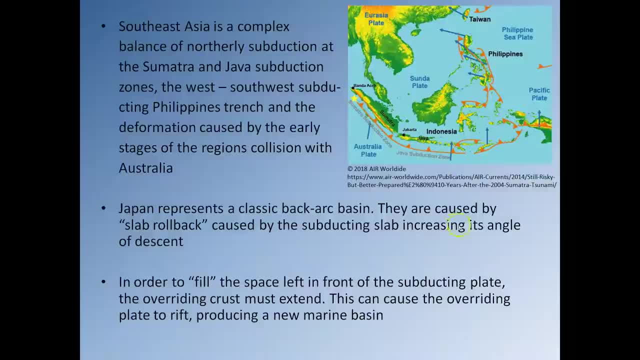 so this is the Sumatran subduction zone, Java subduction zone. So that's taken oceanic crust here from the Indian Ocean and it's subducting it approximately northeastwards underneath Southeast Asia. We also have a subduction zone running along here. 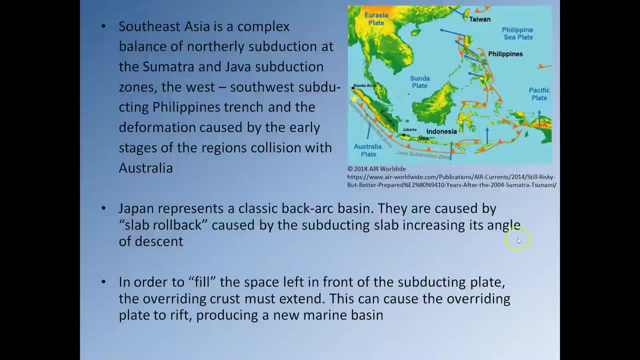 and that's taking crust between Australia and Papua New Guinea and it's subducting that northwards. At the same time, we have the Pacific Plate over here, or more accurately, the Philippines Plate over here, which is subducting westwards underneath Southeast Asia as well. 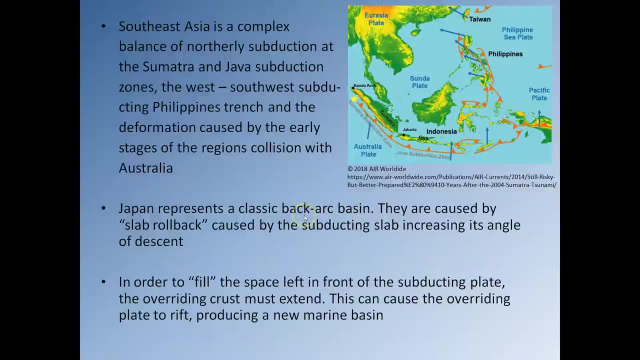 So we have oceanic crust coming from the southwest running northeast, We have subduction coming from the south going north and we have subduction coming from the south, coming from the east going west. So you can see, we have lots of oceanic crust. 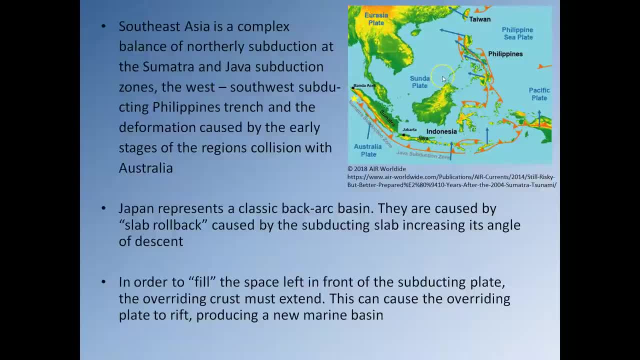 all converging in this area here and this leads to a very complex tectonic situation in Southeast Asia. So it leads to lots and lots of volcanism and an area that is extremely prone to earthquakes. In terms of what's going on further up here. 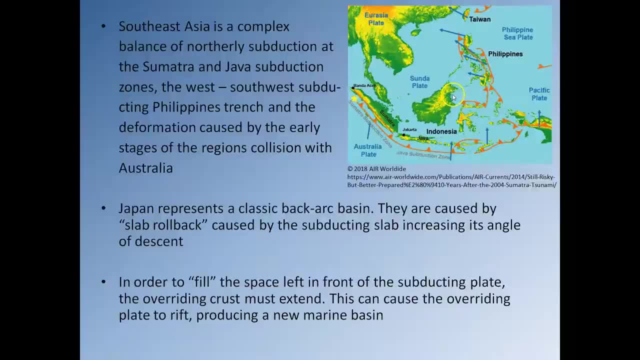 we come to Japan, and Japan represents a classic back-up basin situation, And the back-up basin that forms Japan is the result of what's referred to as slab rollback, And this is caused by the subducting slab, the Pacific Plate, which is subducting underneath Asia. 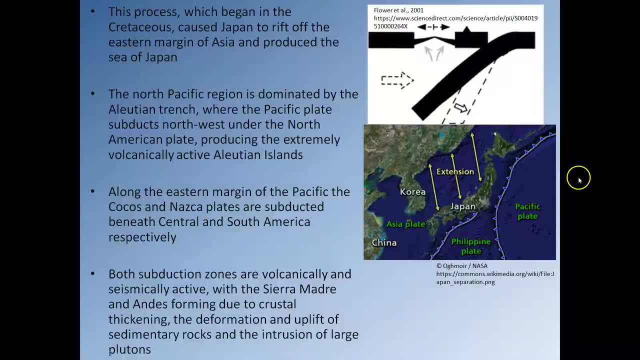 increasing its angle of descent. So if we jump to the next slide for a second, you can see what's going on. So once upon a time, this chunk of crust here would have been joined to this chunk of crust here, So Japan would have been connected. 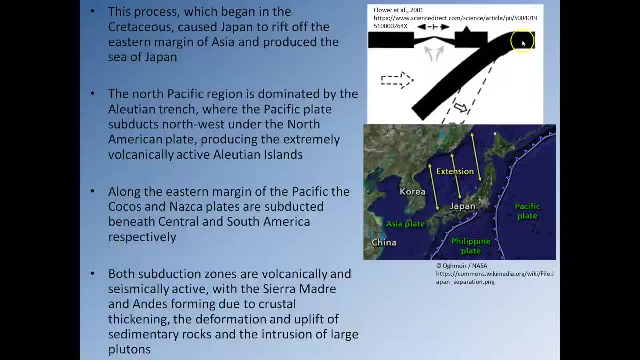 to Asia. Now what's happened is we've got a subduction zone that runs along the Japanese coast here, and so we have the Pacific Plate subducting underneath Japan. Now what's happened is the Pacific Plate initially started to subduct at a relatively shallow angle. 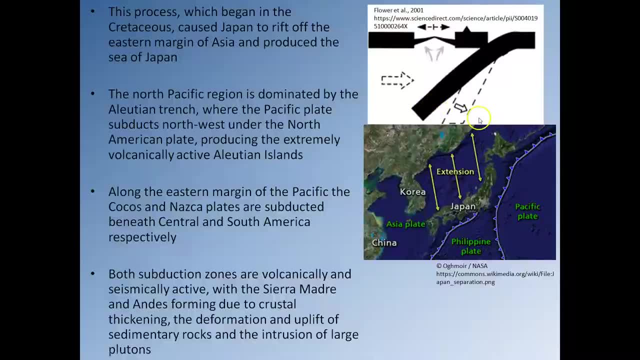 and over time the angular subduction has become steeper. So as the angular subduction has steepened and the Pacific Plate has moved in this direction, it's meant that a region just in front of the Pacific Plate, it means that a region in front of 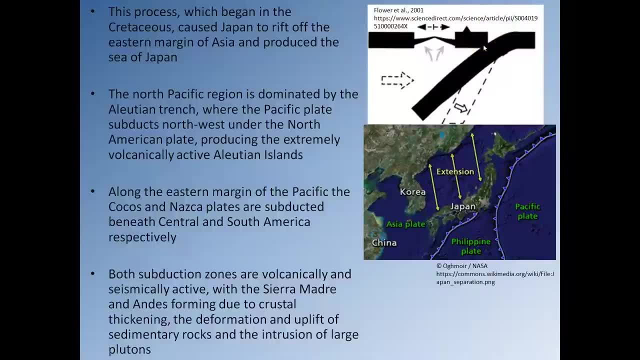 or between the two plates here essentially becomes a void. There's empty space there. So as the Pacific Plate begins to subduct at a steeper angle, it means a void opens up here at the front, And obviously you can't have that. 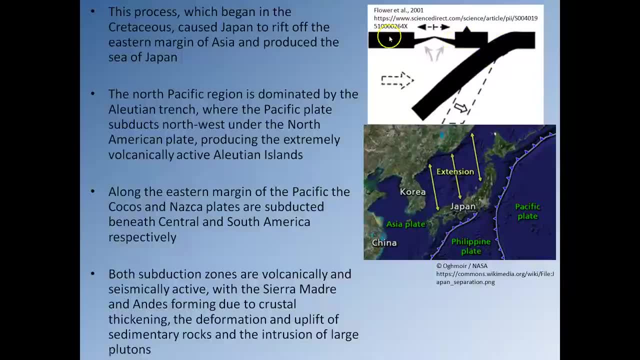 The void has to be filled, and so that has to be filled by the continental crust of Asia stretching to fill the empty space, And of course this results in the formation of extensional tectonics, And this led to Japan rifting off. 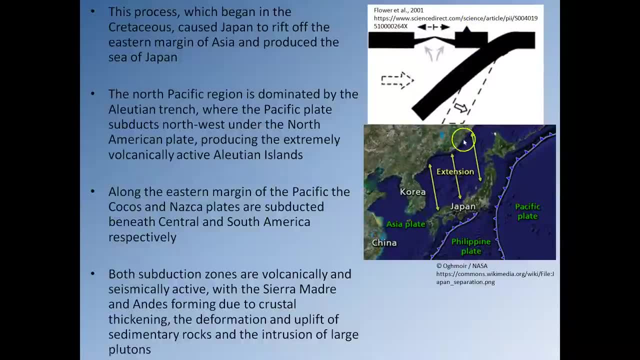 this island. here is Japan, rifting off the side of Asia and eventually it got to the point where the crust between Asia and Japan became so thin that a spreading ridge opened up and it started creating new oceanic crust here and that produces the seafloor. 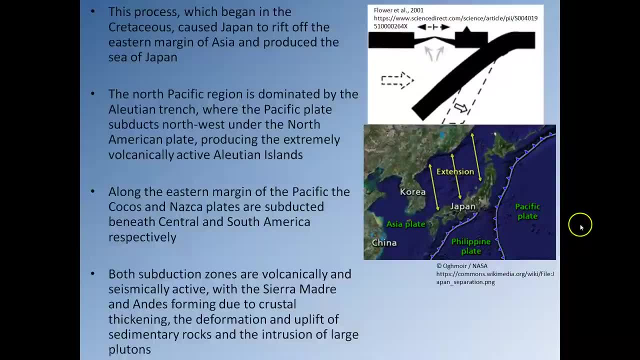 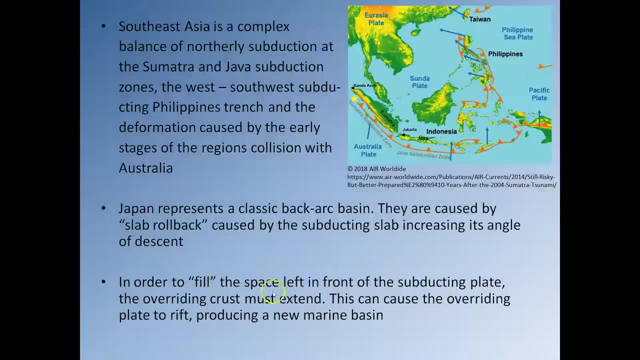 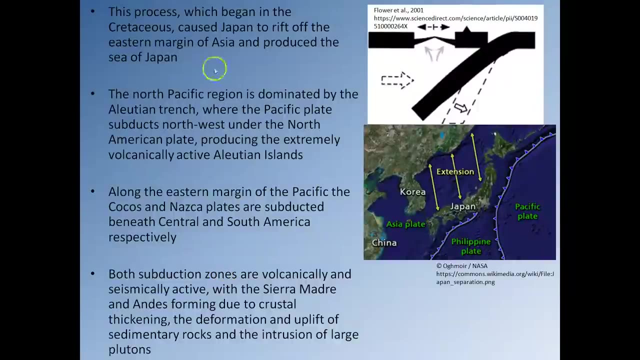 which we see as part of the Sea of Japan. So, as I say, in order to fill the space that's produced by the slab rolling back, Asia had to extend itself to fill the empty space that was being created. So this process began in the Late Cretaceous. 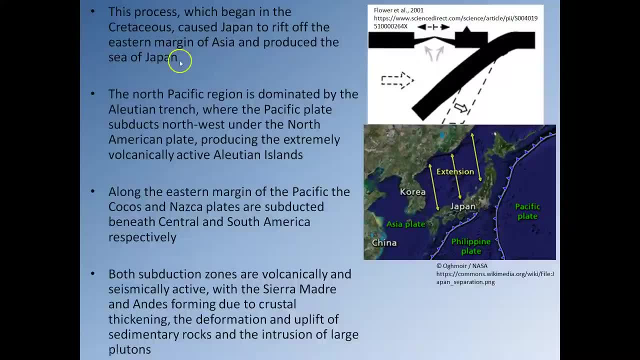 and it caused Japan to rift off the eastern margin of Asia and produce the Sea of Japan. The North Pacific region is dominate, so that was what's going on in Western Asia In terms of the North Pacific. that region is dominated by the Aleutian Trench. 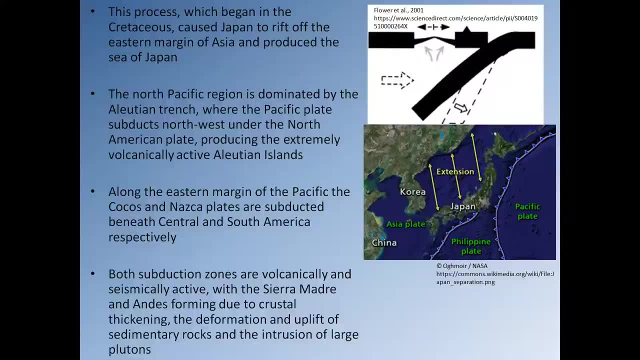 where we have the Pacific plate subducting northwestwards under the North American plate and of course that leads to the formation of the extremely volcanically active Aleutian Islands. So along the eastern margin of the Pacific we have the Cocos and Nazca plates. 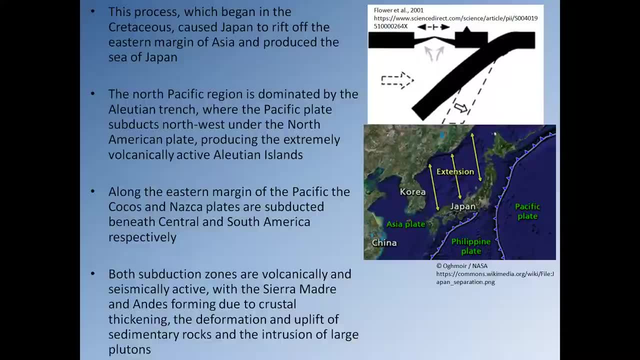 which are subducting beneath Central and South America respectively, and of course that leads to the formation of the Andes and the formation of several smaller mountain ranges through Central America. Both of these subduction zones are very volcanically and seismically active. 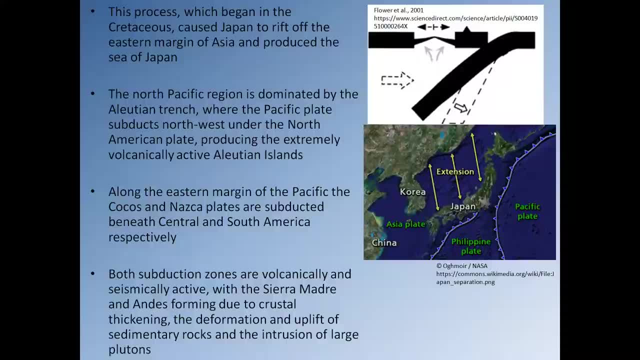 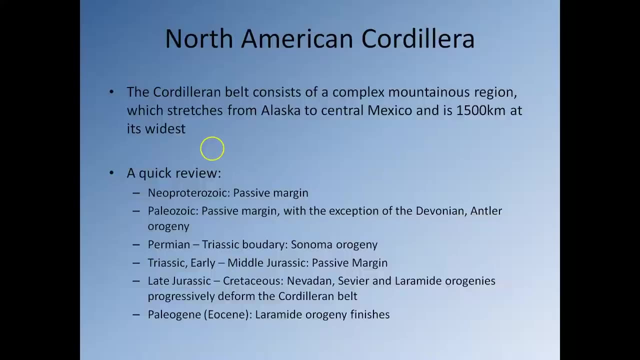 with the Sierra Madre and Andes forming due to the crustal thickening and deformation and uplift associated with the collision. Okay, that leaves North America. So what was going on with North America? So the Cordilleran Belt consists of a complex mountainous region. 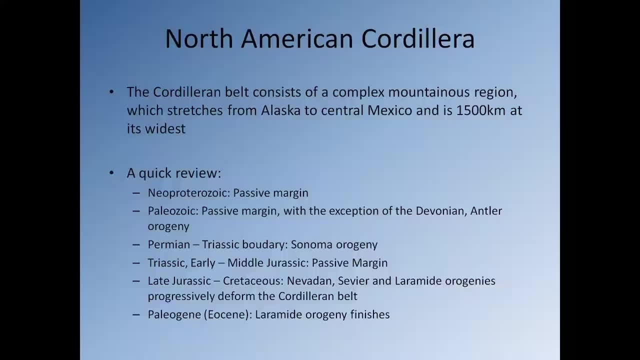 and it stretches from Alaska all the way down to central Mexico. So it's approximately 1,500 kilometres at its widest. So it's very, very long and it's a pretty broad mountain range. Now we discussed earlier why it was relatively broad. 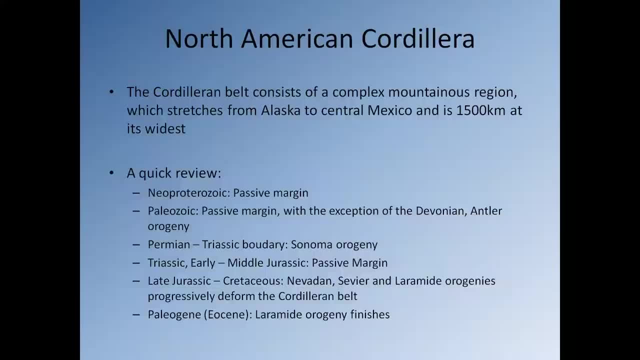 We discussed that because the angular subduction of the Farallon Plate changed over time. it meant that the tectonic forces were steadily dissipated over a larger and larger region of the western North America and this led to the Rockies becoming wider and wider and wider. 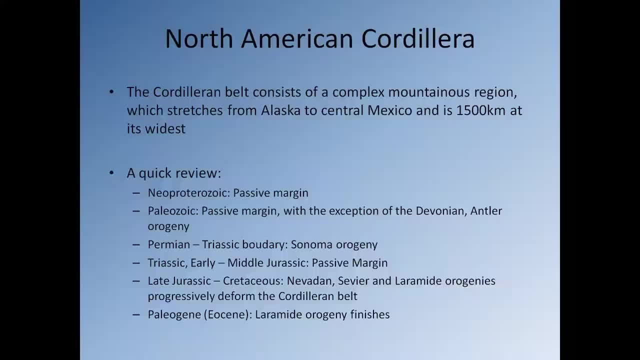 So for comparison, your normal ocean continent subduction zone should have a relatively tight mountain range, a little bit like the Andes. So the fact that the Rockies is so broad is a reflection of the fact that tectonism didn't quite go. 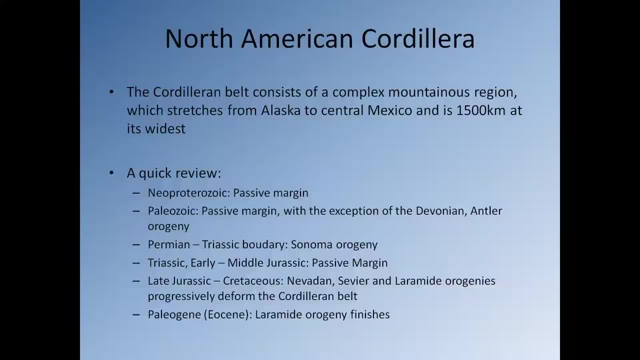 well, didn't quite follow the normal plan along the west coast of North America. So in terms of the west coast of North America, let's do a quick review. So during the Neoproterozoic the margin was passive. 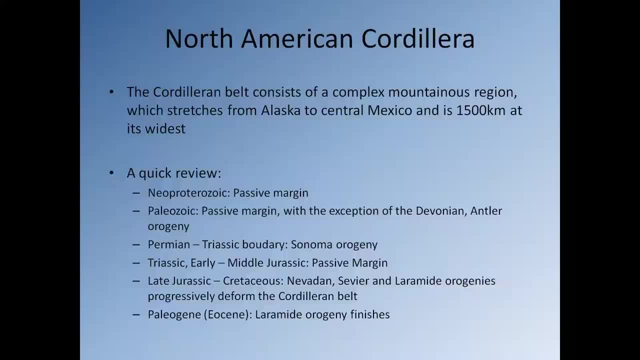 During the Paleozoic. once again it was mostly a passive margin, with the exception of the Devonian Antler Orogeny Between the Permian and the Triassic. we had the relatively small Sonoma Orogeny From the Triassic into the Early and Middle Jurassic. 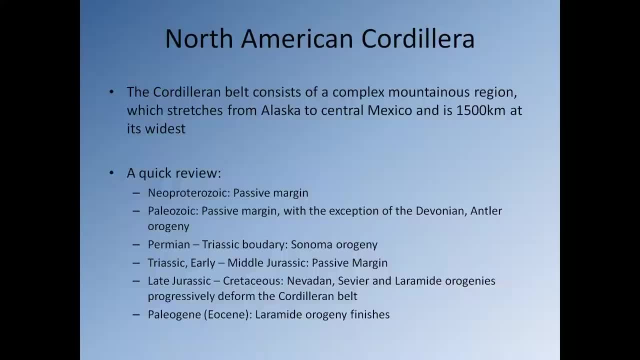 it was a passive margin again From the Late Jurassic to the Cretaceous. we had the Nevadian, Sevier and Laramide Orogenies And that progressively deformed the Cordillerian Belt, producing the modern-day Rockies. 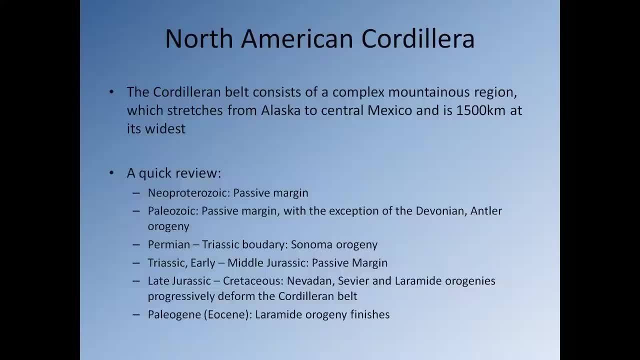 And by the time we make it into the Paleogene, so that's the Eocene, the Laramide Orogeny comes to a stop, So it finishes approximately, you know, 45 million years ago. give or take a little bit. 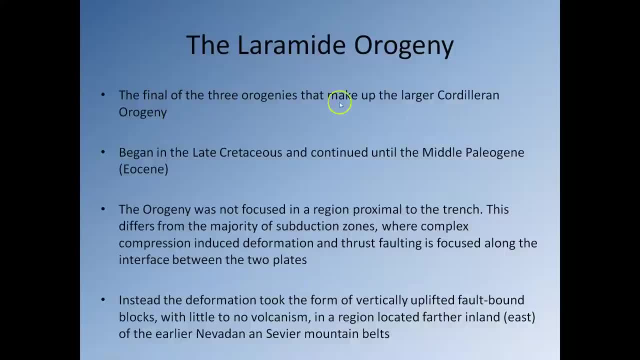 So in terms of the Laramide Orogeny, it's the final of the three orogenies that make up the Cordillerian Orogeny. So it began in the Late Cretaceous and it continued until the Middle Paleogene. 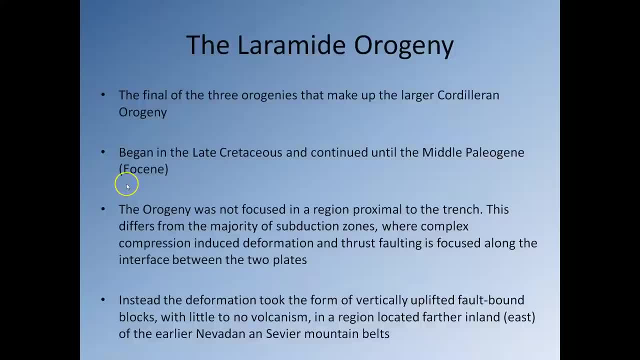 as I said, the Eocene, So the orogeny, was not focused in a region proximal to the trench like most subduction zones. So you know, most of the time the volcanoes, the mountain ranges located relatively close to the trench. 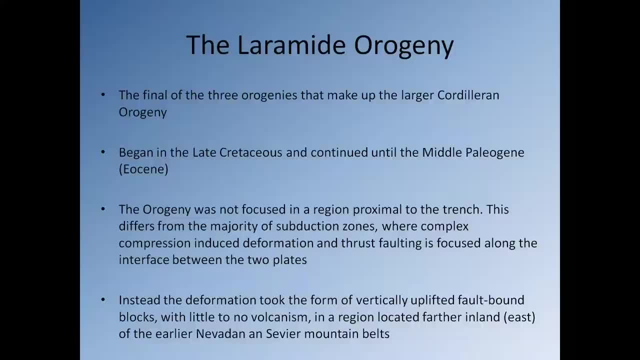 In the case of the Laramide Orogeny. the deformation associated with the Laramide Orogeny occurred a long way back from the trench, So it's relatively deep into continental North America. So it should in theory. 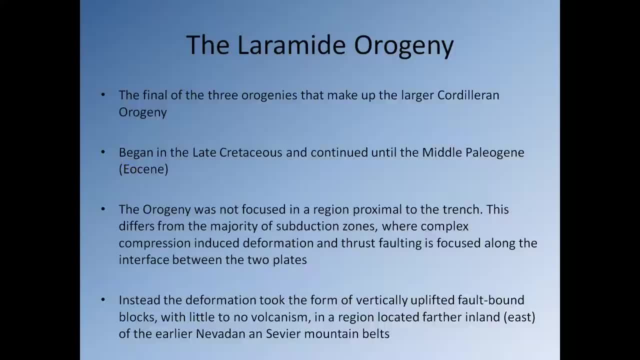 the deformation in the volcanism should have been located along the modern-day west coast of North America. In reality, for the Laramide Orogeny, most of the deformation was in fact well inland, which is a bit abnormal. So what we see is, instead of deformation. 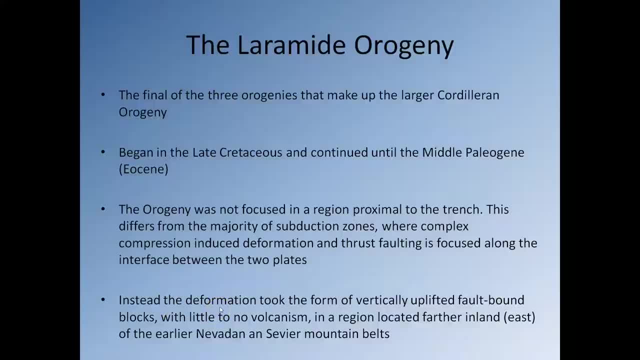 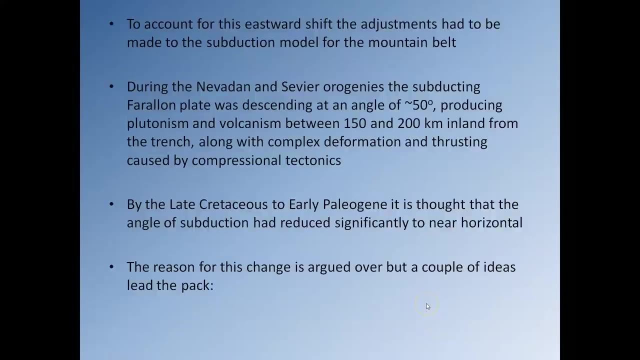 instead of the standard deformation you know that we would expect, what we get is a lot of vertically uplifted fault-bound blocks, little to no volcanism in a region that's located further inland than the Nevadian and the Sevier mountain belts. 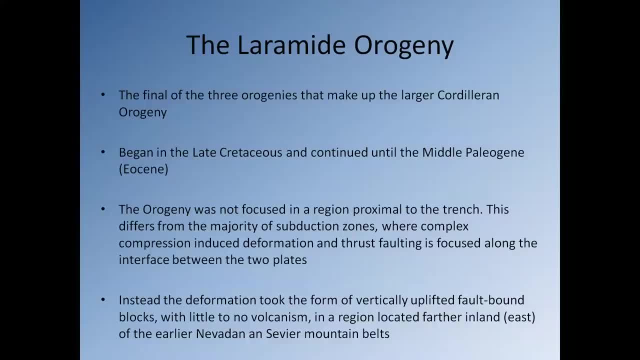 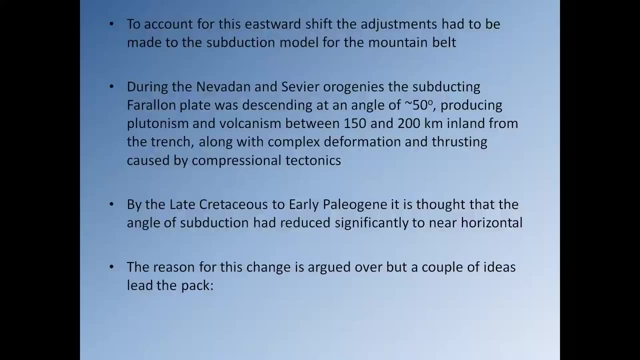 So that's a bit of a problem. Why do we have this shift of the Cordillera Orogeny steadily in an eastly direction, deeper and deeper into continental North America? So to account for this eastward shift, the adjustments had to be made. 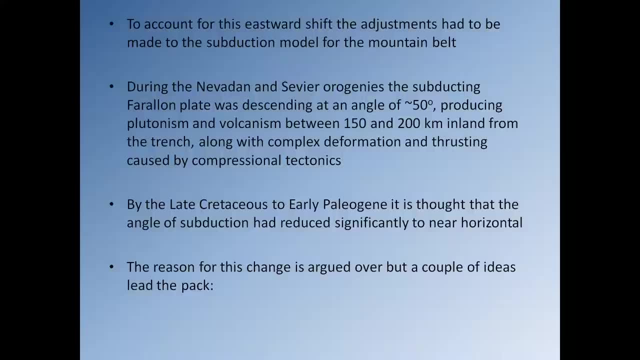 to the subduction model for the formation of the Cordillera Mountains. So during the Nevadian and Sevier orogenies the subducting farallon plate was descending somewhere around 50 degrees, give or take a bit. Now we know the angular subduction was steadily shallowing. 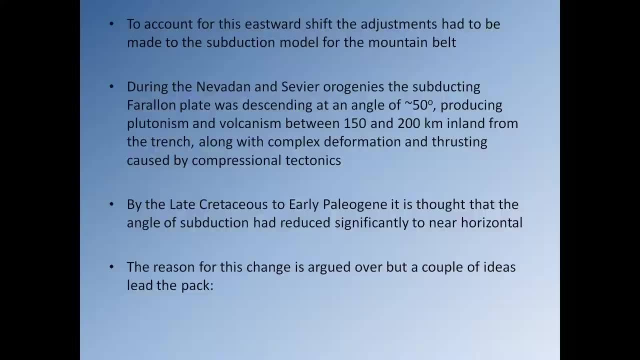 as you went from the Nevadian to the Sevier orogenies, but it was still relatively steep And this meant that the subducting oceanic crust would plunge down into the mantle. it would make it to the magic 150 kilometer depth. 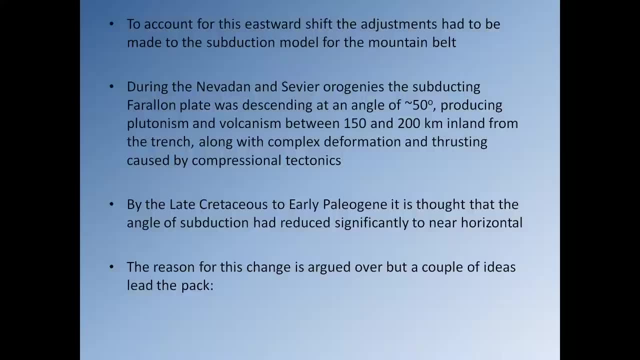 at which point it would start melting, producing magma that would move towards the surface, feeding volcanoes within the mountain range, And these volcanoes were located about 150 to 200 kilometers inland from the trench, pretty much where you would expect them to be. 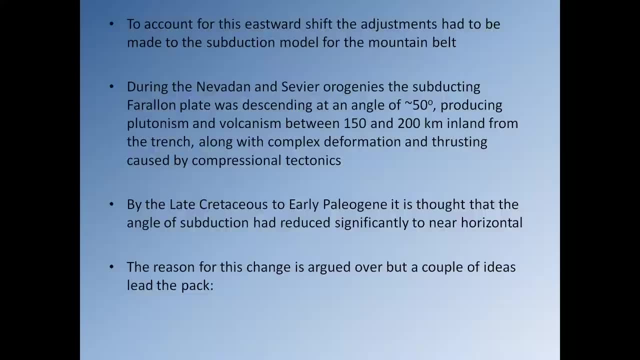 for a normal ocean-continent subduction zone. Obviously, along with the volcanism, there was a lot of very complex deformation and thrusting caused by the very, very strong compressional tectonics. once again, just like the modern-day Andes. 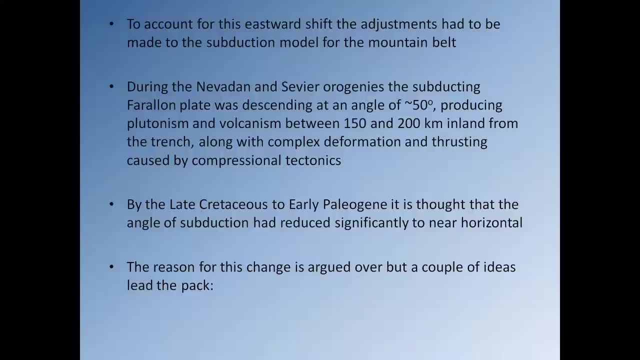 So by the late Cretaceous to early Paleogene it's thought that the angle of subduction, so that's the Farallon Plate, had reduced significantly to near horizontal. And so this means that you know, by the time we're into the late Cretaceous and early Paleogene, 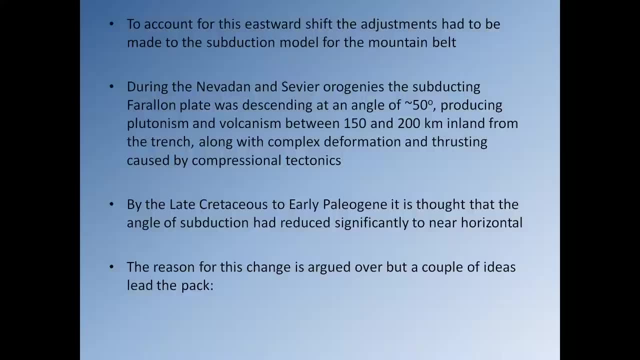 the Farallon Plate is literally grinding along the bottom of North America, so it's not really subducting properly. So that's a bit strange. So we need to come up with an explanation to explain why this piece of oceanic crust that should be diving down into the mantle quite easily. 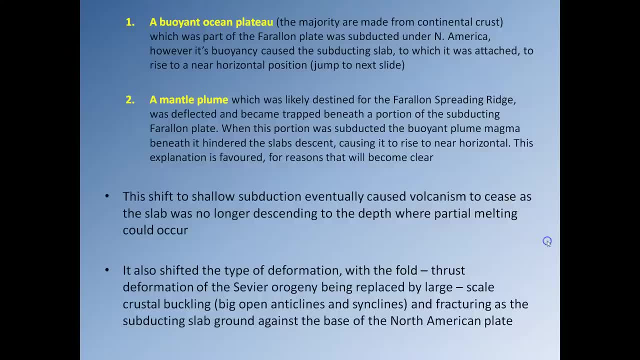 is not subducting well at all, And you know what. We'll discuss that after you guys have had a break. So let's pause the presentation here, get up, have a walk around, go and get a glass of water and please come back in a few minutes. 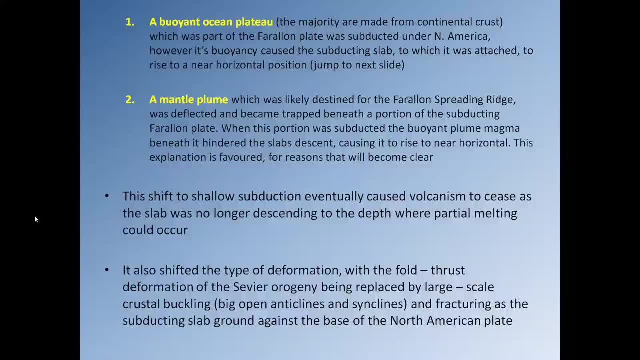 So OK. so why could the Farallon Plate not subduct well? Well, there's a couple of possible reasons. The first one is a buoyant ocean plateau. So the majority of buoyant ocean plateaus have a proportion of continental crust in them. 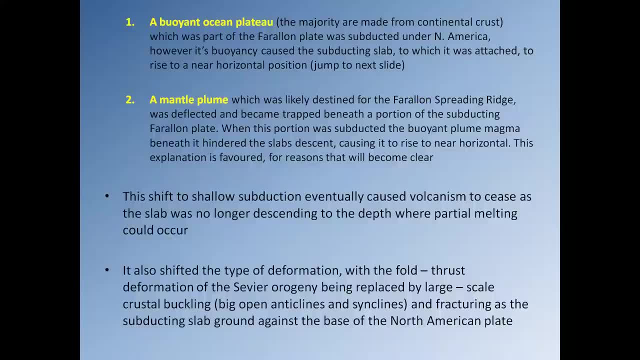 So what is an ocean plateau? Well, it's a flat raised area of the sea floor. So essentially, it's a plateau on the ocean floor, And some of them can be extremely large And, as I said, most of them will have a proportion. 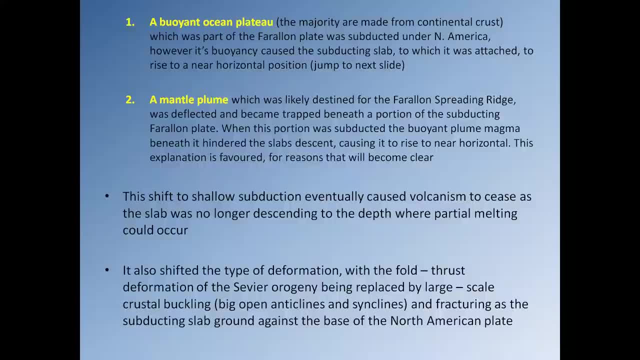 of continental crust mixed in with the ocean plateau, And so this means that when you try and subduct an ocean plateau, well, the continental crust mixed in with it makes it far more buoyant than normal oceanic crust, And so that means if you try and subduct it, 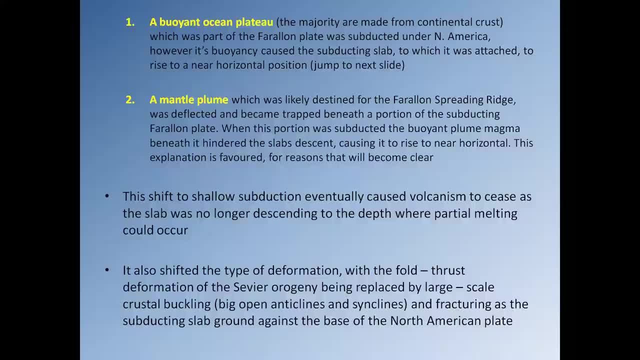 well, it's not going to subduct easily at all. So as the oceanic crust tries to dive down into the mantle- because you know it's old, cold oceanic crust so it wants to go down- it's fighting against this continental crust attached to the top of it. 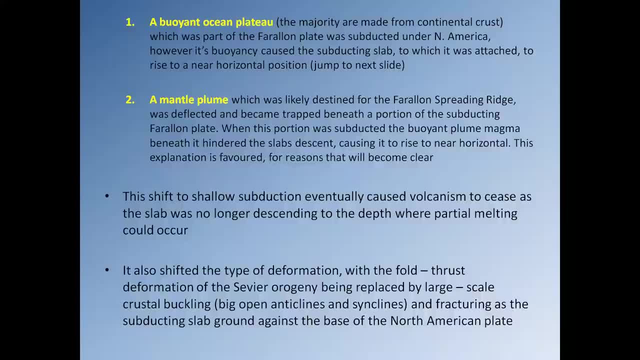 that wants to go up because it's warm and buoyant, And so what happens is the continental crust wins and it starts decreasing the angle of subduction until, eventually, the farallon plate is subducting horizontally and grinding along the bottom of North America. 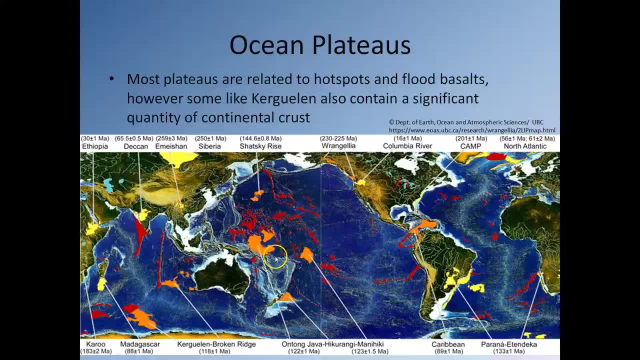 So just to jump to the next slide here, in this slide you can see the position of the oceanic plateau, So you can see them marked out here. They're here in red and orange, So you can see some of these plateaus are absolutely huge. 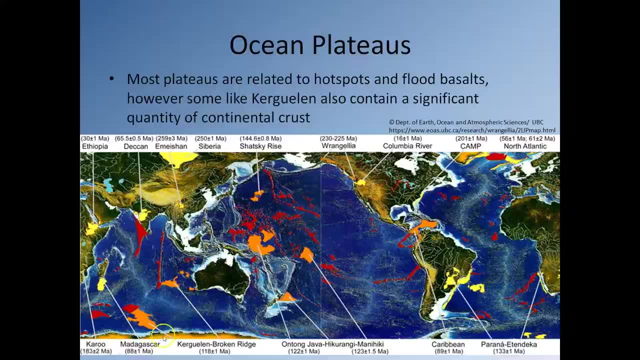 I mean, you've got the Ontong Java over here. You have now do excuse my absolutely horrendous pronunciation, but you've got the Kerguelen broken ridge plateau over here. Now this is mostly made up of, you know, flood basalts. 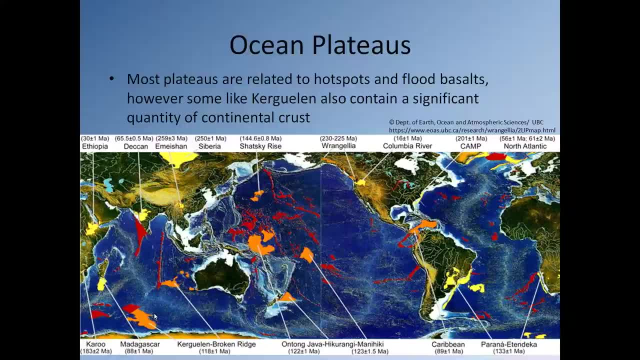 However, mixed in with it there are big chunks of continental crust. So if you try and subduct this mass here, well, it's not going to subduct very easily at all, And so that's the situation that has been envisaged. 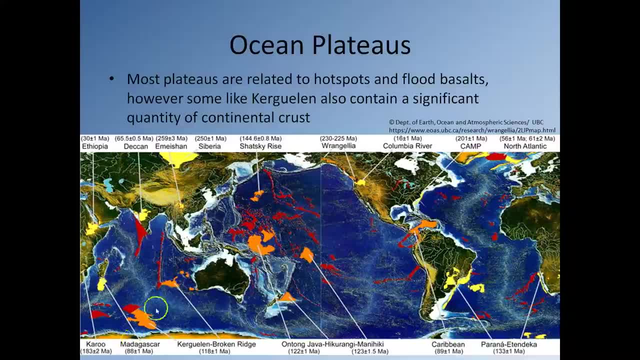 for the farallon plate. So let's say, the farallon plate had something the size of this attached to it As it was subducted underneath North America. well, naturally it's going to cause the subducting farallon plate to begin to rise up and cause the angle of subduction to shallow. 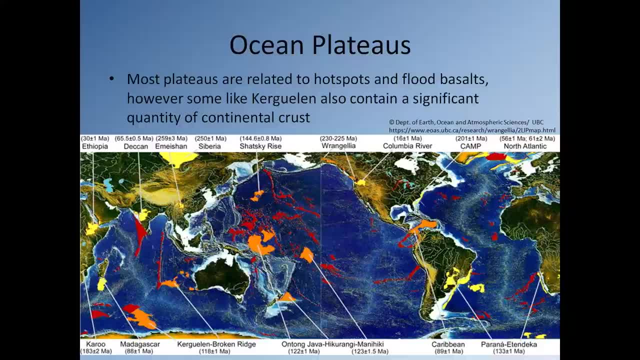 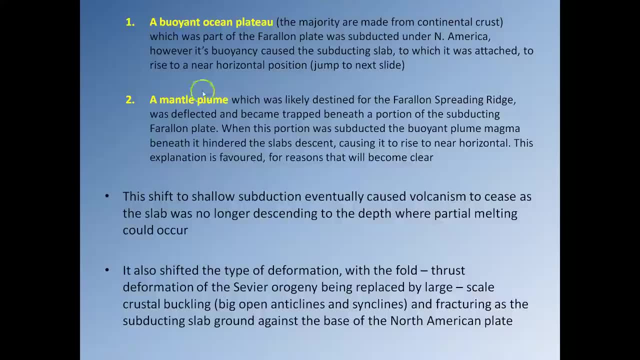 until eventually the farallon plate is subducting almost horizontally. So that's the first possible explanation. The other possible explanation is a mantle plume. So if you remember, a mantle plume is when you get a big ball of magma that forms at the core mantle boundary. 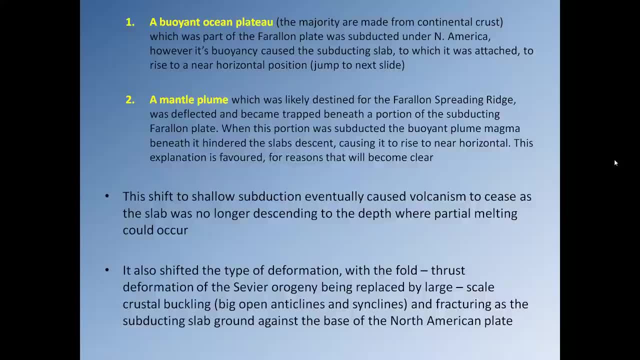 It comes hurtling up through the mantle because it's so amazingly buoyant, And typically they get stuck at the base of the continental or oceanic lithosphere. Now the one thing that you're trying to do is, if you then have a piece of oceanic crust, 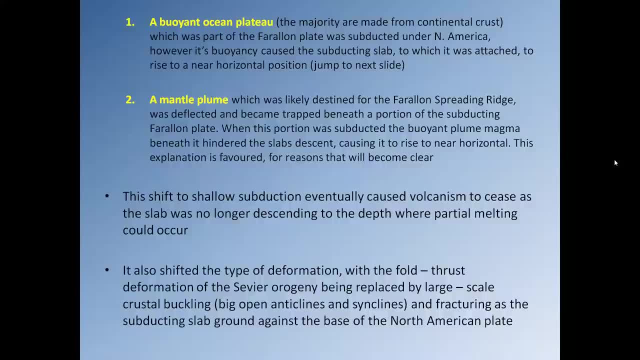 with a mantle plume stuck underneath it and you try and subduct that piece of oceanic crust. well, that piece of oceanic crust is not going to subduct well at all, Because once again, the oceanic crust wants to subduct down into the mantle. 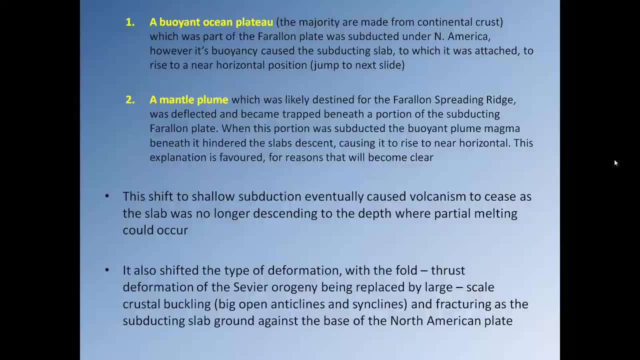 However, the mantle plume, which is extremely buoyant, will be pushing that piece of oceanic crust up, because the mantle plume naturally wants to rise, And so that would also lead to the farallon plate changing its angle of subduction from quite steep, you know, 45 to 50 degrees. 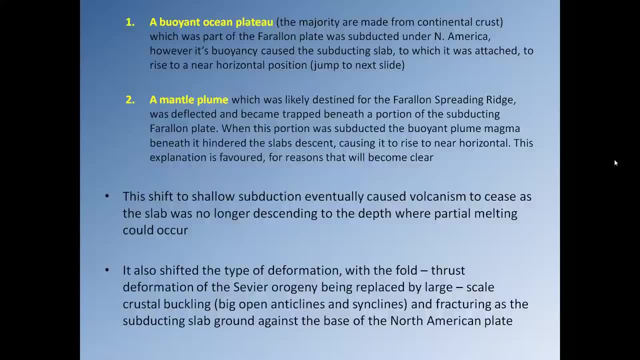 to a much, much shallower angle, Eventually near horizontal. At the moment the mantle plume hypothesis is the favoured model. So the shift to shallow subduction eventually causes volcanism to cease. That's because the farallon plate is no longer subducting down into the mantle. 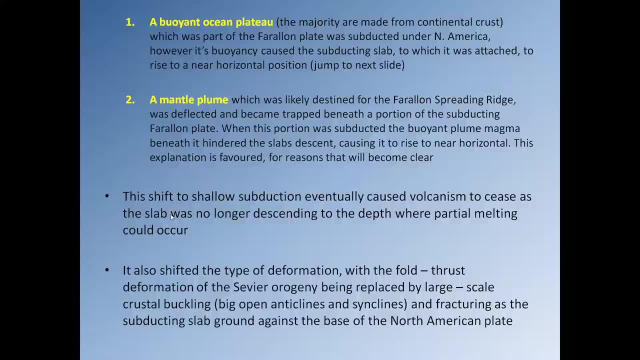 So it's no longer reaching the magic 150 kilometre number. So there's no melting, which means no magma, which means no volcanoes. So the Laramide Orogeny is not associated with volcanism. Most of the Laramide Orogeny is associated with. 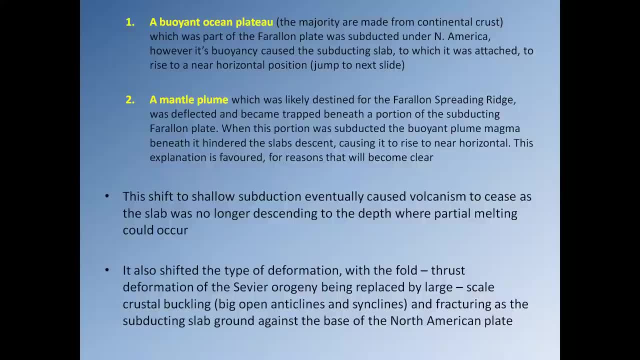 essentially big folds, big folding and some rather steep faulting. So what we see is it's a shift essentially in types of deformation. So when it comes to the Laramide- sorry, when it comes to the Vargin and the Sevier Orogenies, 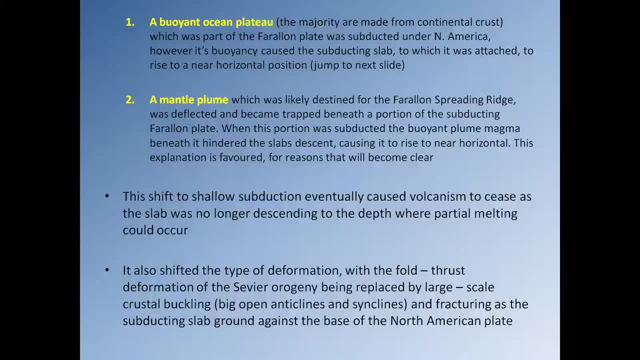 we have lots of folding and thrusting because we have lots of compressional forces being essentially put into a relatively small area of crust In comparison, the Laramide Orogeny, because the oceanic crust is grinding along the base of North America. 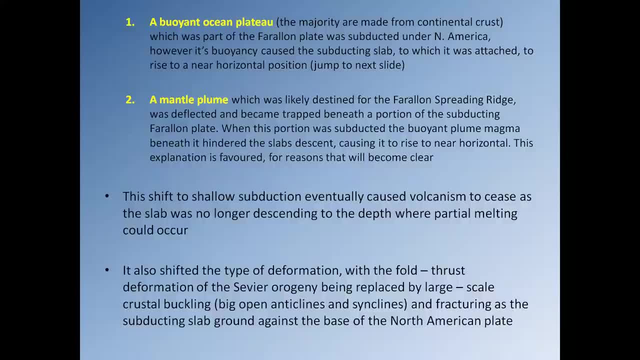 and so it's spreading out those tectonic forces over a very, very large area. we go from very, very focused compressional forces to very broadly distributed tectonic forces And this leads to crustal buckling. so very broad, big, open anticlines and synclines. 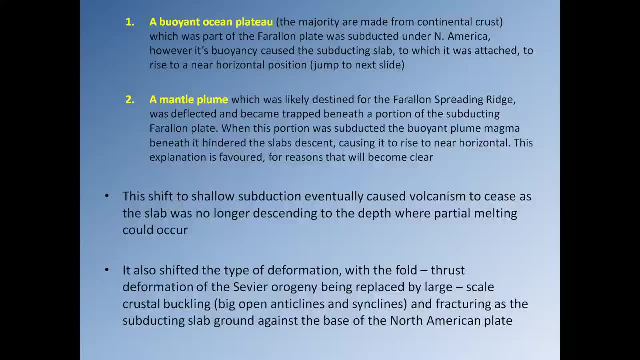 fracturing and faulting. So we see this very single, very significant change in the type of tectonism, the type of deformation associated with the Laramide Orogeny as well. So, in terms of the Laramide Orogeny, 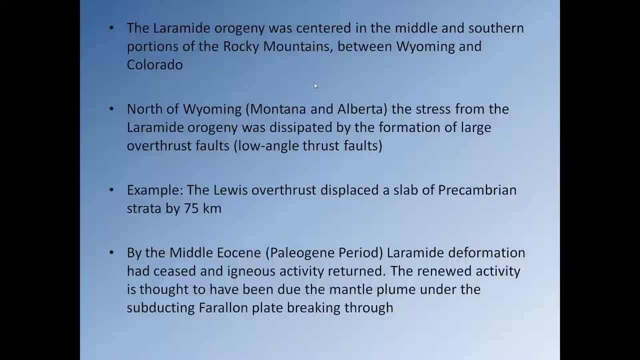 it was centred in the middle and southern portions of the Rocky Mountains between Wyoming and Colorado North of Wyoming, so that's essentially Montana Alberta kind of area. the stresses from the Laramide Orogeny were dissipated by the formation of a large thrust fault. 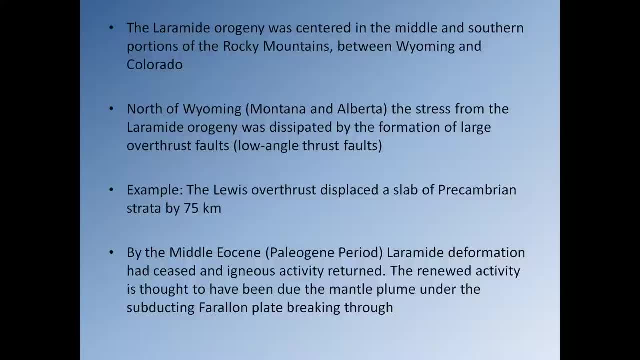 And so you know several large thrust faults, And arguably the biggest of these thrust faults is called the Lewis thrust fault, and that displaced the slab of pre-Cambrian strata by 75 kilometres. Now that might not seem very far. 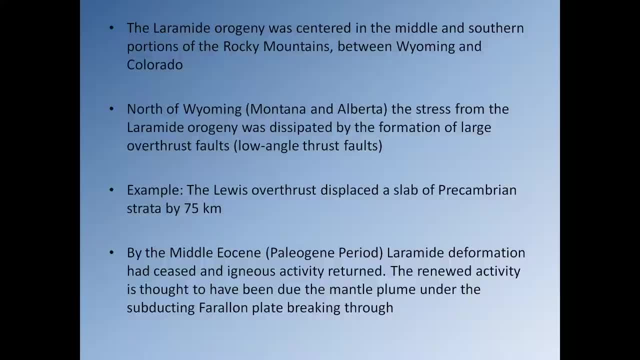 but think of the forces required to push a huge chunk of rock 75 kilometres across the Earth's surface. That's a lot of energy, So you know that does give you some idea of the size of the forces involved in this- By the middle Eocene. so that's the Paleogene period, once again. 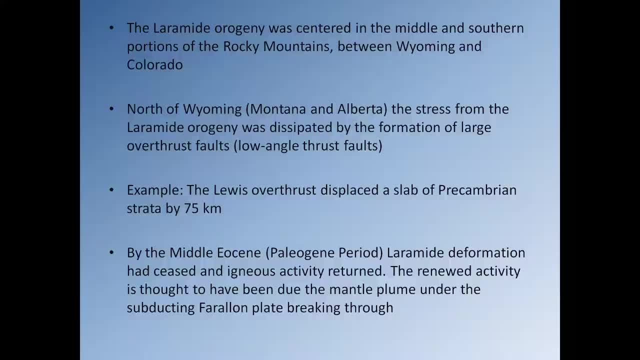 we have the Laramide deformation ceasing and igneous activity returning. So this suggests to us that whatever's been stopping the Faradon plate from subducting has stopped, and now the Faradon plate starts to subduct as it should do. 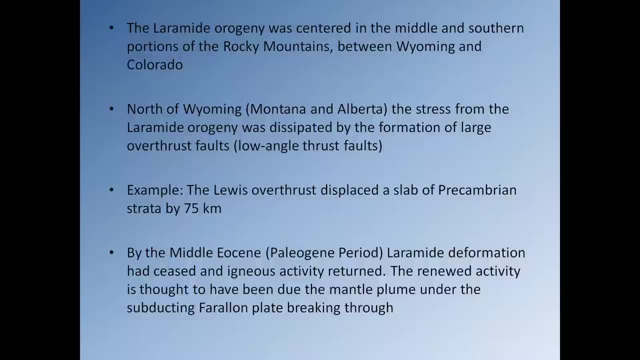 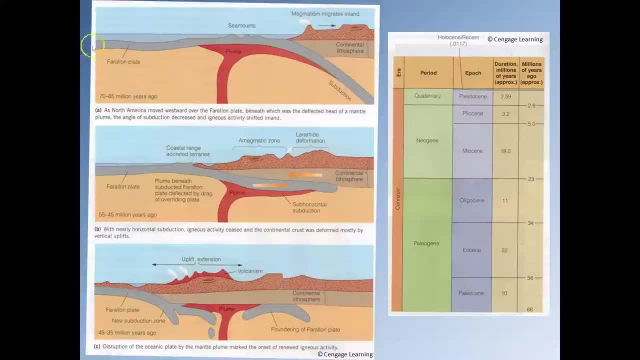 so it starts to dive down into the mantle again. And so why is this? Well, this is our current model. So here's the Faradon plate over here. So a new oceanic crust is being made, let's say over here, off to the left. 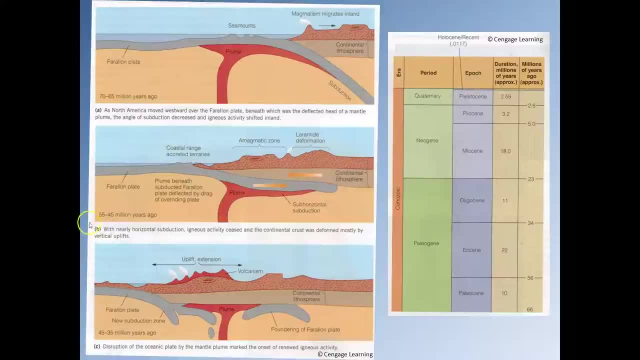 And typically when a mantle plume forms, it should follow the convection cells in the mantle and it should typically get stuck underneath the divergent plate boundary over here. That's normally what should happen. However, it would seem that about 70 to 65 million years ago, 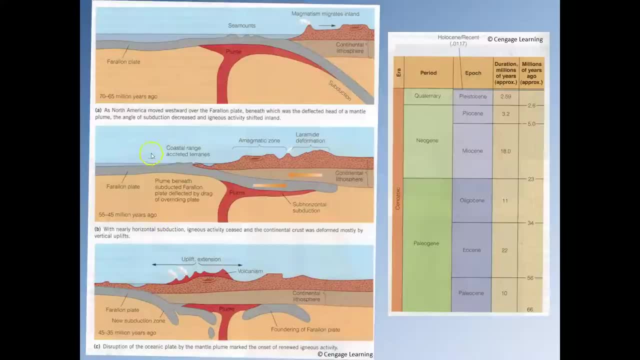 a mantle plume comes flying up from the core mantle boundary and instead of going over here to the divergent plate boundary, it instead gets deflected and it gets stuck underneath the Faradon plate. Now what this means is, as the Faradon plate begins to subduct eastwards underneath North America. 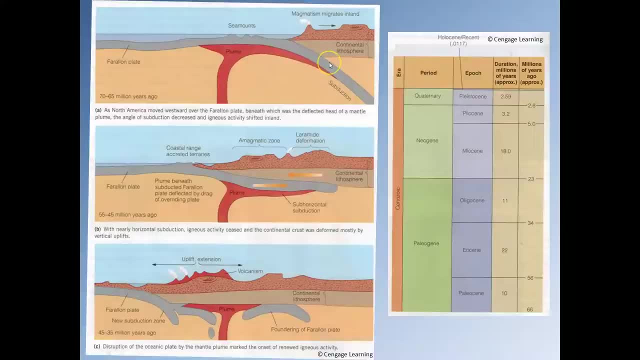 well, it takes the mantle plume stuck underneath it with it, And so, eventually, the mantle plume and the oceanic crust on top of it begin to subduct underneath North America. However, this mantle plume is extremely buoyant. 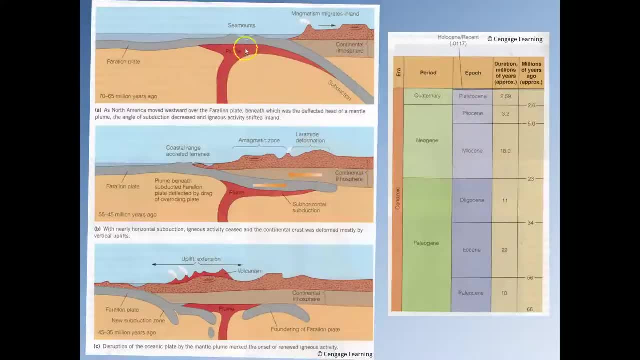 It wants to rise, It wants to go up, And so the subducting oceanic crust begins to be pushed upwards, upwards, upwards, until it's subducting at a near horizontal angle Now, because you have all the tectonic forces now being spread over this huge area here. 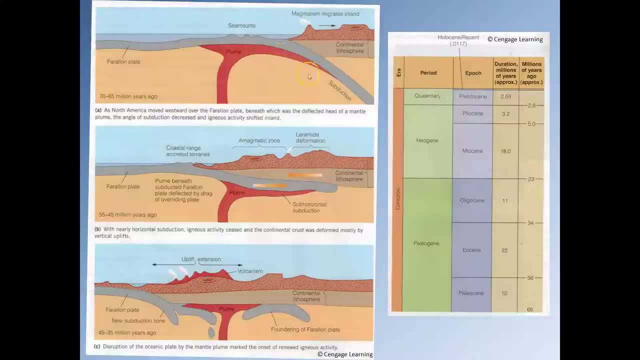 as opposed to this relatively compressed area. here it means that we have a shift from relatively strong, tight compressional tectonics to much broader open folding, because the tectonic forces are being dissipated over a larger area, so they're not quite as intense. 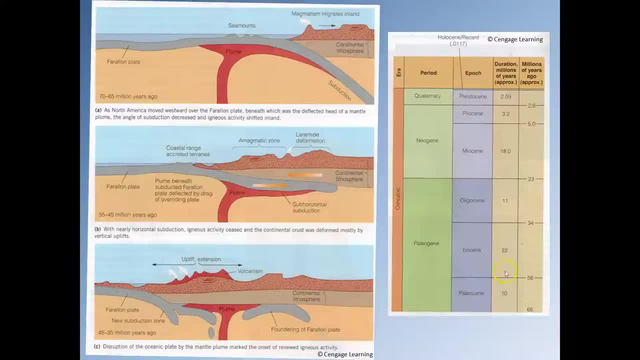 Now what happens? about 45 to 35 million years ago? so that's going to put us here in the middle to late Eocene. we see that all of a sudden, volcanism returns and we see the tectonism of the Laramide Orogeny stopping. 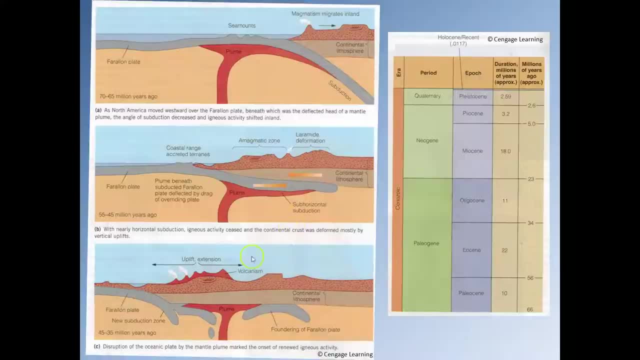 And so that strongly suggests to us that what's happened is is the mantle plume has eventually managed to burn its way through the oceanic crust. Now, once it burns its way through the oceanic crust, any bits of oceanic crust here just simply fall off down into the mantle. 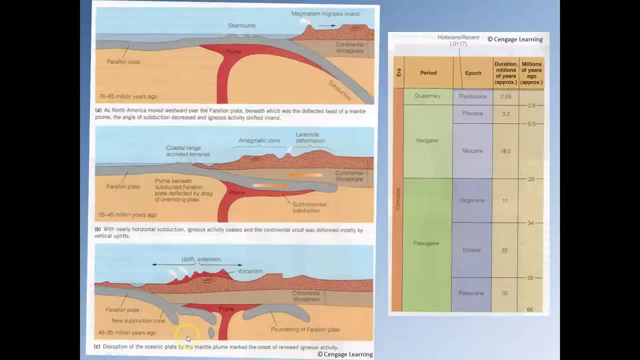 Now behind the plume, subduction starts again normally. Now that means that all of a sudden, all the tectonic forces are now focused back over here and the area which was being deformed by the Laramide Orogeny over here. 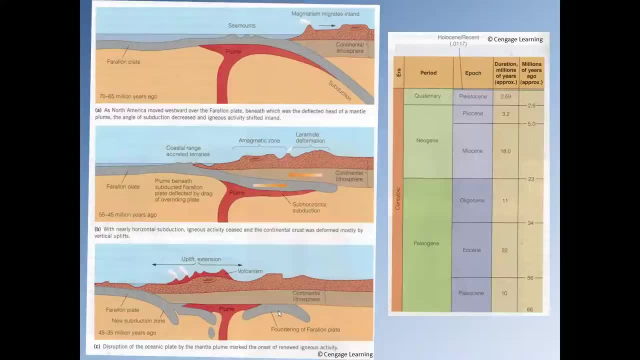 is now no longer being deformed. so we see Laramide deformation stopping Now because the plume has managed to burn its way through the oceanic crust. we now have a big mantle plume stuck underneath the continental crust here, which is obviously going to push magma towards the surface. 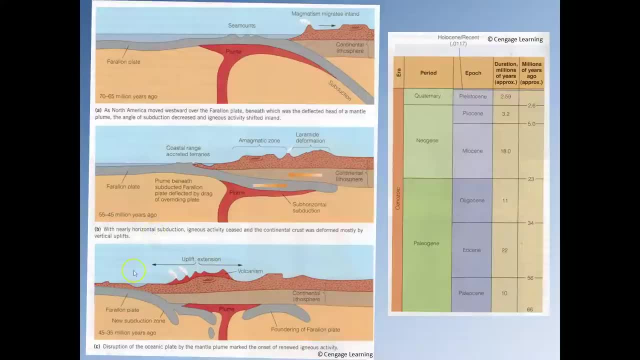 feeding volcanoes at the surface and eventually we have subduction going on here that's also going to produce magma that's going to rise to the surface as well. So for the mantle plume, we're going to see lots and lots of basaltic volcanism. 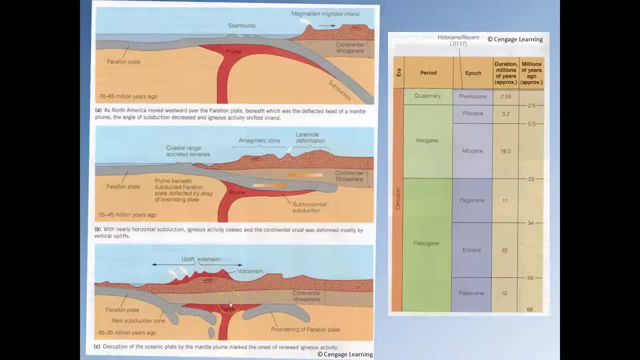 and that's then going to be followed by intermediate and felsic volcanism caused by the melting of the continental crust due to the heat from the mantle plume and any magma being formed by the restarting of the subduction of the Farallon Plate. 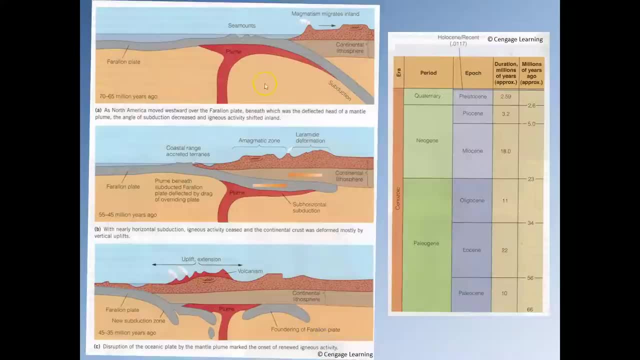 So I know it's a bit of a complicated situation, but I hope this diagram gives you a pretty general, pretty decent overview of what was going on during the Laramide Orogeny and why this shallowing of the subduction angle. 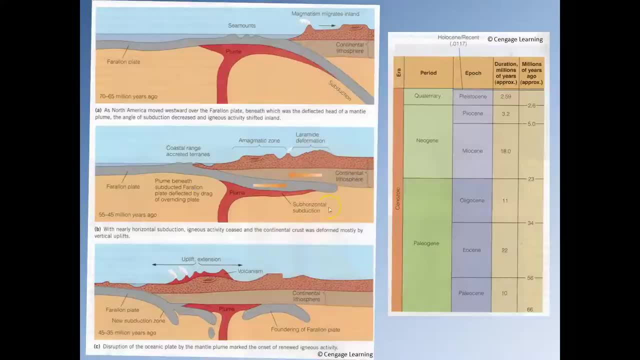 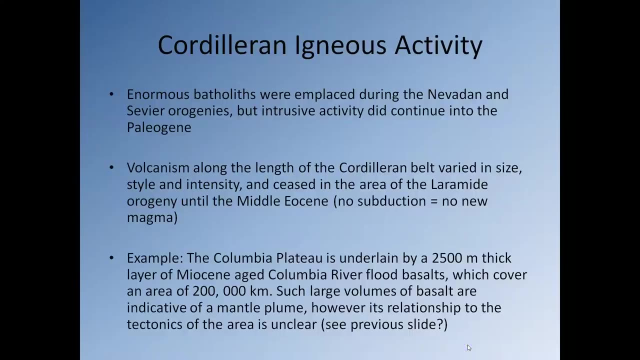 had such a serious caused serious changes when it comes to deformation and volcanism. So okay, so what about igneous activity during or within the Caudalierian region during the Cenozoic? So what we see? 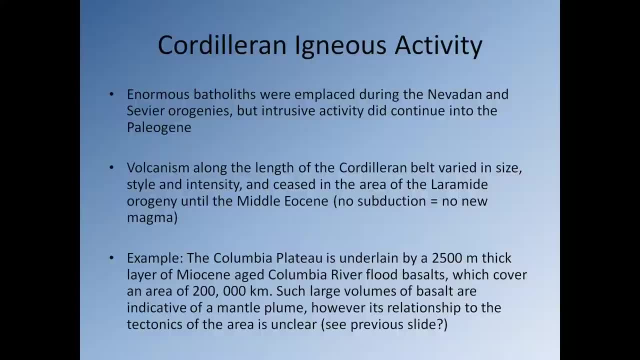 is, we see the intrusion of enormous bafflifts during the Navardian and Sevier Orogeny. So a bafflift essentially is a body of plutonic igneous rock that's typically made up of multiple smaller intrusions. 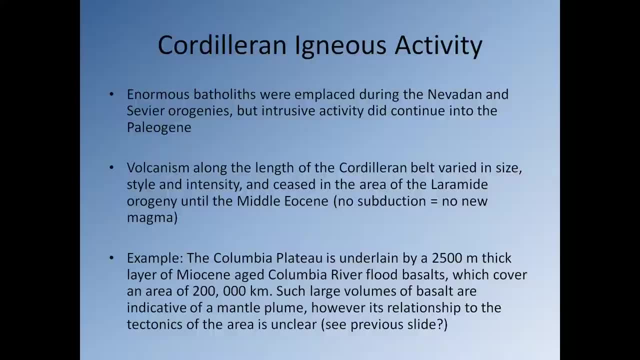 And these multiple smaller intrusions would have been feeding volcanoes at the surface of the Earth. So, of course, the magma chamber underneath the volcano is an intrusion and over time that magma chamber would have cooled down, solidified and it would have produced rocks like granite. 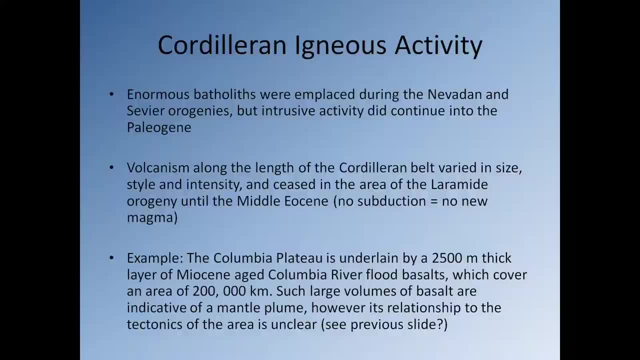 or granodiorite, And we can see these rocks within what's left of the Rocky Mountains. So volcanism along the length of the Caudalierian belt varied in size, style and intensity, And it ceased in the area of the Laramide Orogeny. 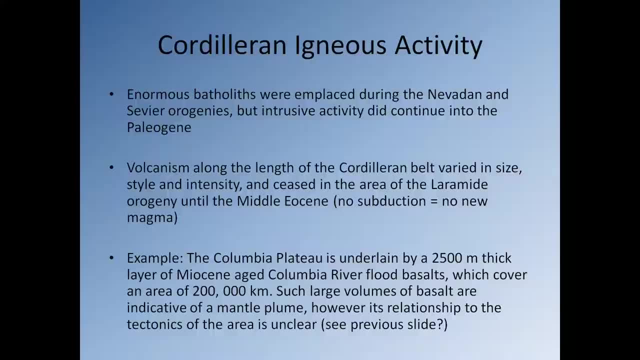 until the Middle Eocene. So, as I've already touched on, no subduction during the Laramide, Orogeny equals no new magma, which means obviously no volcanoes. So a good example of the types of volcanism that we see. 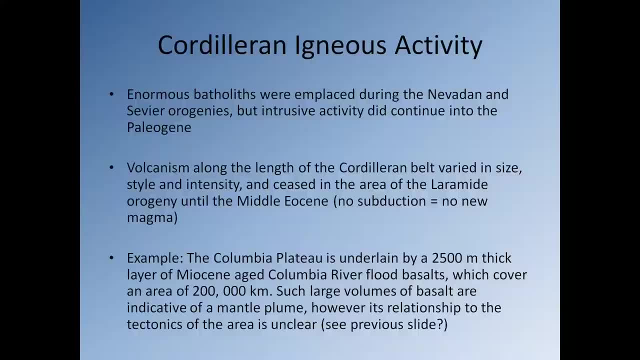 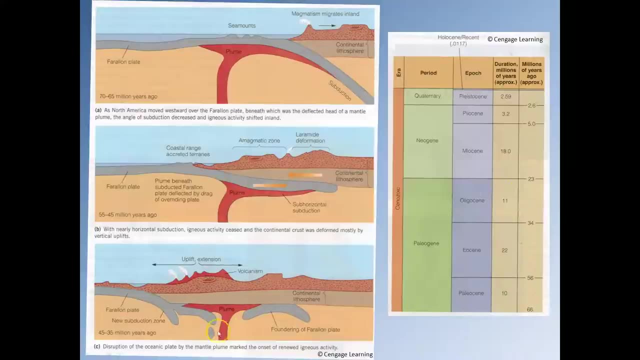 is the Columbia Plateau. So the Columbia Plateau is underlain by about two and a half kilometres of Miocene aged Columbia River flood basalts. So if we just come back to this diagram here, we know that essentially the plume begins to burn its way through. 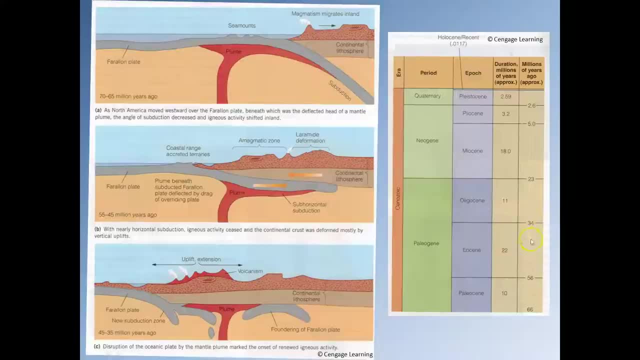 between about 45 and 35 million years ago. so around here And then here in the Miocene, we see suddenly a huge quantity of basalt pouring out onto the surface of North America, And chances are that's related to basalt from this mantle plume. 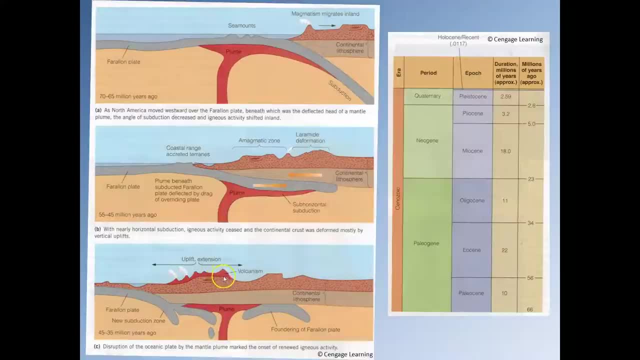 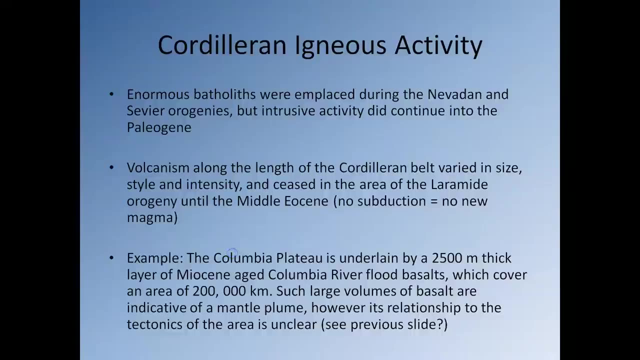 working its way steadily through the crust until it eventually reaches the surface, where it's erupted out as very large flood basalts. Oh, went too far there. No, it didn't. So if you want to know where the Columbia Plateau is. 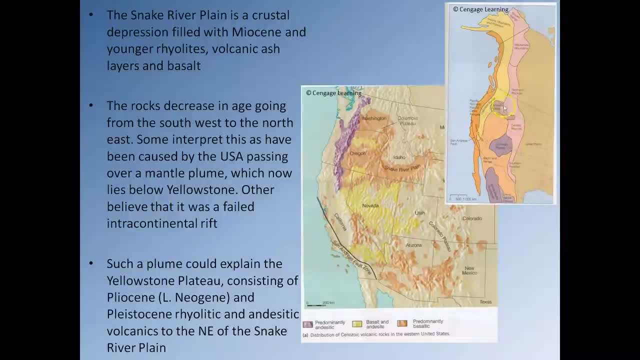 let's just have a quick hunt Here. it is right here, You can see it's got this rather distinctive shape there. So it consists of this area over here plus the Snake River Plain coming around here. So it's this region here. 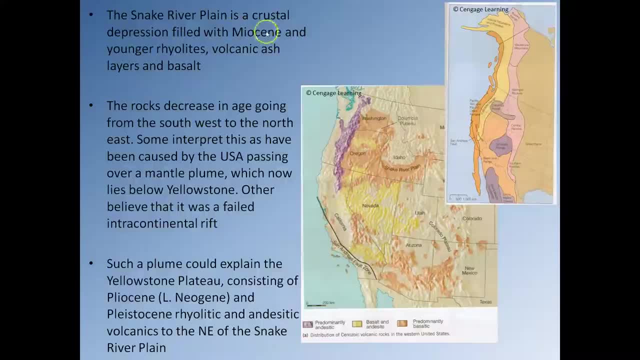 So the Snake River Plain is a crustal depression, once again filled with Miocene and Younger rhyolites, volcanic ash layers and basalt. So once again it's mostly underlain by basalt, And that's very, very important. 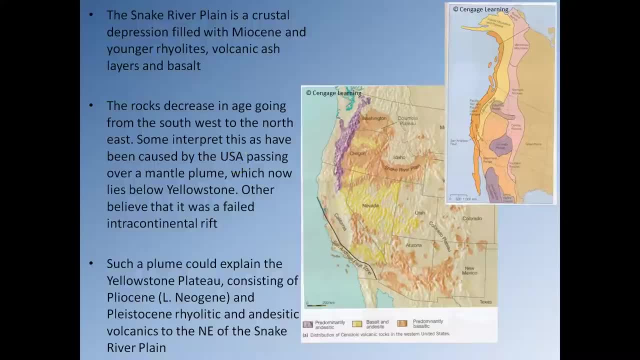 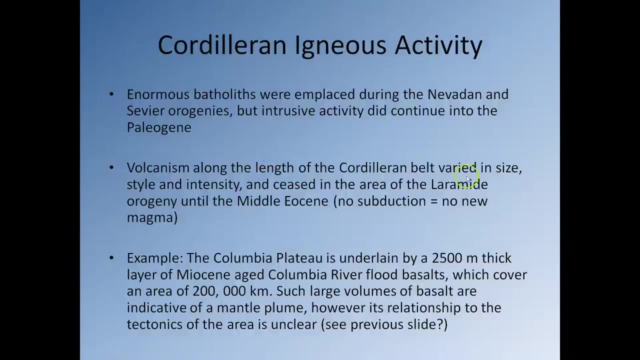 Basalt tends to form at either divergent plate boundaries, so in the middle of the oceans, pretty much so nowhere near this, or or it's associated with hotspots- mantle plumes, Think Hawaii, think Iceland. And so what we have here during the Miocene, 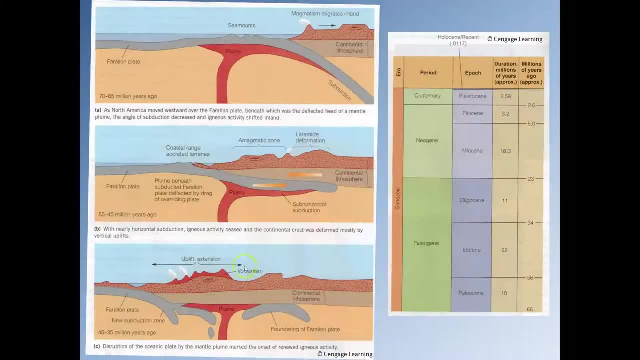 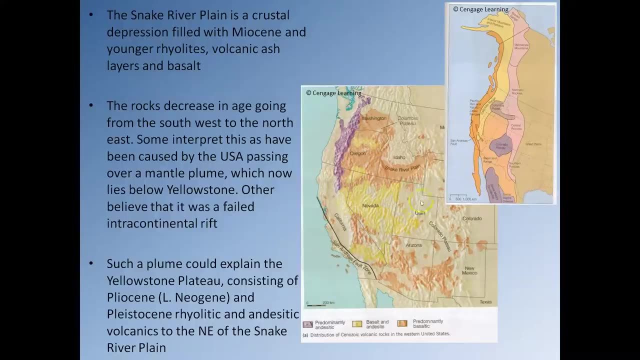 so up here is, it looks like we have huge eruptions, very, very large quantities of basalt, probably coming from the mantle plume, pouring out onto the surface of North America, giving us the Columbia Plateau. So when we look at the Snake River Plain especially, 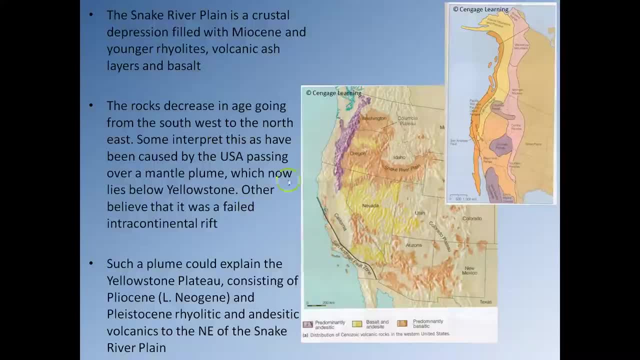 the rocks decrease in age, going from the southwest to the northeast. So the rocks of the Snake River Plateau get younger as we come in, move in this direction. So the youngest rocks will be over here. the oldest rocks will be over here. 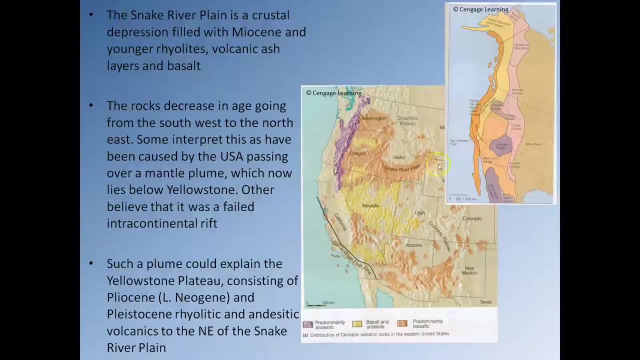 And it just so happens that right here at the tip of the Snake River Plain, is Yellowstone And, as I'm sure we've discussed by now, Yellowstone is the location of a mantle plume. So we know that under underneath Yellowstone we have a mantle plume. 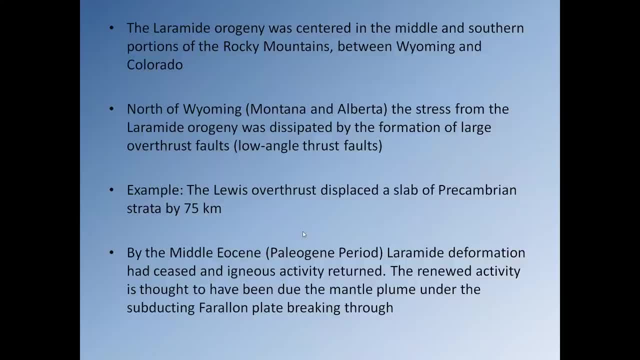 Oh, going the wrong way again. We have a mantle plume. Sorry about this, everyone. There we go. We have a mantle plume, just like this one stuck underneath Yellowstone, And so that would help to explain, you know. 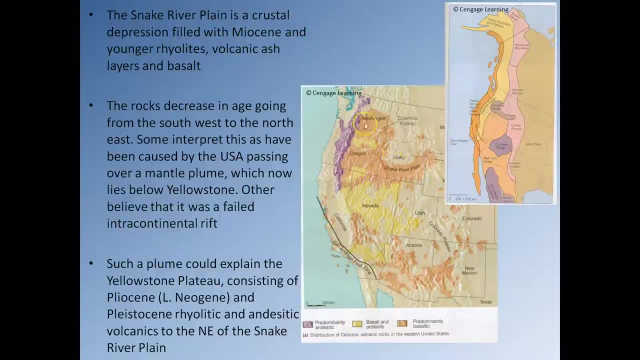 quite effectively where the basalts for the Snake River Plain and the Columbia Plateau actually came from. So, as I said, such a plume can explain the Yellowstone Plateau consisting of Pliocene, Late Neogene and Pleistocene. 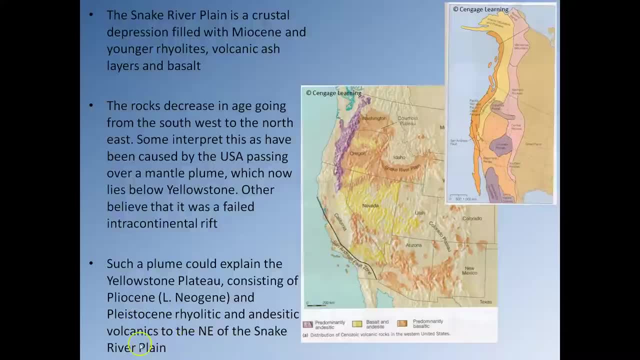 rhyletic and anisitic volcanics in the northeast of the Snake River Plain. So this northeastern portion here is referred to as the Yellowstone Plateau And that consists of rhylites and andesites related to the Snake River Plain. So you're thinking 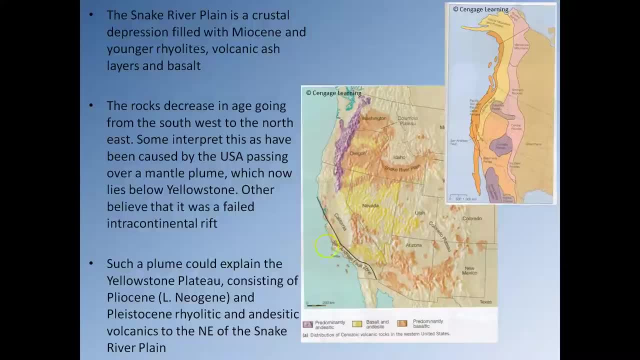 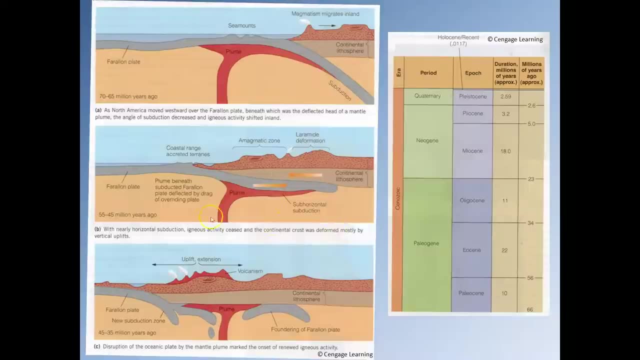 hold on a minute. I just said that you know mantle plumes will give you basalts. Of course, if you remember, the mantle plume will. I'm going the wrong way again. The mantle plume will melt the continental crust. 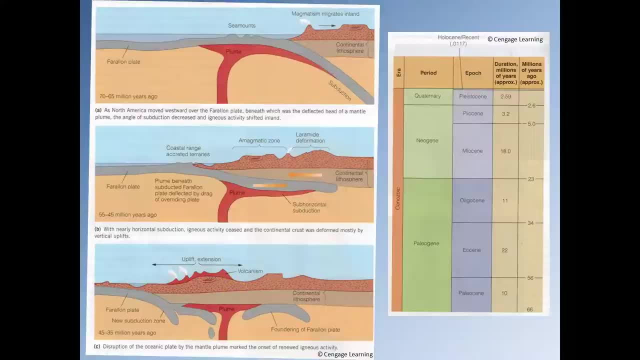 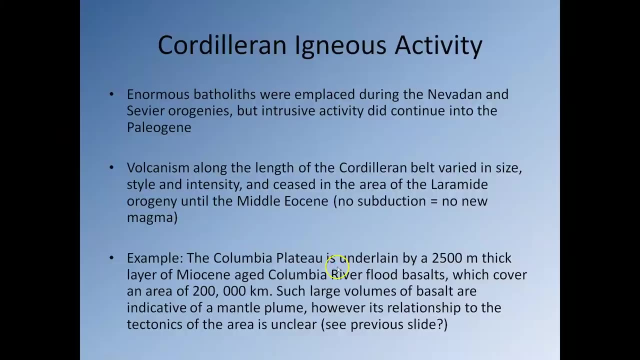 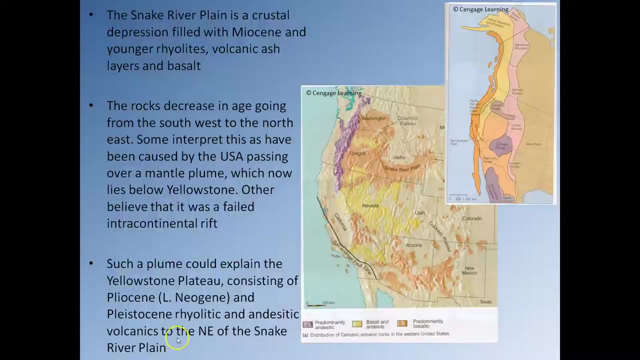 and that will eventually lead to the formation of felsic and intermediate magmas, And they will then rise to the surface, feeding volcanoes. So what we're seeing is we eventually see the melting of the continental crust caused by the plume. Now that's essentially occurring now. 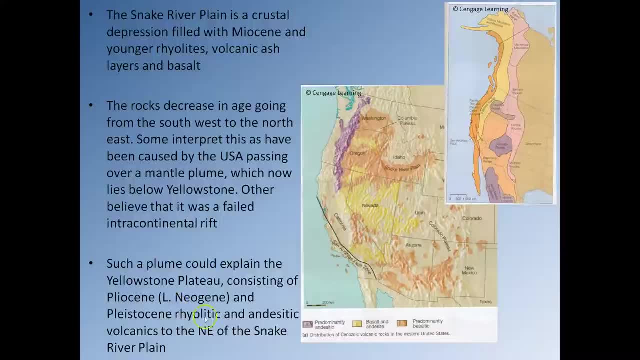 in the modern day Yellowstone area And that produces felsic and intermediate magmas that rise to the surface, feeding volcanoes. So we can see we have a big area here that's covered in, you know, huge quantities of basalt. That's a very, very large flood, basalt eruption. 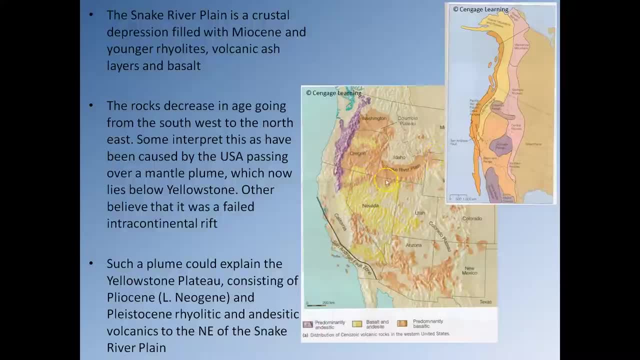 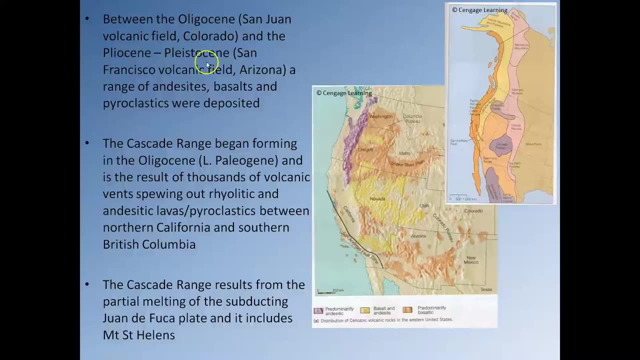 And then steadily, as the plume moves this way, we begin to see less and less basalt being put out. So it means the plume is starting to slowly run out of material. So, between the Oligocene and the Pliocene-Pliocene, 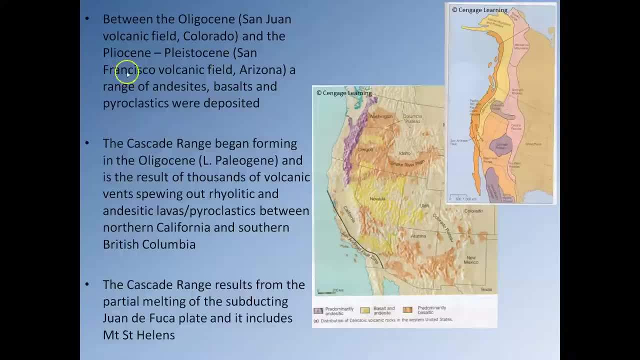 we have the San Juan and the San Francisco volcanic fields located in Arizona. So they're down here, Okay, And we see they are formed by a range of andesites. Once again here it is, again Basalt and pyroclastic rocks. 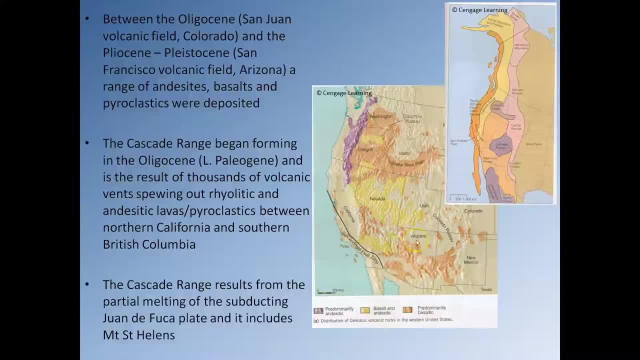 Once again, this is very likely related to some kind of mantle-plume related volcanic activity. Just like up here, Same thing happening down here. So it looks like the mantle plume that you know had affected the farrow and plate had very serious impact. 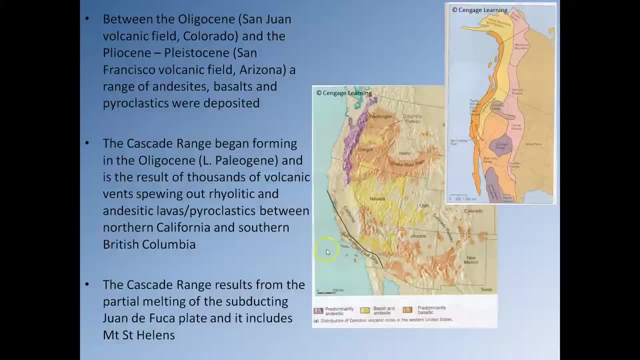 and very serious repercussions for very large, for a very large portion of the western United States In terms of this purple region up here. well, that's the Cascade Range. And the Cascade Range began forming in the Oligocenes, That's the late Paleogene. 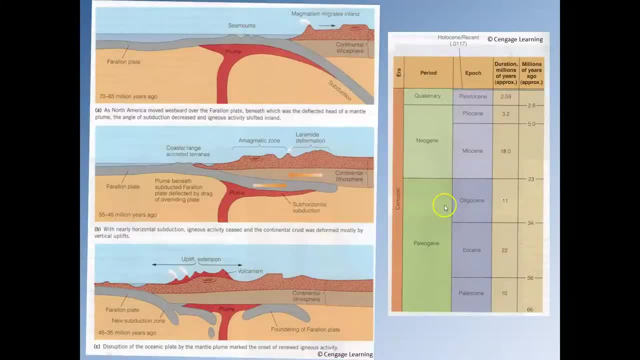 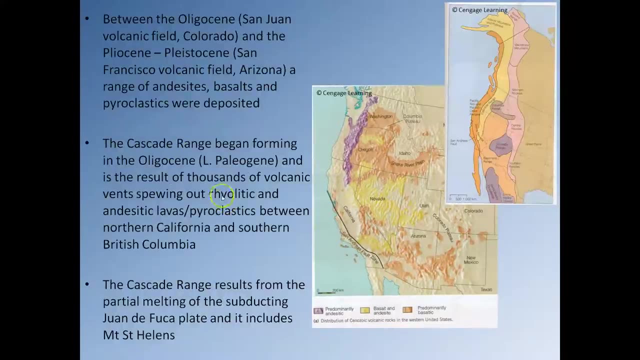 So if we go back up for a second? So here's the Oligocene here. Let's see where am I. Sorry, I lost my place there for a second And it's the result of thousands of volcanic vents spewing out rhyolitic and andesitic lavas. 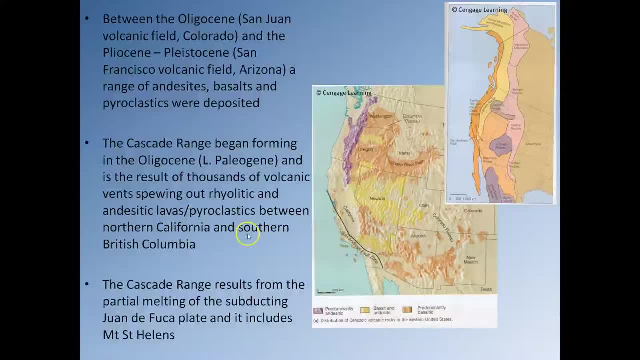 pyroclastic materials between Northern California and Southern British Columbia. So what happened is, although subduction stopped here and up here in Canada, there's a region of the west coast of North America, here through Washington State, Oregon and into Northern California, that is still undergoing subduction. 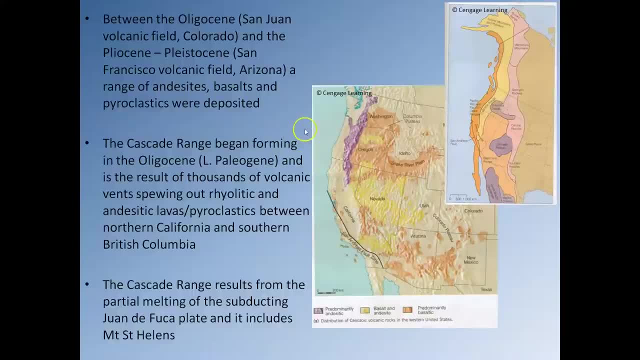 There's a very little piece of oceanic crust here which is subducting underneath North America. obviously it's melting when it gets to 150 kilometres, producing magma which is rising to the surface to feed the volcanoes of the Cascade Mountains. So the Cascade Range results from the partial melting. 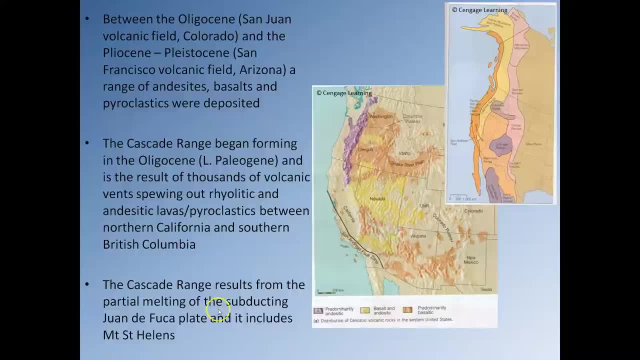 of the subducting Juan de Fuca Plate, and it includes Mount St Helens, Mount Baker, Mount Rainier are all members of the Cascade Mountains. So the question becomes obviously: well, where does the Juan de Fuca Plate come from? 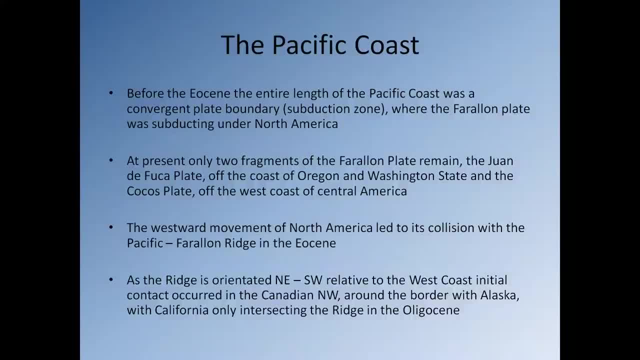 And that will be explained in a minute. Ah, do you know what? This is the perfect time to stop for a quick break, So please pause the presentation, get up, have a walk around and go and get a glass of water. 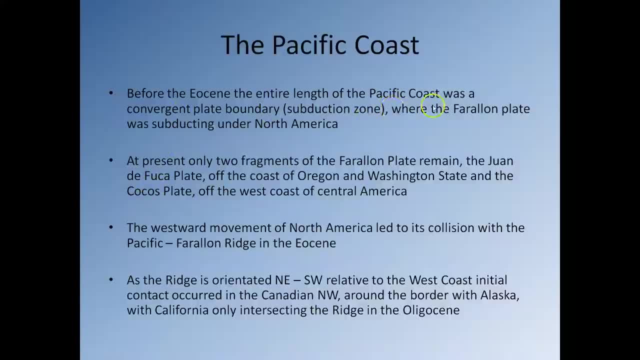 So before the Eocene the entire length of the Pacific Coast was a convergent plate boundary. It was one long subduction zone And that was because the Farallon Plate was subducting under North America- At present- only two fragments of the plate. 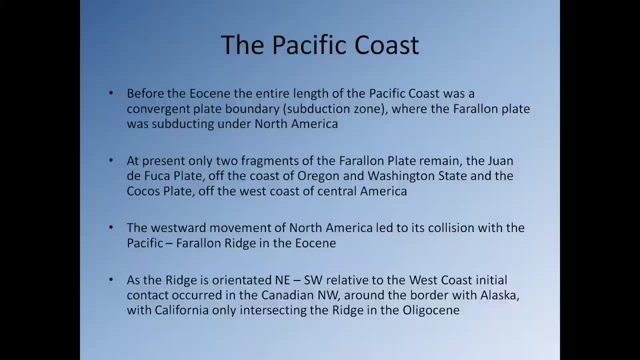 remain and they've been renamed. The northern fragment is called the Juan de Fuca Plate, and that's off the coast of Oregon, Washington State and California, And the southern fragment of the Farallon Plate is now called the Cocos Plate, and that's off the west coast of Central America. 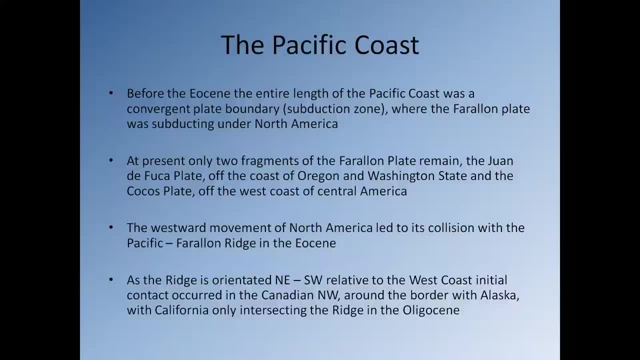 So the western movement of North America led to its collision with the Pacific Farallon Ridge in the Eocene. That's the divergent plate boundary that was producing the Oceanic Farallon Crust. Now, obviously, once that spreading ridge, that divergent plate boundary is subducted, 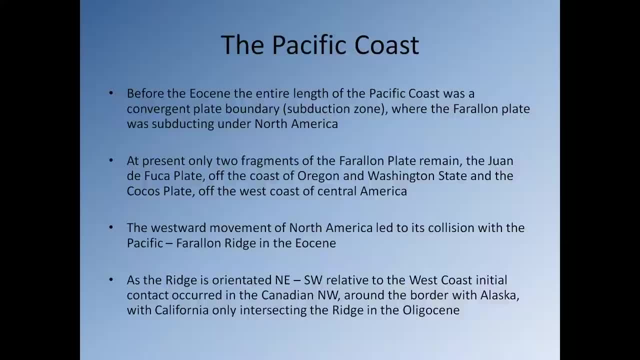 of course that's going to lead to very significant changes in the tectonism experienced by the west coast. So, as the ridge was orientated northeast-southwest relative to the west coast of North America, the contact, the initial contact between North America, 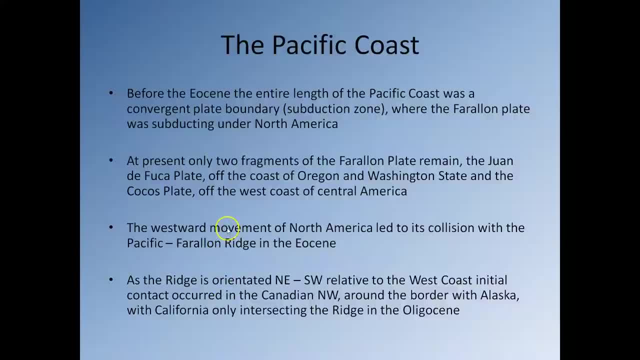 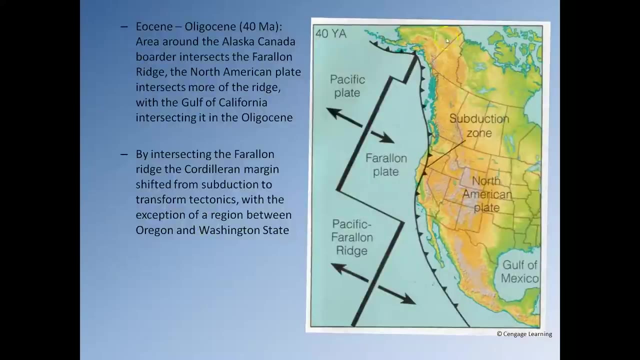 and this Farallon Ridge occurred in an area that's approximately around the Canadian-Alaskan border, And so because the ridge was orientated in such a way, it means that more and more of the ridge has been subducted over time. So this is the situation around 40 million years ago. 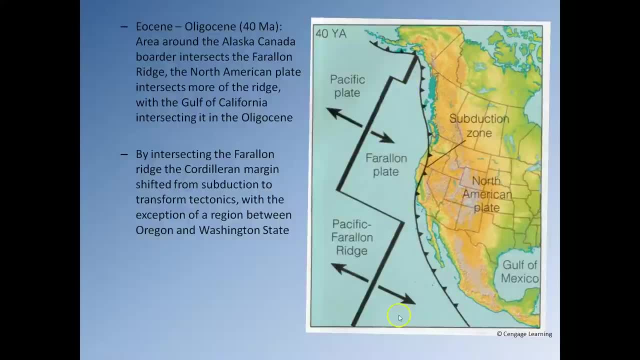 Here's the Farallon Plate. so it comes all the way along here. Here's the subduction zone associated with it. So here's the subduction that runs down here. This is where the subduction plate is being subducted underneath North America. 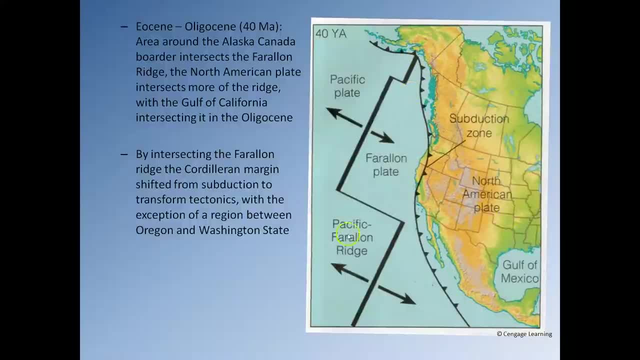 Now you'll notice that the ridge is orientated approximately northeast-southwest, And so the initial contact between the Farallon Ridge here and the North American Plate here occurs around the Alaskan-Canadian border. Now what's going to happen is is as North America moves westwards. 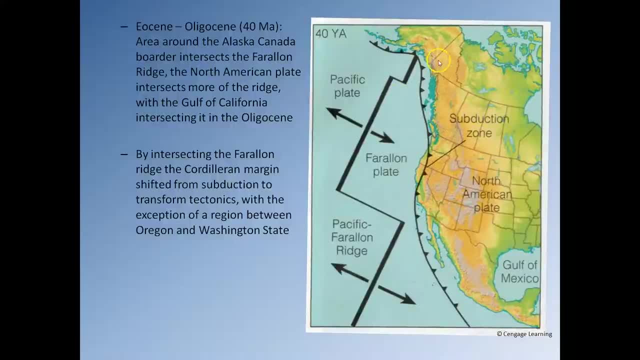 it's obviously going to keep rolling over this portion of the ridge here and it's going to subduct it And obviously it's eventually going to start rolling over this portion of the ridge here And that's going to cause the Farallon Plate. 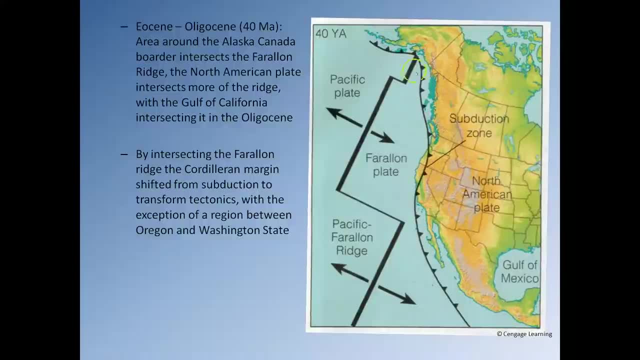 to be cut in two. You're going to have a northern fragment up here and a southern fragment down here. This will become the Juan de Fuca Plate and this will become the Cocos Plate. So let's see, by intersecting the Farallon Ridge, 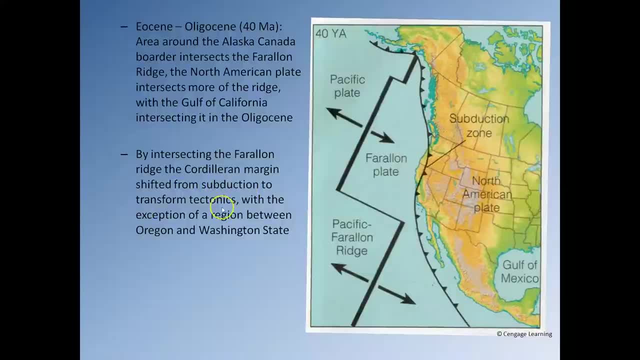 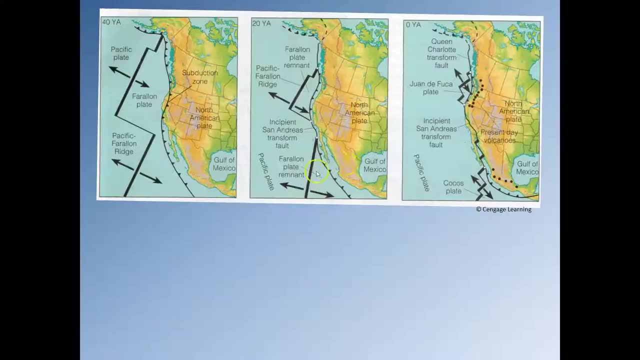 the cordillera margin shifted from subduction to transformed tectonics, with the exception of a region between Oregon and Washington State, And the next slide is going to show that. OK, so this is what we just saw a second ago. 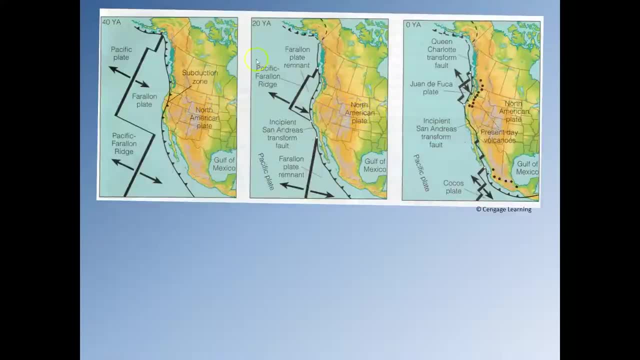 And as North America keeps moving westwards, it begins to override this portion of the Farallon Ridge and this area down here. Now this means that we have this area of Farallon Crust left, so that becomes the Juan de Fuca Plate. 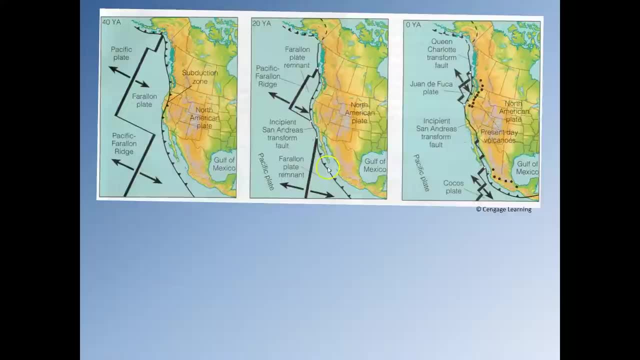 and this becomes the Cocos Plate down here. Now what's happened at this point is we have a problem. Well, as there's nothing pushing the Oceanic Crust over here eastwards anymore, it means this subduction zone stops. Same up here. 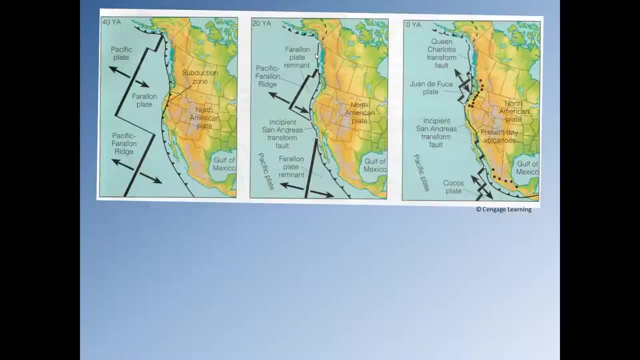 You can't have subduction there anymore because there's nothing pushing the Oceanic Crust eastwards. So alright, we have a problem. The other problem is that the Pacific Crust, the Pacific Plate, is moving in an approximately north-westerly direction. it's moving up here. 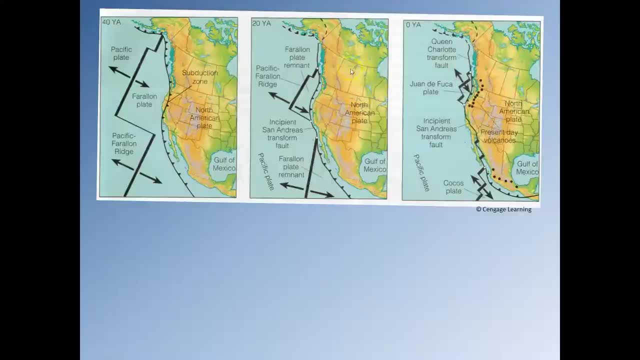 So even if North America wants to try and override the Pacific Plate, it can't do it because the Pacific Plate is trying to move this way towards the northwest, so it's essentially running away. So the North American Plate might be trying to move westwards. 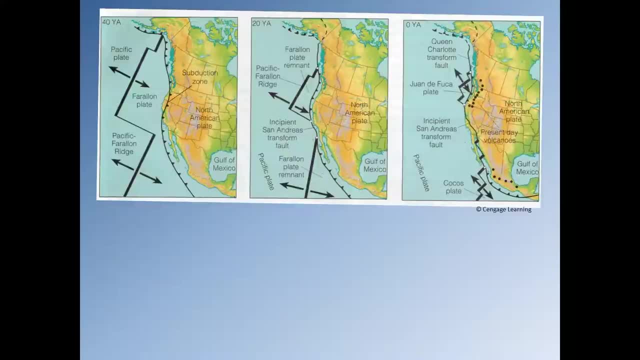 it might try and subduct the Pacific Plate, but it can't because the Pacific Plate isn't helping. So what happens instead, then, is you have a situation where the North American Plate can't override the Pacific Plate, so that means no more convergent plate boundary. 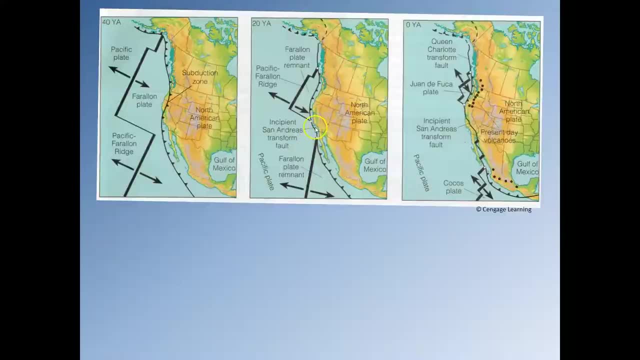 There's obviously you have the wrong tectonic setup for a divergent plate boundary, so that can't happen, And so all that can happen is you have to have a situation where the Pacific Plate just starts to move past the North American Plate. 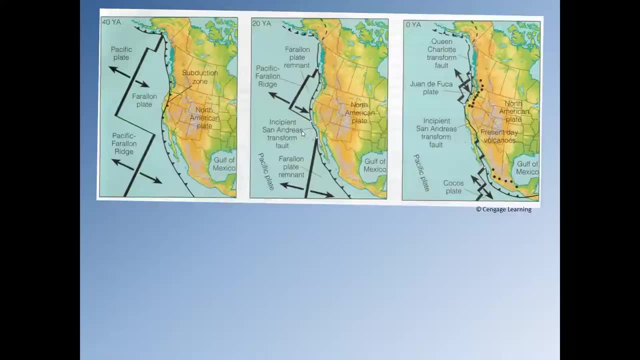 And so we have a transform plate boundary forming, And of course, this transform plate boundary is well known: it's the San Andreas Fault. Up here we have another transform boundary. this is called the Queen Charlotte Fault. Well, I should say it's the Queen Charlotte Fault in Canada. 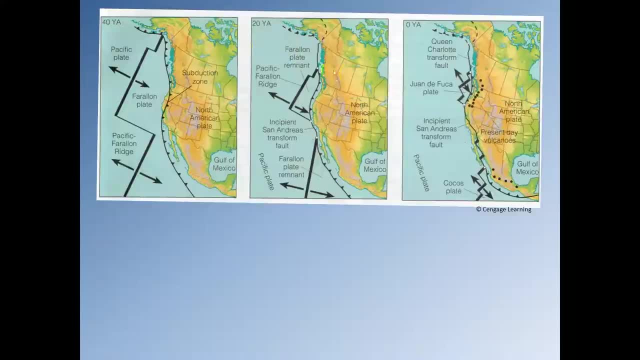 it becomes the Fairweather Fault in Alaska, And you can see that the present day situation is is a large proportion of the spreading ridge here has been subducted. we only have a small fragment of it left here, just off the coast of Oregon and Washington State. 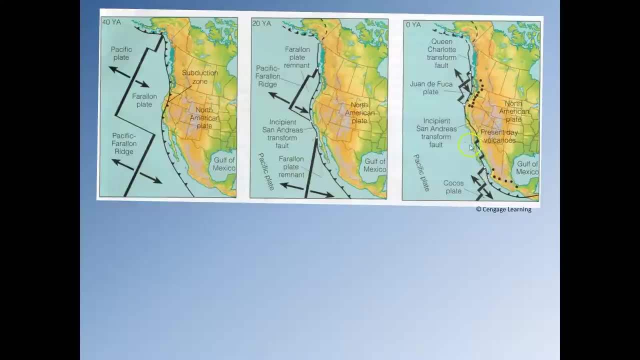 And we have a fragment of it remaining down here off the west coast of Central America, And so that's why we have volcanism up here in the Cascades and why we have volcanism down here in Central Mexico. So that explains why we have this shift. 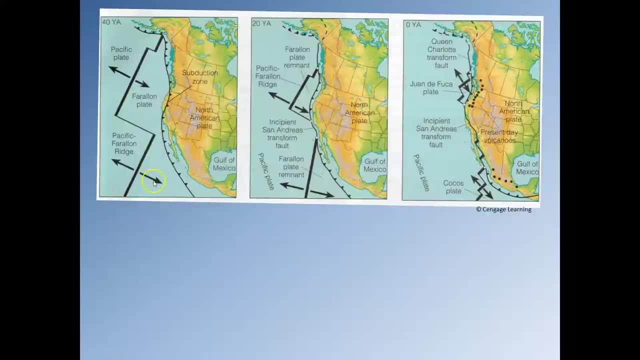 from a long subduction zone here around 40 million years ago to a transform boundary here where the Pacific Plate is moving northwestwards and North America obviously is moving approximately westwards, give or take a little bit. So during the Miocene we obviously form two triple junctions. 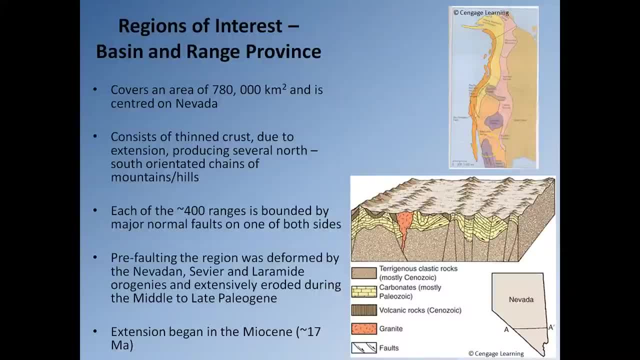 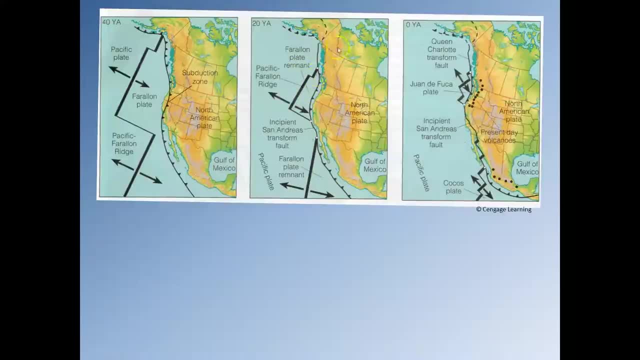 and that's a place where we have three plates meeting at the same location, So you can see. so here we have a triple junction, here we have the Farallon Plate, the Pacific Plate and the North American Plate meeting, And here we have the Cocos Plate. 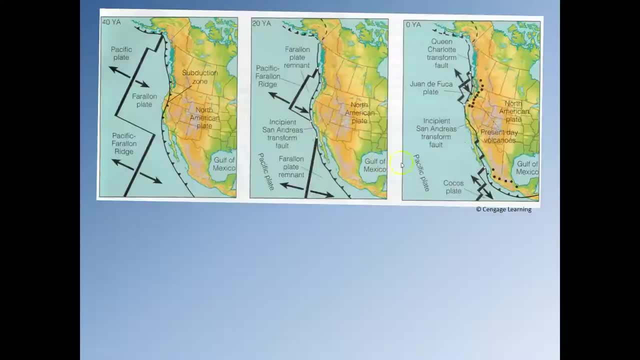 North American Plate and Pacific Plate meeting. And what you can see if you look at the position of these white dots is you can see they are steadily moving westwards, moving down and up the subduction zone as more and more of the spreading ridge gets subducted. 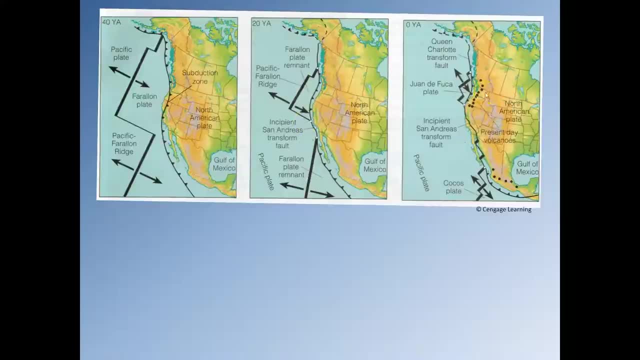 And so we can see that the length of the subduction zone gets smaller and smaller as we go from 20 million years ago to the present day, And eventually North America is going to completely roll over this spreading ridge here, at which point the west coast of North America 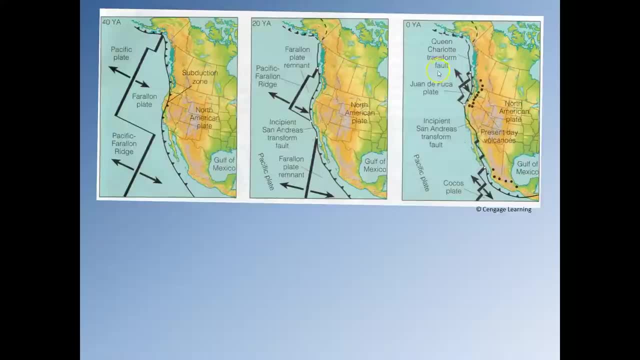 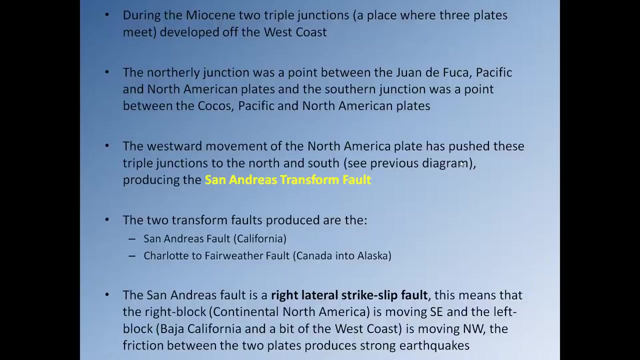 is going to become one long, continuous transform plate boundary And once again, eventually, Mexico here is going to override this spreading ridge over here and once again that's going to turn this area probably into a large transform plate boundary as well. So let's see. 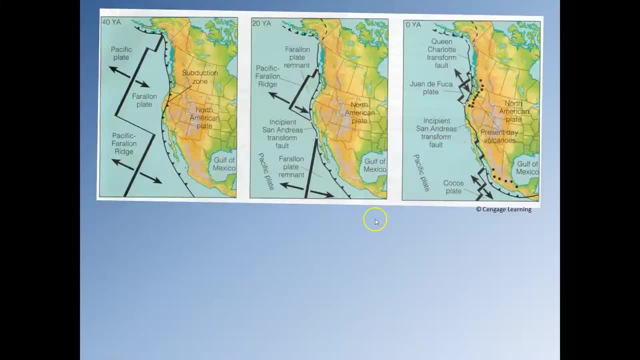 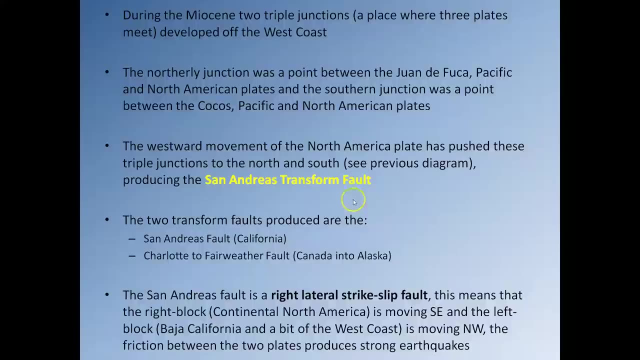 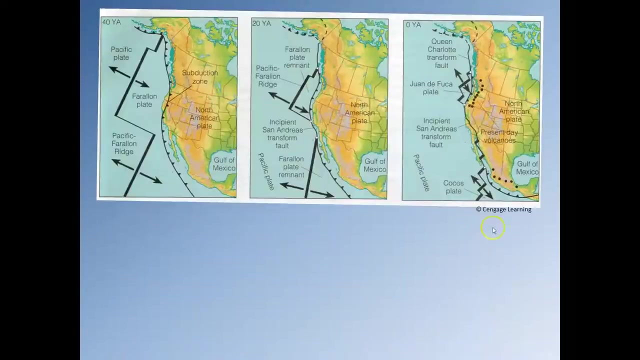 So the two transform faults produced by this movement of the North American Plate westwards, as discussed are the San Andreas Fault and the Queen Charlotte Fault. So the San Andreas Fault is a right lateral strike-slip fault. So the piece of crust over here on the right 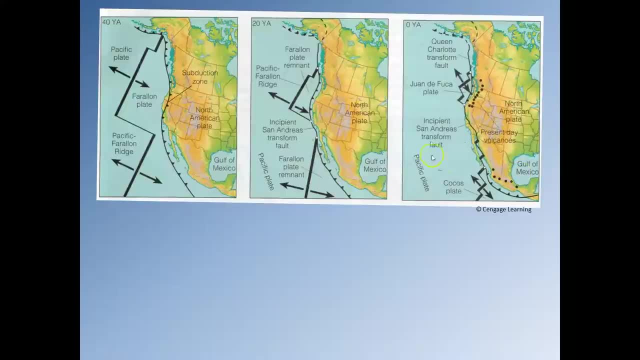 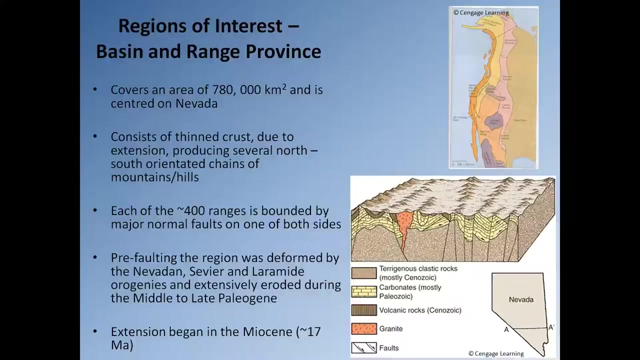 is moving down towards the southeast, And that means, conversely speaking, the Pacific Plate and this little bit of California here is moving off towards the northwest. OK, so that was where the San Andreas Fault comes from. So now we're going to look at another area. 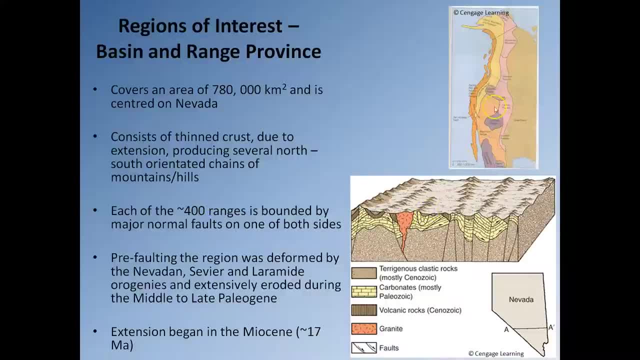 We're going to focus on the Basin and Range Province. So the Basin and Range Province is this area here marked out in this kind of peachy orange. So, as you can see, it's an extremely extensive area. Essentially, it's in both the United States. 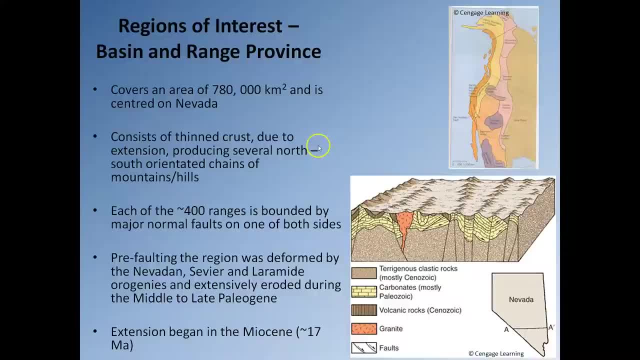 and it goes down into northern Mexico as well. So it covers an area of around 780,000 square kilometres. It's centred mostly in Nevada, but it does cover a broader area, So this entire area consists of thinned crust due to extension. 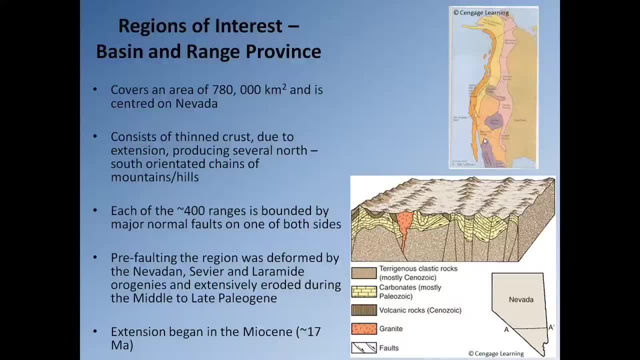 So this entire area is being stretched and it produces several north-south orientated chains of relatively large hills to small mountains, depending on how you want to classify them, And these are referred to as ranges. So these sets of hills, sets of small mountains, 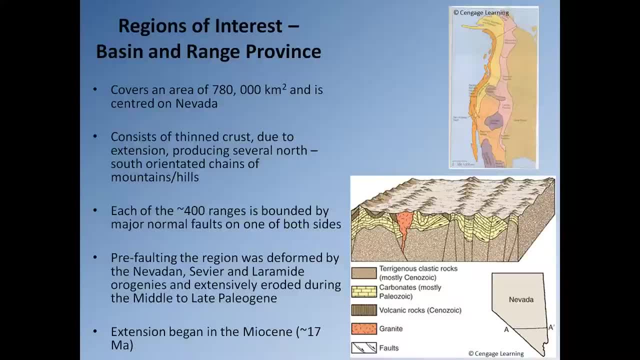 are referred to as ranges, And there's approximately 400 of them, And these ranges are bounded by normal faults, So they have faults either on one side or both sides of them. So, before the fault occurs, the region was deformed by the Nevadian. 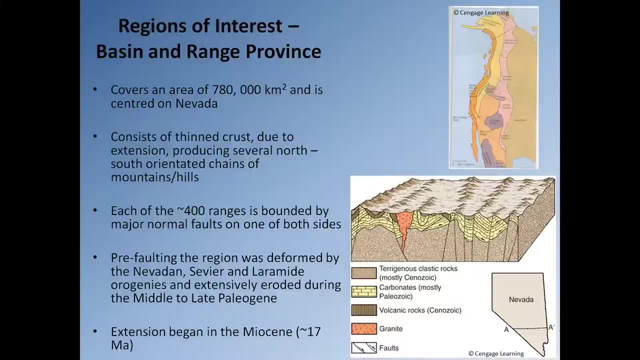 Sevier and Laramide orogenies And it was extensively eroded during the Middle and Late Paleogene. So the area was deformed, so there was some faulting, lots of folding in the area And then of course, the Laramide orogeny stops. 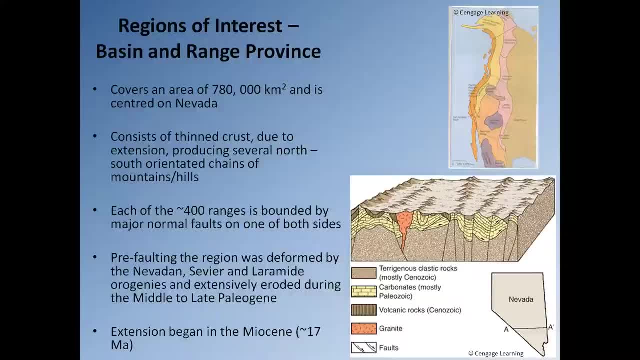 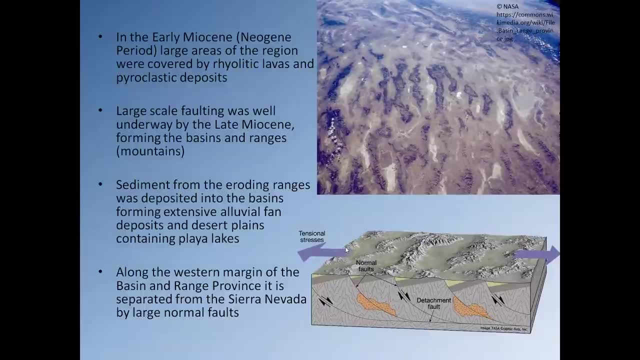 There's a period where the crust is exposed, There's lots of erosion And then we have extension beginning around 17 million years ago, That's during the Miocene. So this is a picture of the Basin and Range Province. This is some space. 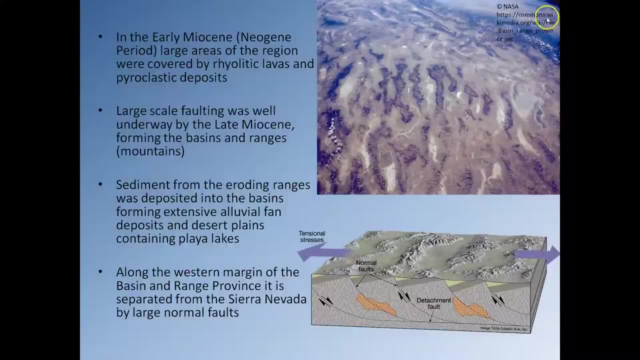 You can just see the curvature of the earth up here in the top right corner And you can see you have these linear bands of very large hills or small mountains running approximately north-south And you can see in between them you have these valleys. 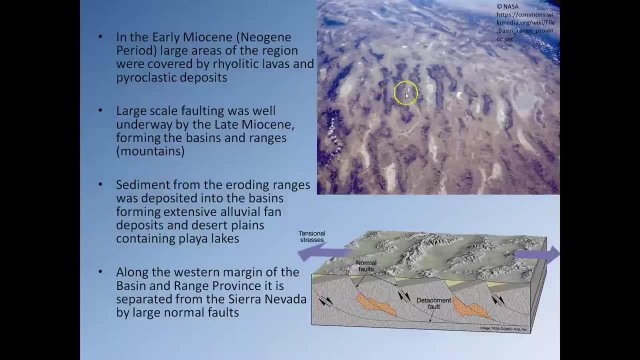 So the mountain ranges are called the ranges, And the bodies of land between them are obviously the basins, hence the name Basin and Range Province. So in the early Miocene we get large areas of the region being covered by rhyolitic lavas. 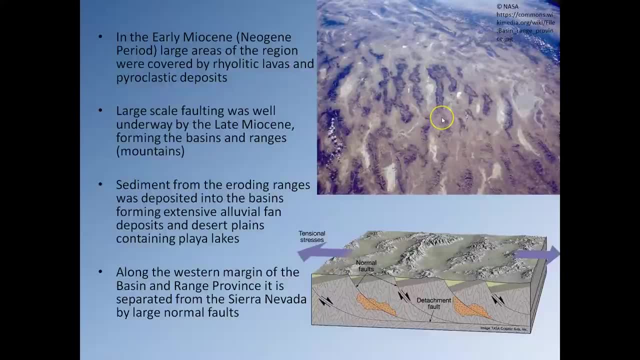 and pyroclastic deposits. So there was lots of volcanic activity And this is probably the result of large-scale faulting started Because, remember, faults are the perfect pathway for magma to move, for magma to move through, So as soon as a fault opens up, 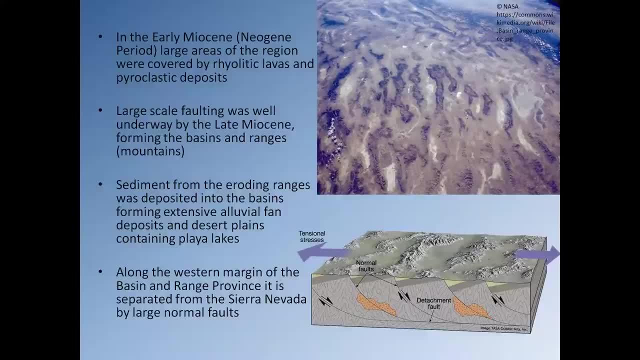 it's a weak point along which magma can move very, very easily. So as soon as the area starts to undergo extension and these faults start to form well, it means that magma can start to move up along them relatively easily, And that leads to the formation of lots of. 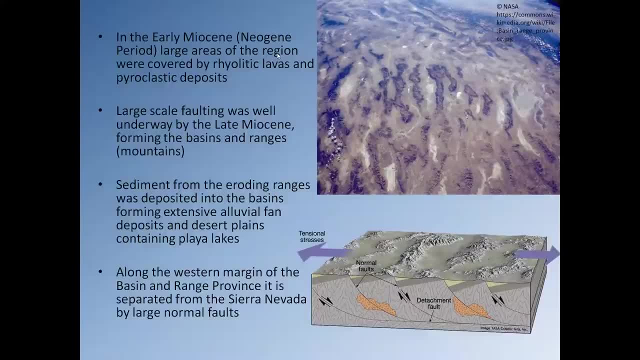 you know, felsic and intermediate volcanoes, And so this area begins to become covered by rhyolitic and anisitic lavas and pyroclastic material. So we see, large-scale faulting is well underway by the late Miocene. 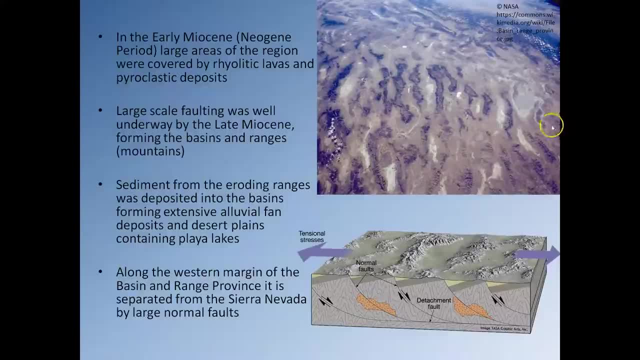 And that actually leads to the formation of the basins and the ranges. So what actually happens? Well, this is what's causing them. So these are big, curved, normal faults. They're called listric faults, And a listric fault doesn't cause. 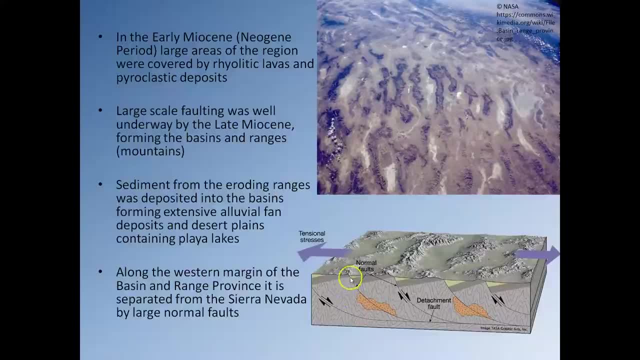 a block of rock to just drop straight down, Because the fault is curved. when this block of rock here drops down, this side of it drops down faster than this side, And so it means essentially this block of rock pivots as it drops. 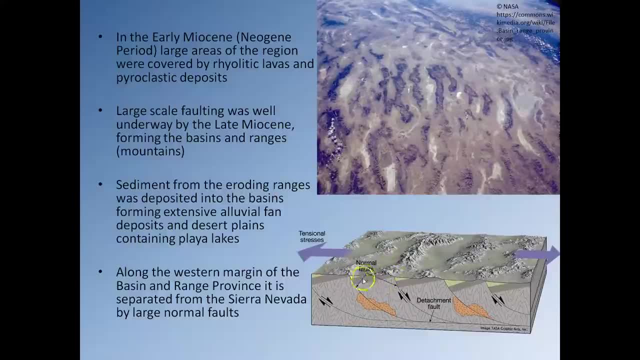 So this side essentially stays up and this end goes down. So as this side drops, you form a depression, a topographic low That becomes your basin, Whilst this portion over here, which remains essentially, comparatively speaking, higher, becomes your range. 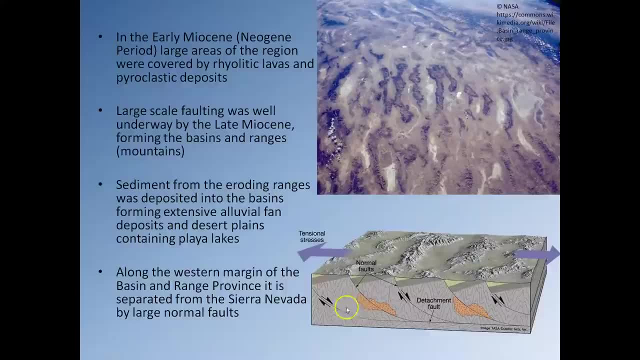 your mountains, your hills. Obviously, the basins in between the ranges are being filled up by material that's being eroded off from the ranges and deposited into the basins, And we see that these areas are, you know, they're desert to semi-desert. 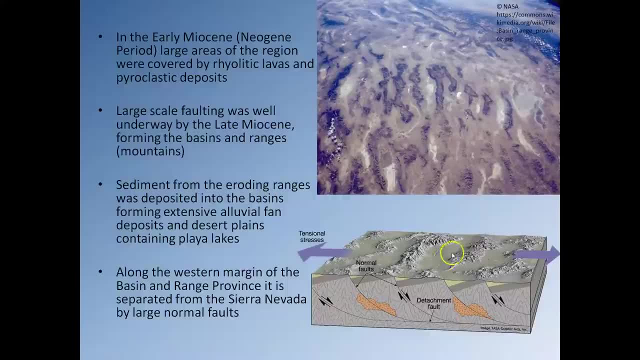 There's lots of alluvial fans, lots of player lakes, lots of- you know- desert environments. in these regions It's very, very dry. So along the western margin of the Basin and Range Province it's separated from the Sierra Nevada. 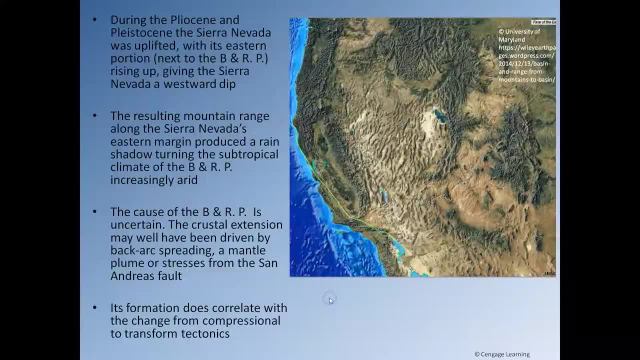 by large normal faults. So OK, so here we go. So this is a shot of the western United States And you can see the Basin and Range Province quite easily. here. You can see all of these ranges orientated approximately north-south. 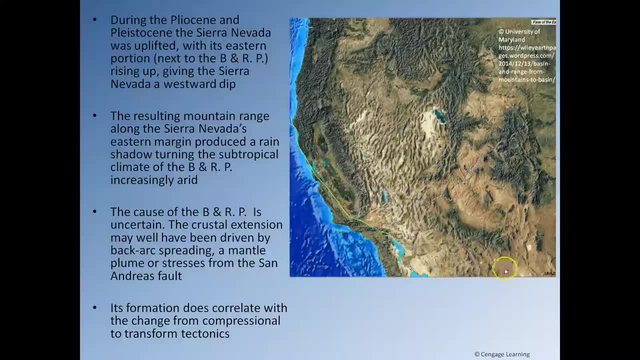 And you can see them carrying on all the way down here, And you can see some of them down here as well. So you know, don't think that it's just limited to this area. It's quite extensive. In fact, you can see one range coming down here there. 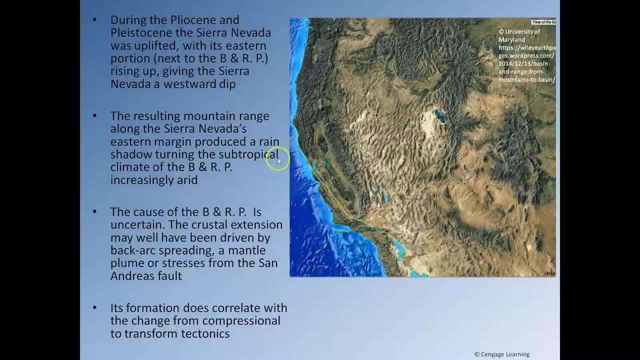 So you know it's a very expansive area. So during the Pliocene and Pleistocene the Sierra Nevada was uplifted, So OK, so there's the Basin and Range Province, And over here we have the Sierra Nevada. 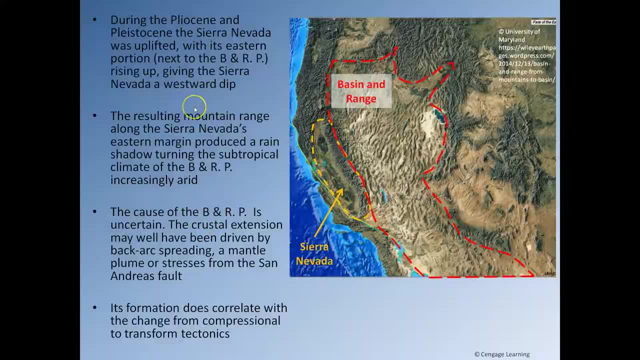 So during the Pliocene and Pleistocene, so relatively recently, the Sierra Nevada was uplifted with its eastern portion. so that's the region along here rising up, And that gives the Sierra Nevada a westward dip. So the Sierra Nevada is tilted. 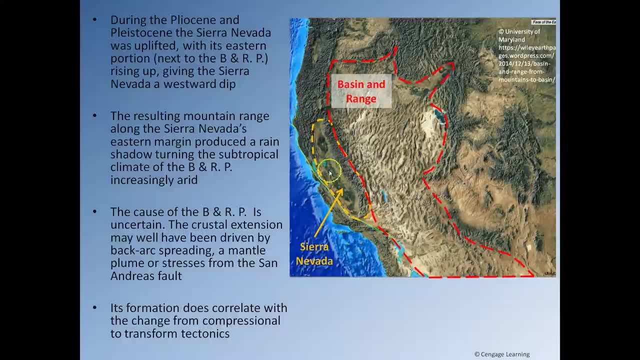 This eastern side here is higher than the western side, And so it means the rocks are all dipping towards the west. It also means, though, on the eastern side of the Sierra Nevada, here you have a set of mountains forming, Because the western side of the Sierra Nevada 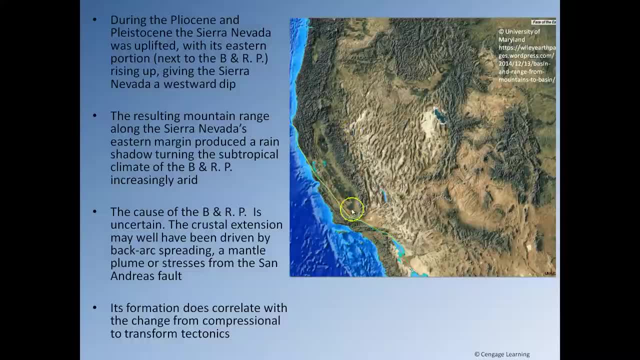 the eastern side gets tilted up, And so that means you form an area of high ground. So this resulting mountain range along the Sierra Nevada's eastern margin produces a rain shadow, So all the wet water that's coming off the Pacific comes in and moves essentially eastwards. 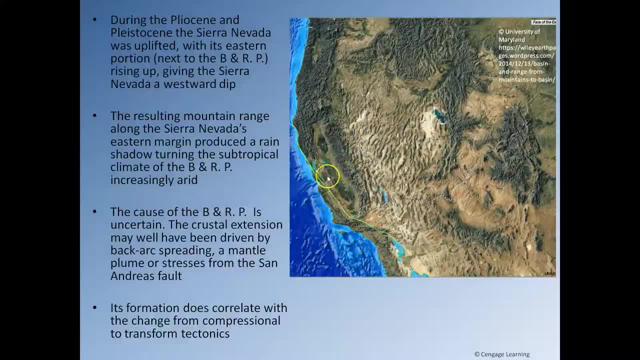 And in order to get over this mountainous terrain here, the moist air has to rise to try and get over it. And as it rises the moist air gets cooler. Then that causes the humidity in the air to begin to condense, to form raindrops. 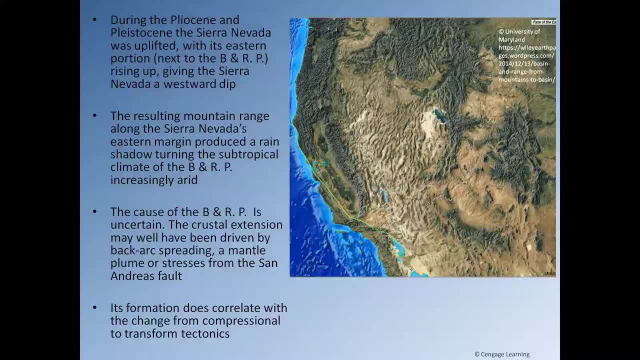 And, of course, that water falls out of the sky in the form of rain or maybe even snow, And so, by the time the water makes it over to the other side of the mountain range, most of the water that was in that body of air. 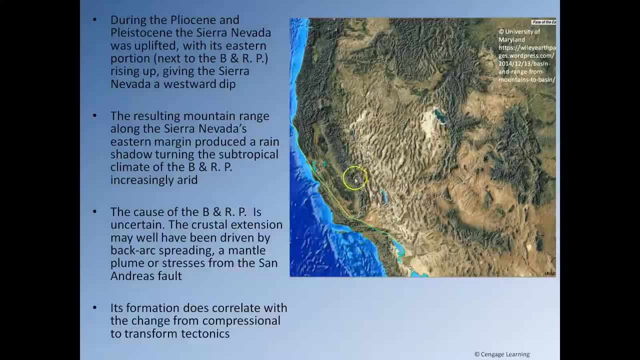 has been lost, And so it's very, very dry air, And so this means that you have a region behind the Sierra Nevada which, essentially, is referred to as a rain shadow. It's a region where the air is very, very dry. 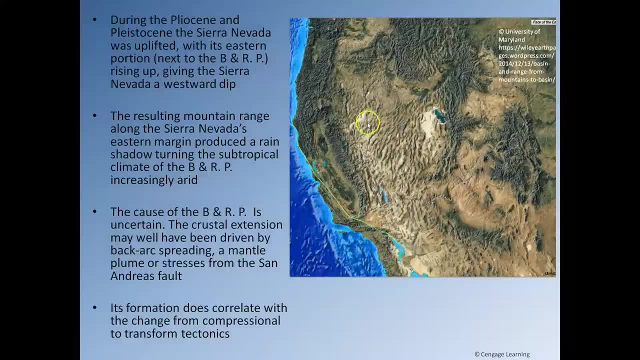 And so that explains why this area, which is the modern-day Basin and Range Province, is associated with very, very dry conditions. I mean, if you've ever been to Nevada, you'll know that it is a very warm on the whole, relatively low humidity place. 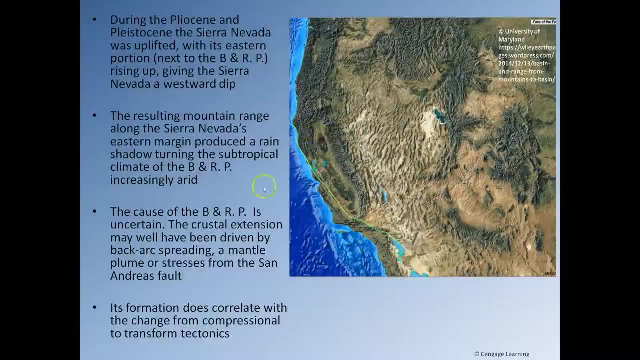 And that's all due to the Sierra Nevada. So the cause of the Basin and Range Province is actually uncertain. It's this huge area and we're not 100% sure why it actually formed. So we know this area is under crustal extension. 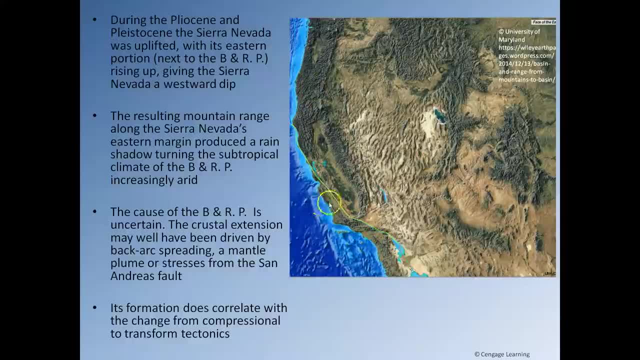 so we know it's being stretched. So this area of crust over here must be going this way and this area of crust over here must be going this way. So we know that, And that's obviously causing the area of crust in between to be extended. 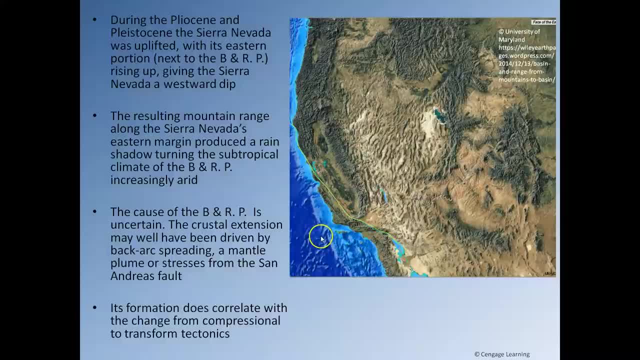 So the question is why? Well, we're not really sure. It could be driven by some kind of back arc spreading, a bit like Japan. However, back arc spreading requires a subduction zone, So the subduction zone is long gone. 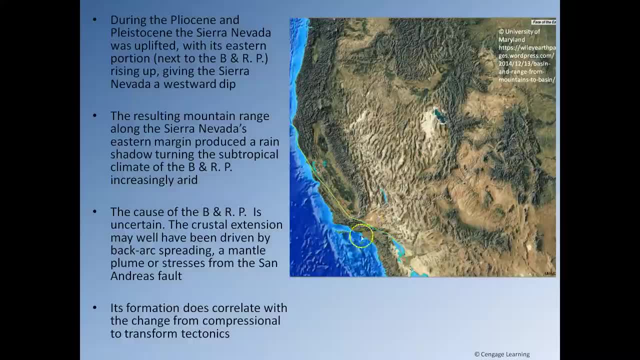 so whether that would be the case is very debatable. Some people have suggested there could be some kind of really large mantle plume underneath this area which is pushing up the crust, causing it to dome, and that makes it extend, That makes the crust get stretched. 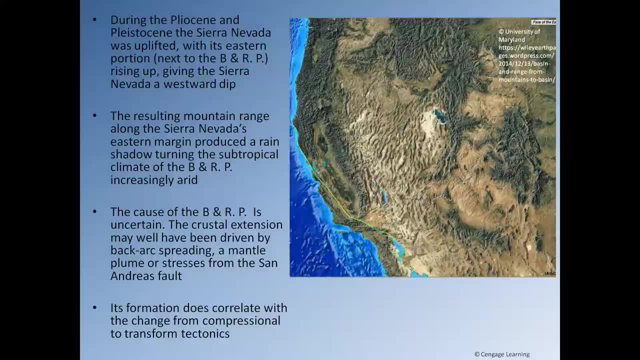 However, once again, there's very little evidence for that. You would expect large volcanic eruptions in the area if that was the case, which we just don't have, So the most likely explanation at the moment is it's due to the San Andreas Fault. 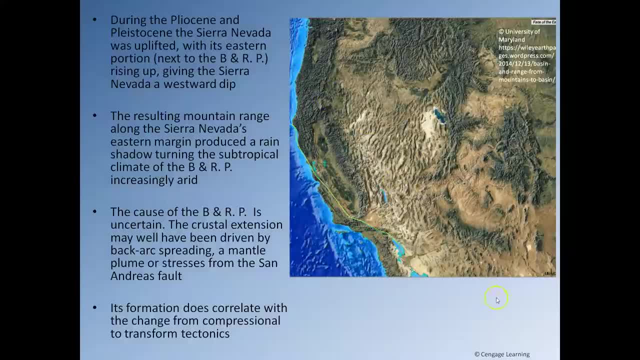 So, as we discussed, this area of crust here is trying to move towards the southeast and this area of crust over here is trying to move off towards the northwest, And so what people think is happening is, as this area of crust here is trying to move southwestwards. 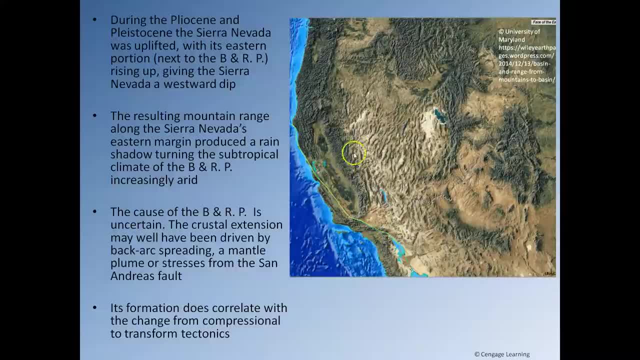 you can see there's a kink here in the San Andreas Fault. So this area of crust here, the Sierra Nevada, is trying to move down towards the southeast, but it can't go straight down. It's got to kind of work its way down here. 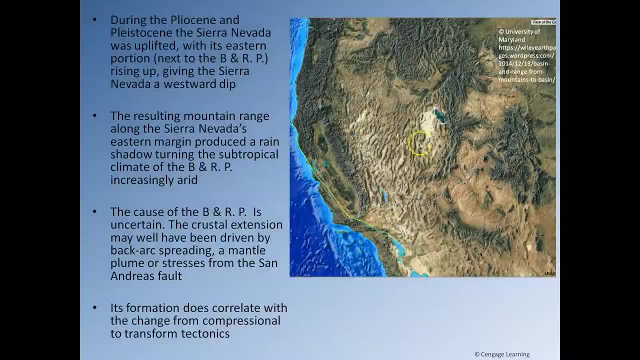 and curve with the fault here, and that means that this area of crust here begins to become stretched as the Sierra Nevada begins to pivot a little bit. So as the Sierra Nevada tries to curve and come around here like this, it puts this area of crust under extension. 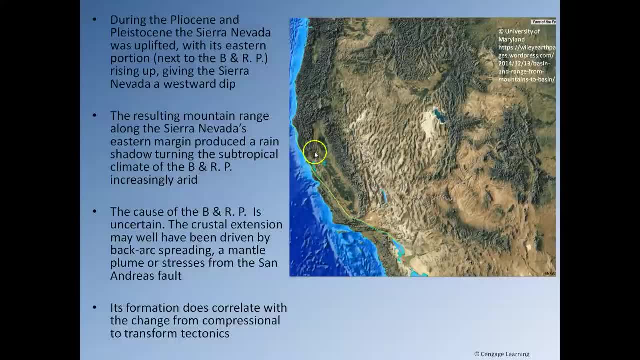 and starts to stretch it. So that seems to be one reasonable indication as to why the Basin and Range Province forms. So its formation does correlate with the change from compressional to transformed tectonics. So around the time when the Sierra Nevada 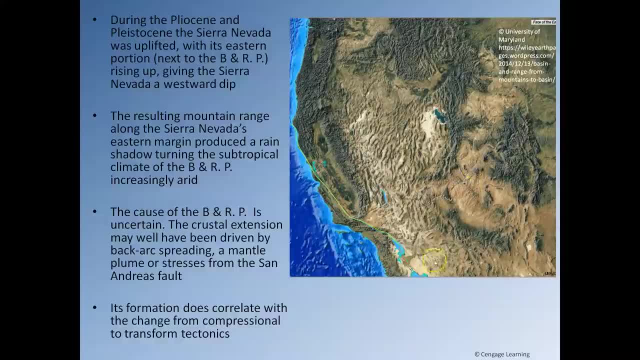 when the San Andreas Fault begins to form, we see the start of the Basin and Range Province formation, And so that also helps to somewhat suggest that the formation of the Basin and Range Province is probably due to the shift to transformed tectonics. 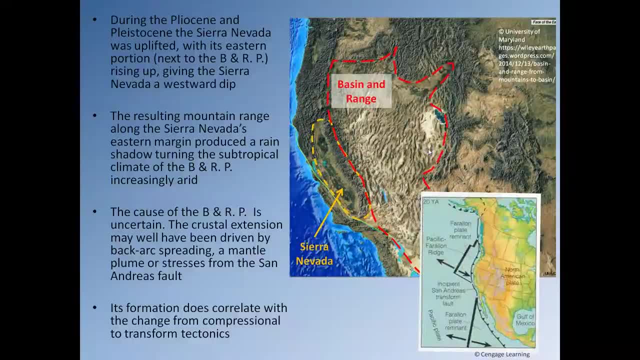 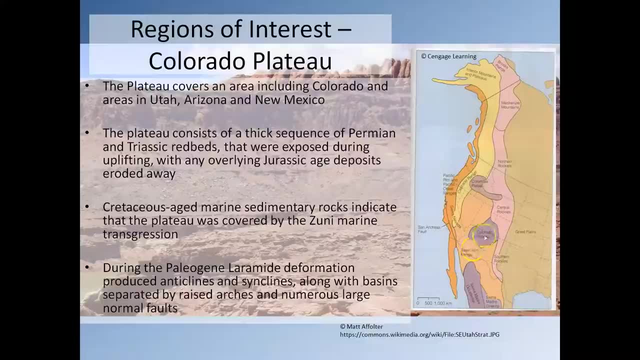 So okay, so that was the Basin and Range Province. Then we have the Colorado Plateau up here, So the Colorado Plateau covers an area that includes Colorado and areas of Utah, Arizona and New Mexico. So the plateau consists of a thick sequence. 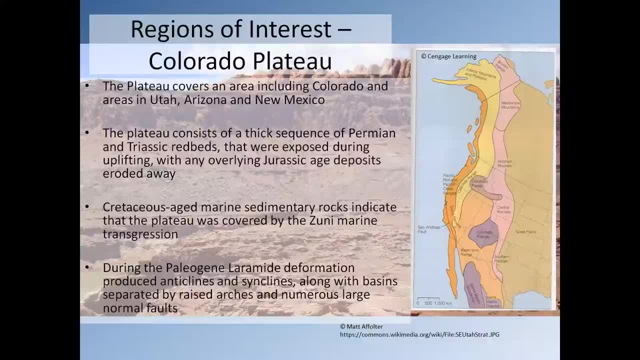 of Permian and Trassic red beds. So this entire sequence was exposed due to uplifting and that meant that the younger settlement on top of these Permian and Trassic beds, the Jurassic rocks, were eroded away. So that occurred during the late Jurassic to early Cretaceous. 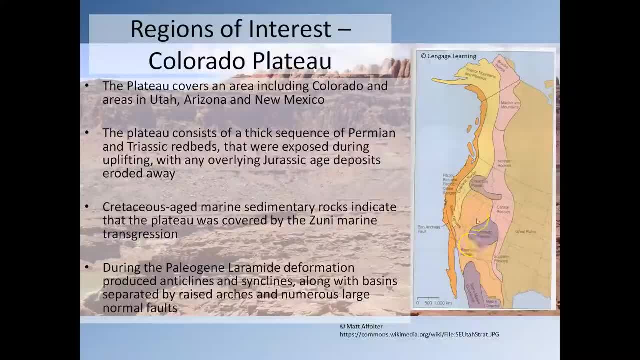 During the Cretaceous, the area that's now the modern-day Columbia Plateau was underwater because, of course, we had the Zuni marine transgression and that caused the formation of the Cretaceous Interior Seaway, So this entire area here was all underwater. 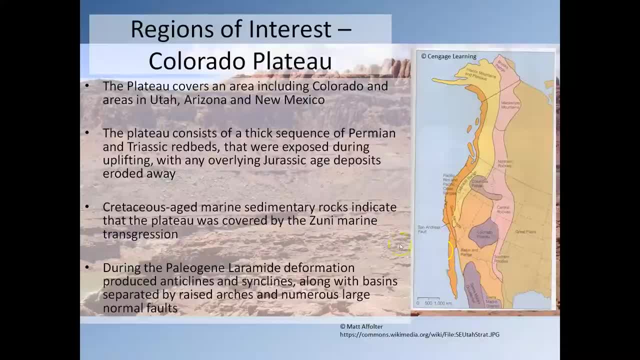 including the Colorado Plateau, And so that meant that during the Cretaceous, the area that is now the modern-day Colorado Plateau was covered by sequences of marine sediments. Then, obviously, as we move from the Cretaceous into the Paleogene, 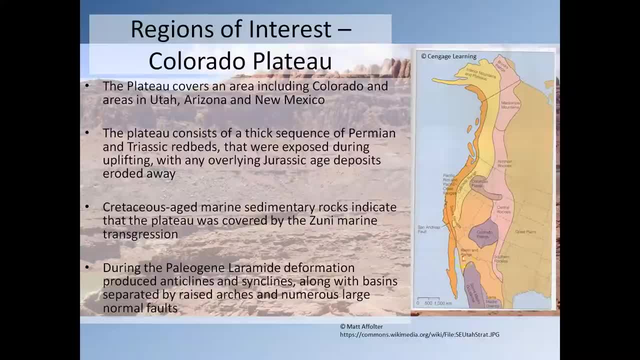 we see the Zuni marine transgression retreating and the Colorado Plateau eventually becomes exposed, and that leads to erosion. It's also deformed during the Laramide Orogeny and that leaves the area being essentially deformed, producing these large, broad, open anticlines and synclines. 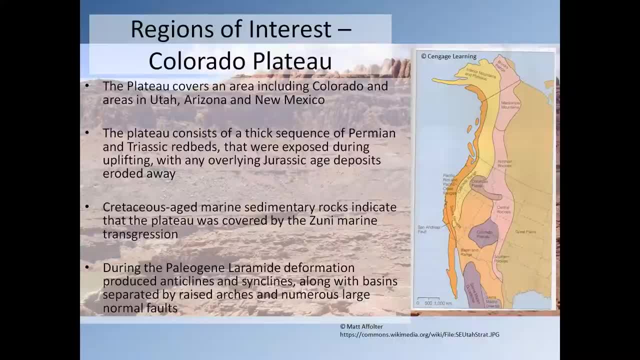 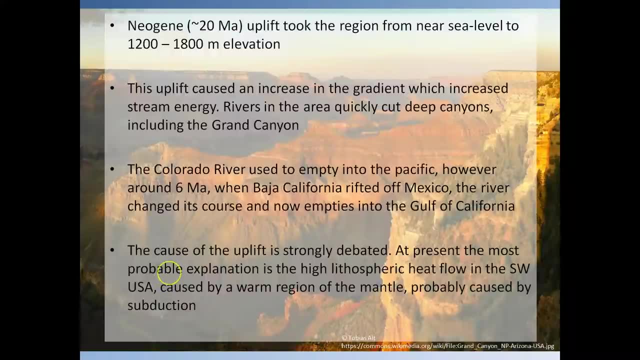 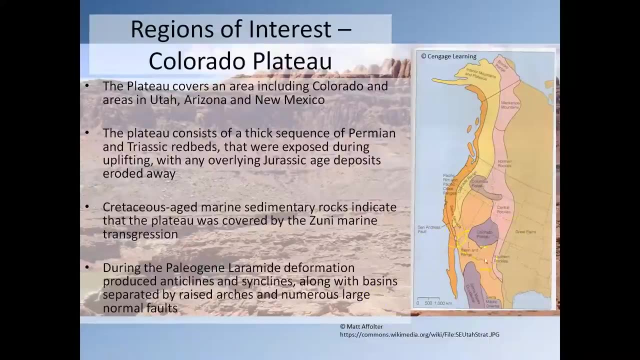 and several large normal faults pushing big blocks of rock straight up. So this entire area was, you know, on the whole relatively unscathed by the Nevadian and Seville orogenies, but it suffered most of its deformation during the Laramide. 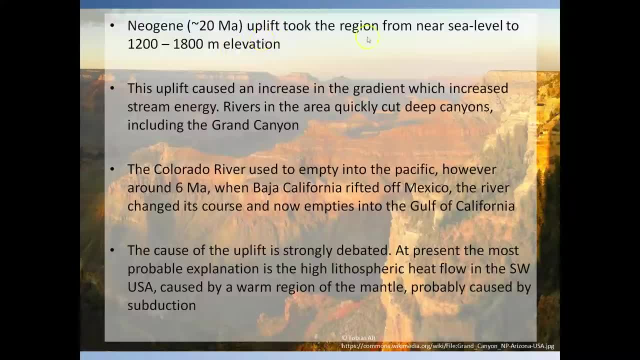 So around 20 million years ago, we see that the area begins to go up. Something happens that begins to make that area rise. So around 20 million years ago it goes from near sea level to around 1,200 to 1,800 meters above sea level. 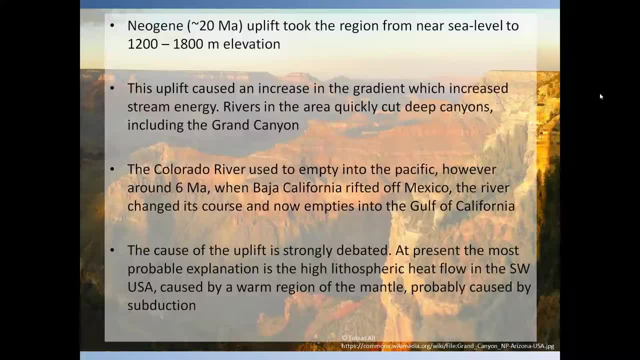 So that's a pretty significant increase. What's causing it? Well, the answer is: we're not really sure. So the uplift actually caused the gradient? Actually, as the ground level goes up, of course that means the rivers that are going through that area. 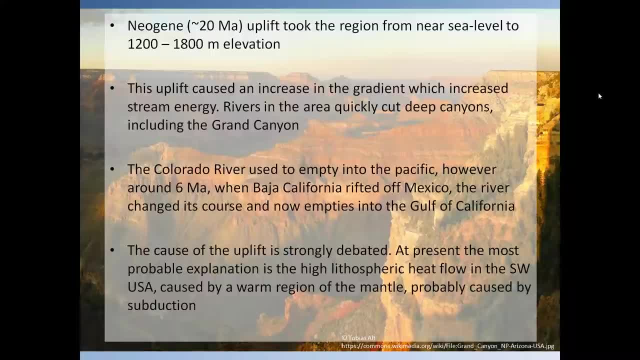 well, they obviously start to drop faster As the gradient gets steeper. the rivers move faster because they're dropping over a steeper gradient, And so this means those rivers have more energy, and so they begin to cut down very, very quickly. 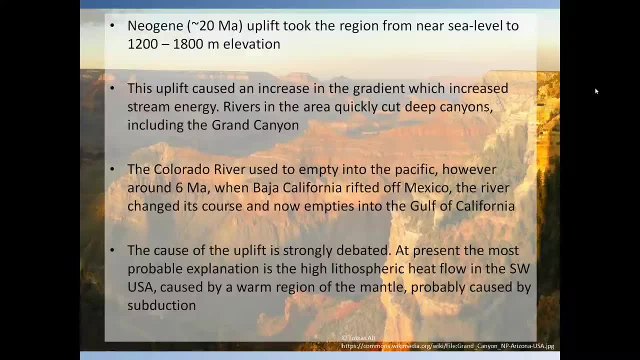 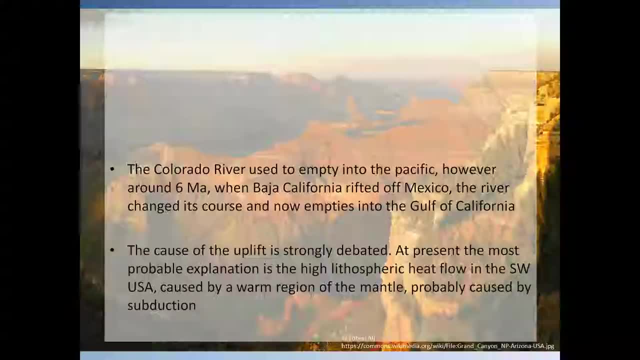 They erode straight down very, very quickly And, of course, this led to the formation of the Grand Canyon. So the Colorado River is the main reason that the Grand Canyon exists and that used to empty into the Pacific, However, around 6 million years ago. 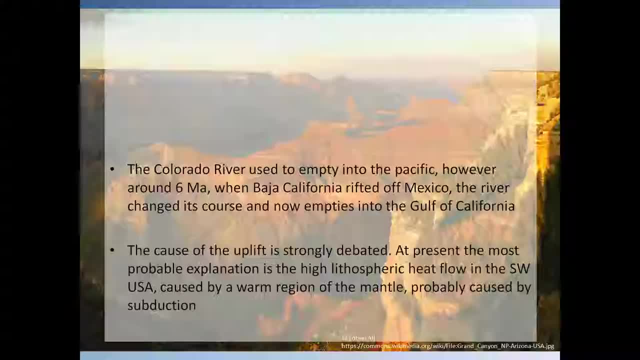 when Baja California began to rift off Mexico, the river actually changed its course and it now empties into the Gulf of California. So this uplift, and the resulting tectonism associated with it, caused the Colorado River to essentially change its course. 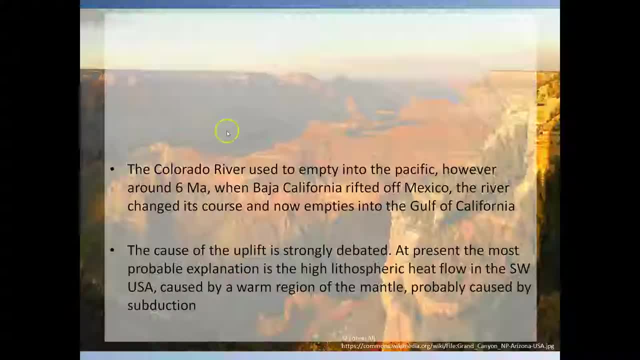 And so that gives us some idea. So around 6 million years ago. it shows that the area had undergone very significant uplift by that point. So the cause of this uplift is very strongly debated. So at present the most probable explanation is that we have what's referred to. 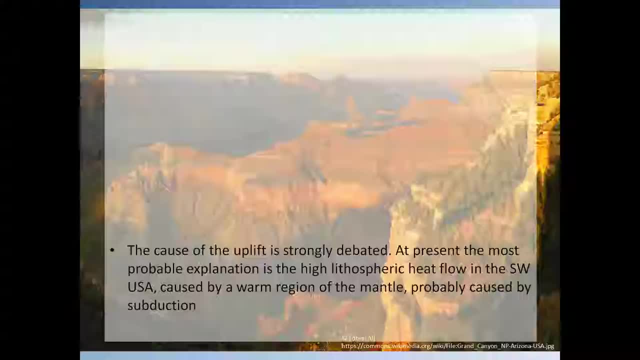 as a high lithospheric heat flow. So this entire area of the United States has continental crust that's rather warm. That means the mantle underneath it is rather hot as well. So this hot mantle underneath it, underneath this area of the southwestern United States, 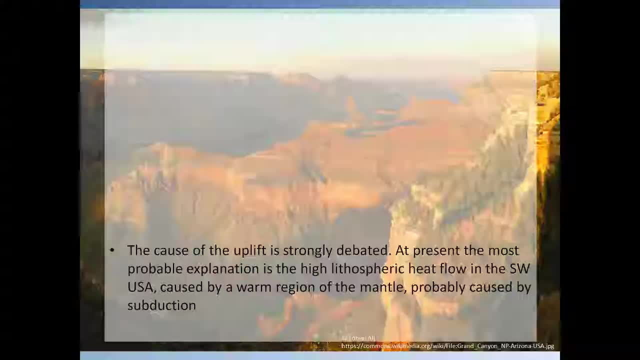 is heating up the continental crust, And, as we've already touched on numerous times before, when rock gets hot, it becomes buoyant and it naturally wants to rise, And so we think that's probably what's going on. This area of crust is rather warm. 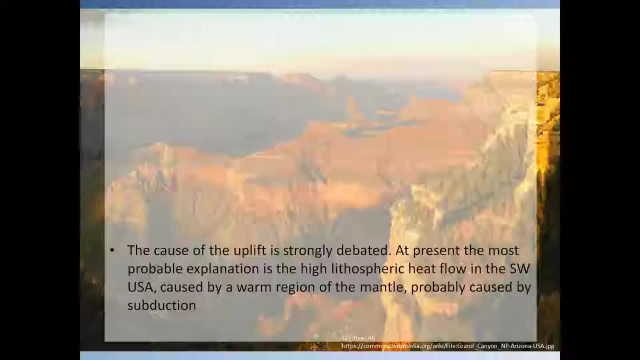 and so it's just naturally rising up. Now, what's causing that warm region of mantle underneath the southwestern United States? that's a bit of a mystery. We're really not sure what's going on there, But as far as we can tell, 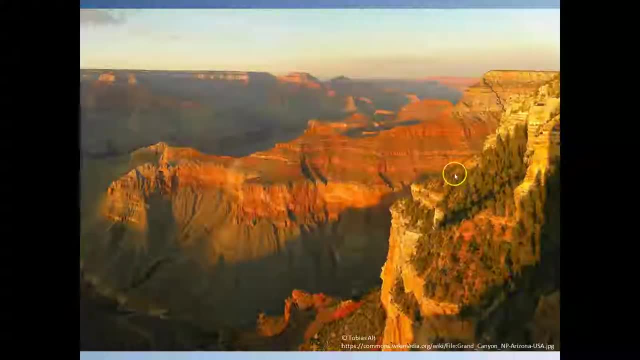 the fact that the crust in this area is surprisingly warm and therefore buoyant. that's what's driving this upward movement, And as the land gets pushed up, it causes the rivers to erode down relatively quickly, and that leads to the formation of course. 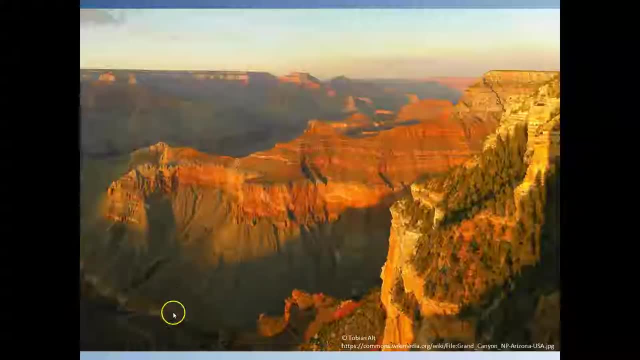 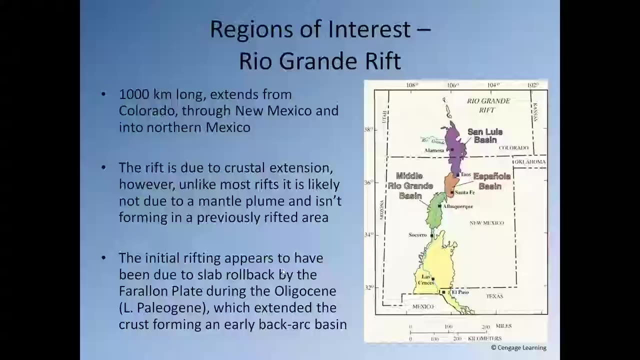 of the Grand Canyon. You can see the huge quantity of material that's been eroded through in the last 20 million years. give or take a little bit, OK. so we've been going for 20 minutes, so once again pause the presentation. 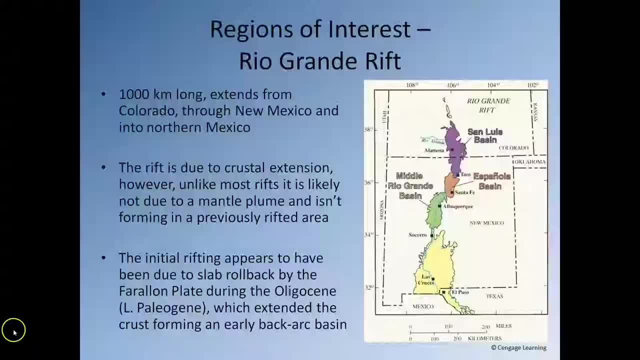 get up, have a walk around and come back in a few minutes, please. So, as discussed, the Basin and Range Province is an area of the western United States that's currently undergoing extension. There is also another region that's currently undergoing extension. 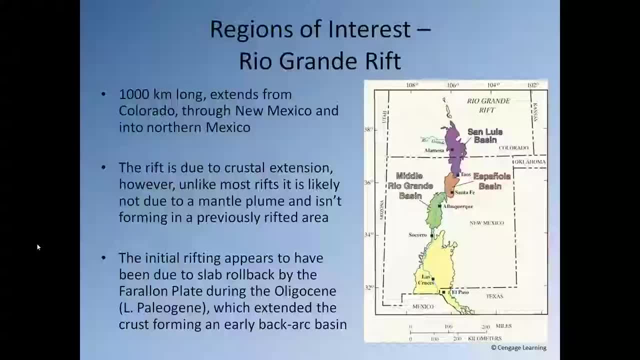 and that's the Rio Grande Rift. So the Rio Grande Rift is around 1,000 kilometres long and it extends from Colorado down through New Mexico into Texas and then into northern Mexico. So the rift is due to crustal extension. so the crust in this area here is being stretched. 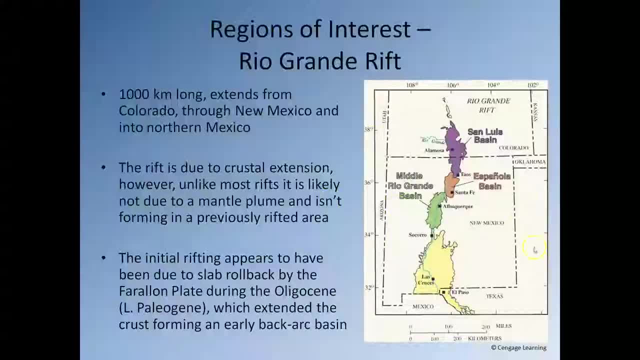 This piece of crust over here is going westwards. this piece of crust over here is trying to go eastwards, and that means the rocks in between are undergoing extension, they're being stretched. So the question is: is why? Why are the rocks here being stretched? 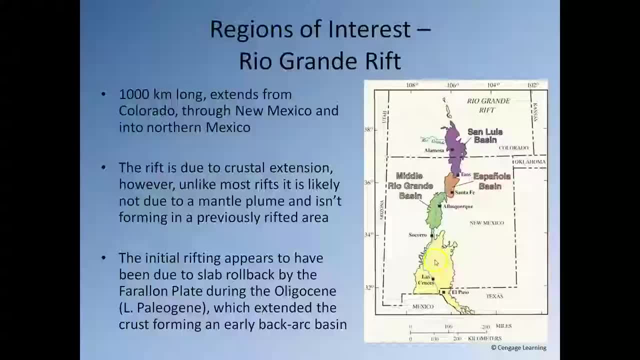 Well, we know it isn't likely due to a mantle plume, because essentially it's an area that isn't formed. Sorry, let's try that sentence again, I've got myself confused there. So the rift is due to crustal extension. 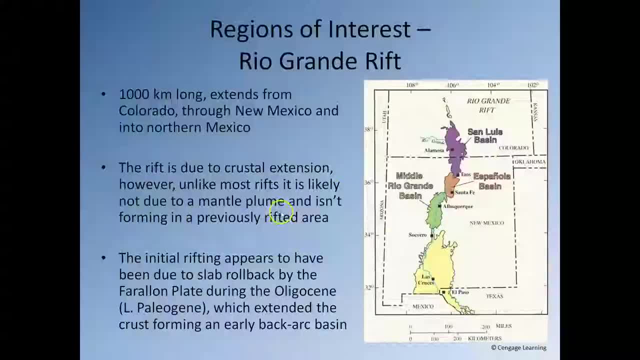 however, unlike most rifts, it's likely not due to a mantle plume, So we have no evidence here to suggest there's a big mantle plume under the ground that's stretching the crust, making it undergo extension. And another interesting fact is: 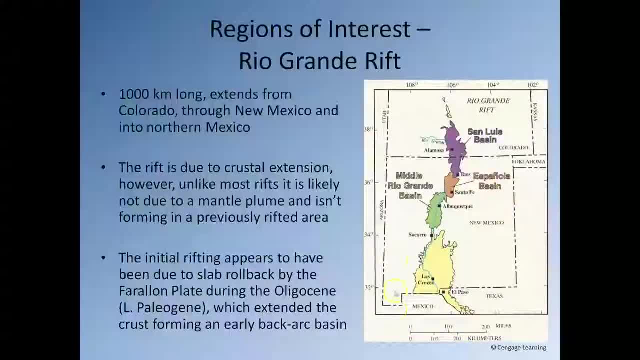 this area is not a previously rifted area. There's no pre-existing weakness here that could explain why this area is rifting. If there's a weakness there, then that's a point of weakness along which the crust could split relatively easily, But this area hadn't undergone any significant deformation. 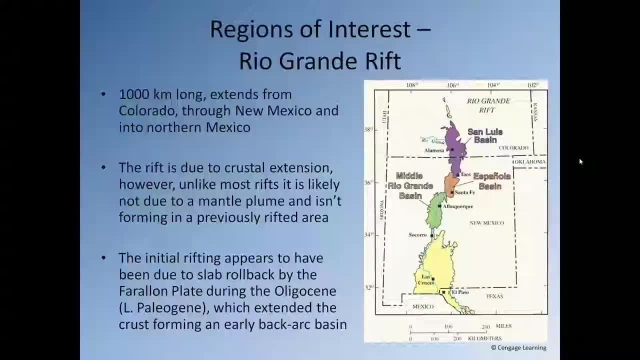 since about 252 million years ago, So not much happening there. So the initial rifting appears to have been due to a slab rollback by the farallon plate during the oligocene. So it would seem that some of the initial extension in this area was due to farallon subduction. 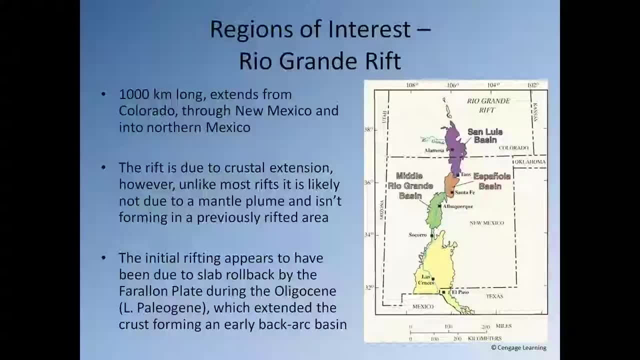 as part of the later stages of the cordillera neurogeny, And that caused this area of crust to begin to be extended and stretched, just like the opening up of the Sea of Japan that we discussed earlier in the presentation. So that was the first stage of rifting. 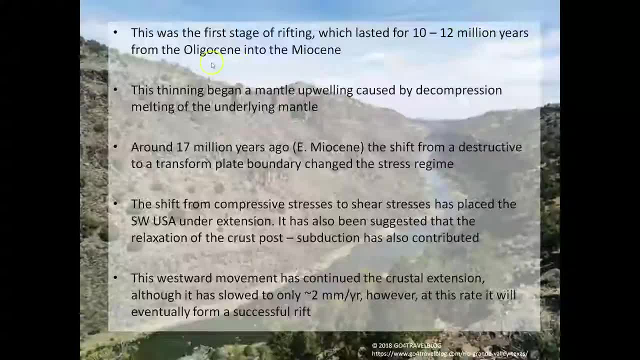 and that lasted for around 12 million years, from the oligocene into the Miocene. So this thinning began a mantle upwelling caused by decompression, melting of the underlying mantle. So the area underneath the Rio Grande started to get very, very hot. 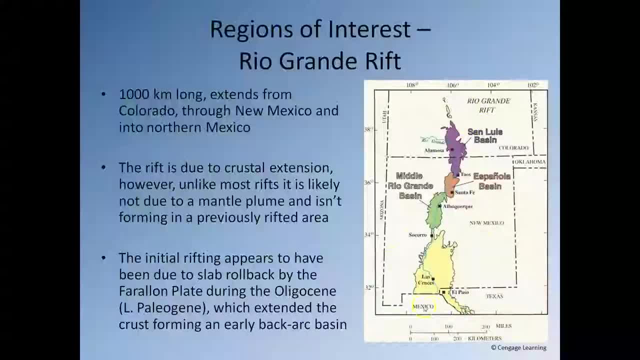 So as this crust here began to thin, the mantle underneath it was under less and less pressure, and so that meant it began to partially melt. That meant the mantle in that region became very hot and very buoyant, and so it wants to start rising. 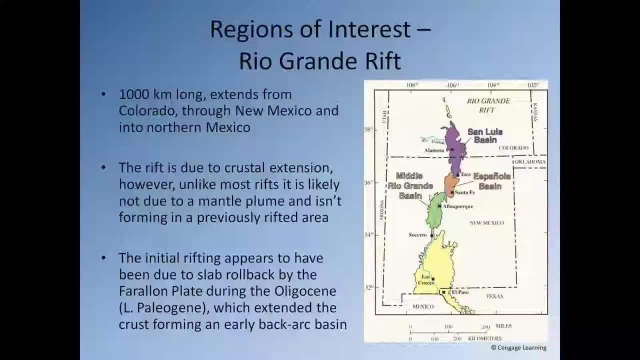 And because it wants to start rising. it's just like taking a sheet of silly putty and pushing your hand into it. If you take a piece of something flexible, like rubber or something, and you push it with your hand, the rubber begins to stretch and deform. 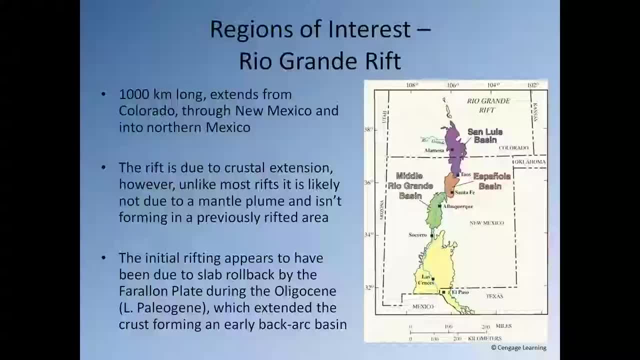 And eventually, if you were to push that rubber hard enough and keep going and going and going, eventually you would push the rubber too far and it would split. And that's essentially what we've got going on here, Because the crust is being pushed up. 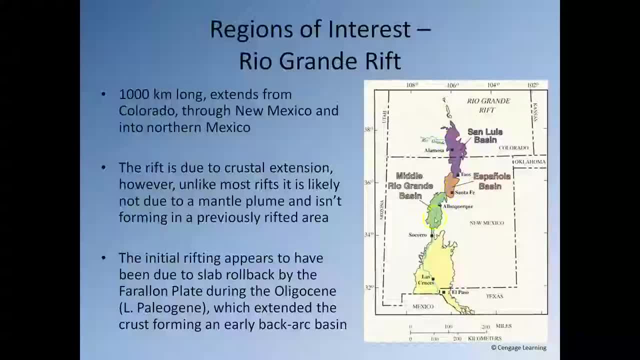 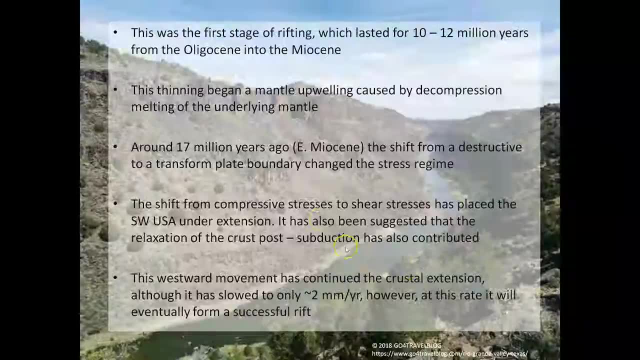 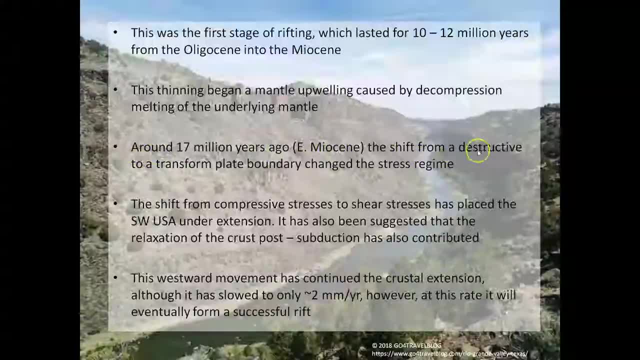 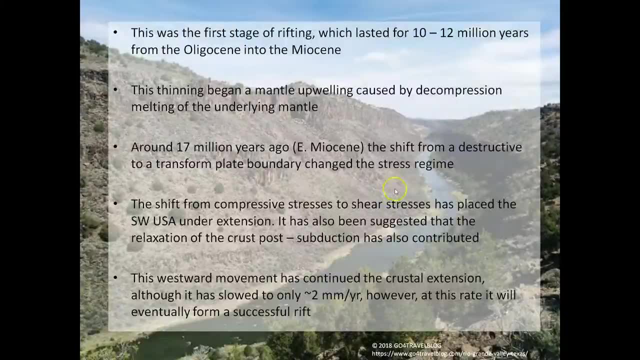 that's the early Miocene. we see a shift from a destructive to a convergent plate boundary, to a transformed plate boundary And of course this has a very significant effect because it changes the stress regime. So this shift from compressive stress, 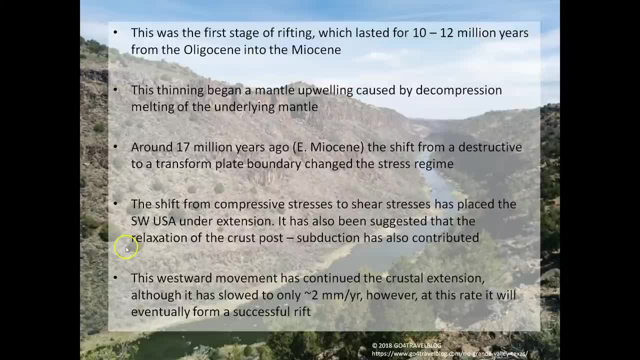 to shear stresses has placed the southwestern United States under extension, as we've already discussed. So this shift from a convergent plate boundary to a transformed plate boundary means that the entire southwestern United States begins to become stretched and warped. it's sheared. 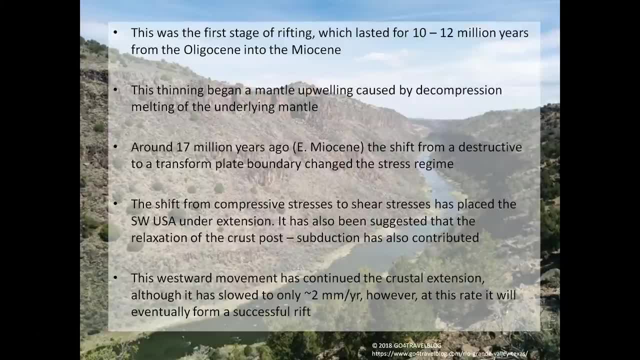 as essentially, the United States is trying to move southeastwards, whilst the eastern side of the western side- sorry, of California and the Pacific Plate- is trying to go northwest And that's causing this entire area to be stretched. There's also another factor involved here. 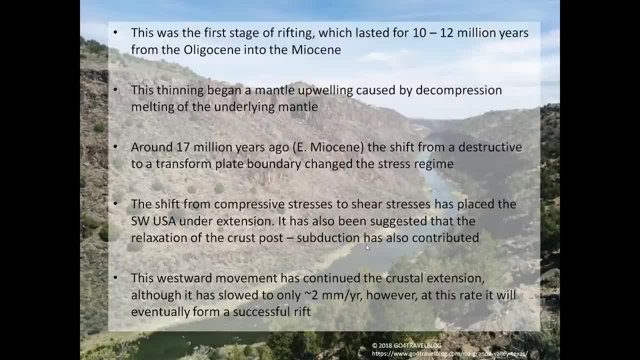 which is that, as the area had undergone some compressional forces due to the Cordillera and Orogeny. well, once that Orogeny stopped and the compressive forces disappeared, well, it meant the crust that had been for a long period of time under pressure. 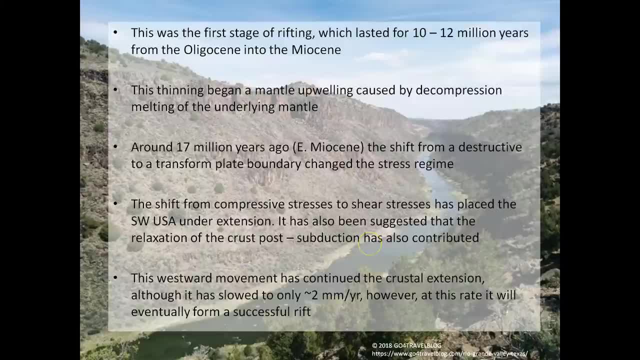 under compressional forces all of a sudden could undergo extension, it could stretch, And so, obviously, when that crust begins to stretch, what does it do? Well, obviously that leads to extension and that will also contribute to the formation of the Rift Valley. 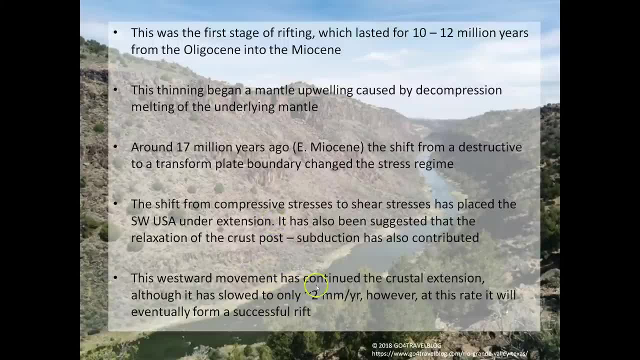 So the westward movement has continued and crustal extension, although it's slowed, it's still going at around 2 mm a year. That's still fast enough to allow this valley to keep getting bigger and bigger and bigger. and in theory, if crustal extension continues, 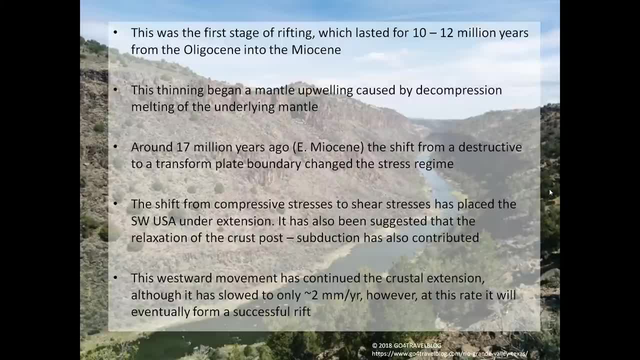 it could form a proper rift, and the western side of the United States could begin to rift off from the eastern portion of the United States, And so you can actually see the Rift Valley here. So here is the Rio Grande Valley. You can actually see it's a Rift Valley. 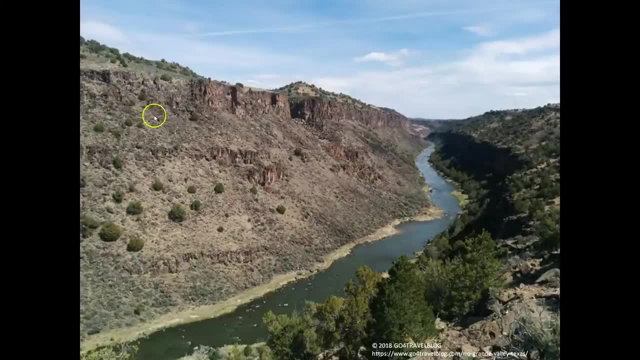 It's quite a nice example. You can see we have a fault here, There's the fault scarp there. So that's one step. Then we have another fault block. Here's another fault scarp- A second step. Then we have another fault block here. 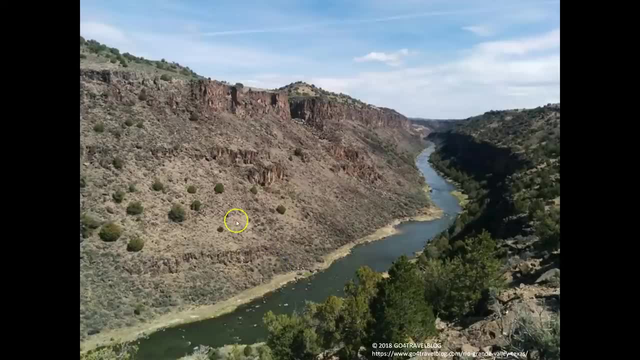 Another step. Then we have another fault block down here, Another step. So the crust is going: one fault, two faults, three faults, four faults, And so we have these normal faults where these blocks of rock are dropping down relative to one another. 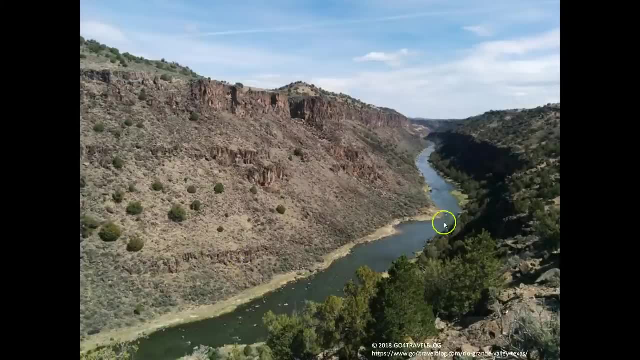 Classic Rift Valley, tectonics And obviously the Rio Grande River is going to take the path of least resistance. If there's a nice valley that's already been made by this rifting, the Rio Grande River is going to simply follow it. 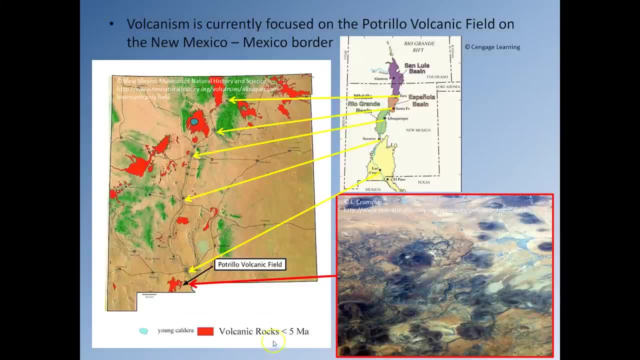 So when we look at the Rio Grande Rift, so this is a map here that shows you volcanic activity in the last five million years And you're going to see that it is pretty extensive. So this entire area here is undergoing extension And that's allowing the crust essentially to fault. 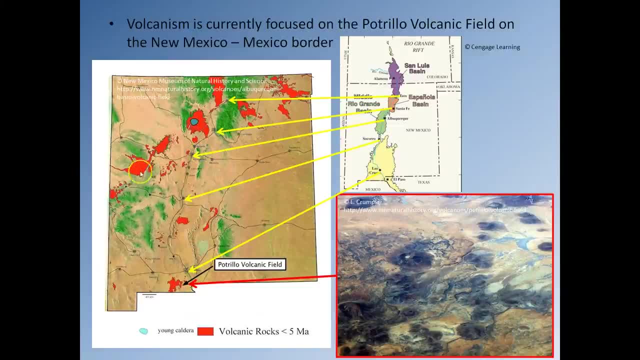 producing pathways along which magma can rise And we can see all this red stuff. here are relatively recent blocks, It's relatively recent volcanic activity. So, for instance, there are active volcanoes around Albuquerque And there are active volcanoes down here around the New Mexico-Texas border. 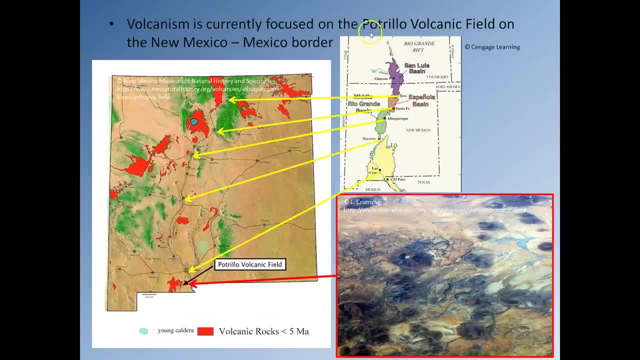 And the most active area at the moment is the Potrillo volcanic field. That's on the New Mexico-Mexico border And here's an aerial photograph of it. So all of these black circles here are active volcanoes. So this entire area here. 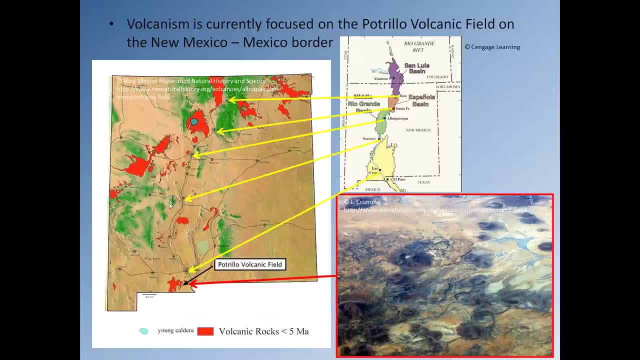 is volcanically active Because the crust is becoming so thin, the mantle underneath it is beginning to melt. That's producing magma which is going to feed volcanoes on the surface. Now we're not at the point where the rift is so advanced. 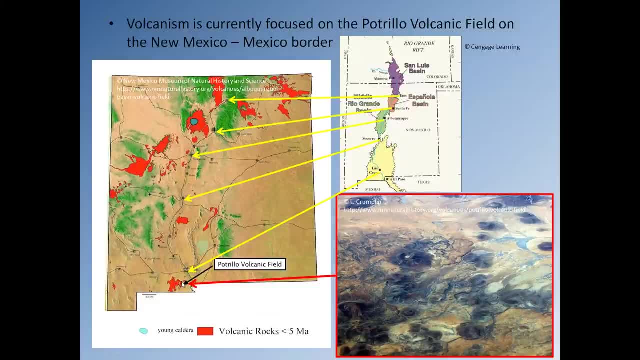 that it's going to form large quantities of basalt, which would give us oceanic crust. So we're nowhere near the western side of North America, rifting off from the eastern side, But the possibility is there. So, OK, so that was the western side of the United States. 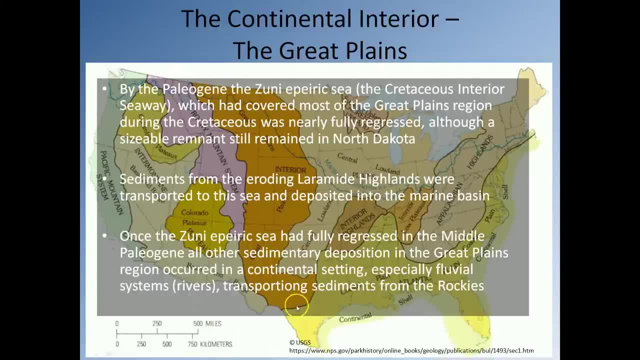 So what's happening in the middle, What's happening in this orange area here, the Great Plains Well, by the Paleogene, the Zoonoepiric Sea. so that's the Cretaceous interior seaway which had covered this Great Plains region. 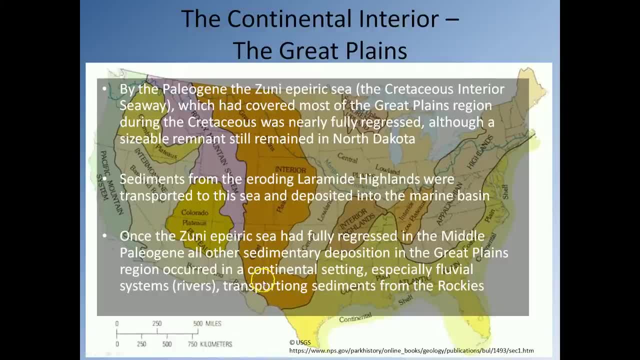 during the Cretaceous had nearly fully regressed, Although there was a small area of the Zoonoepiric Sea which got trapped and it got destroyed, you know, got isolated, and that was located here. sorry, up here, sorry. 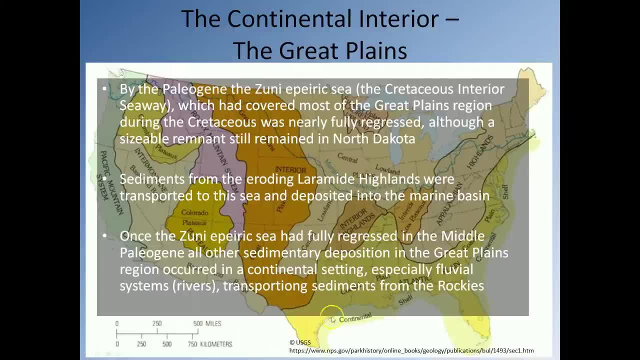 in North Dakota. So this area was underwater during the Cretaceous. By the time we're into the Cenozoic, going into the Paleogene, this body of water's retreating southwards into the Gulf of Mexico and northwards towards the Arctic Ocean. 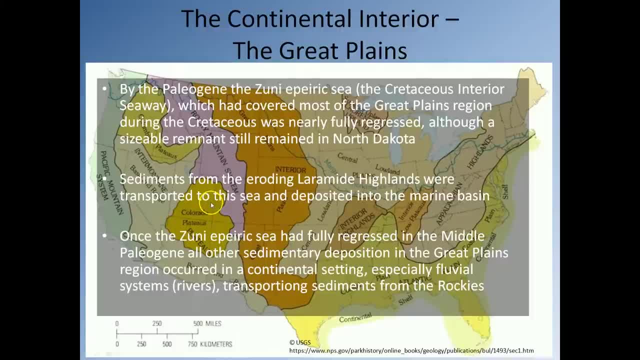 And that means this area is going from a marine environment into a continental environment. So sediments from the eroding Laramide Highlands up here were transported into the sea when it was there and deposited into the marine basin. Now, once the marine basin's gone, 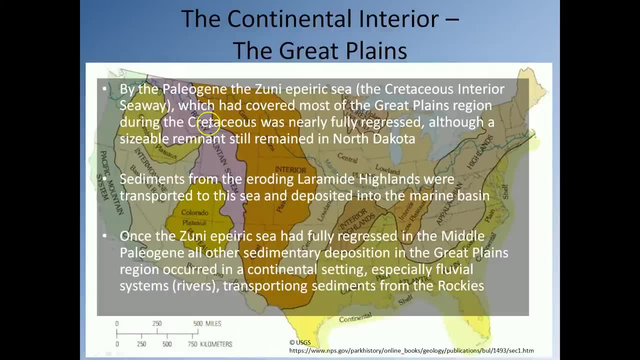 what happens? Well, exactly the same thing. So, from the Paleogene onwards, although the body of water's gone, we still have large quantities of erosion from the Rockies over here. That's producing huge quantities of sediment that's being transported by very, very large rivers. 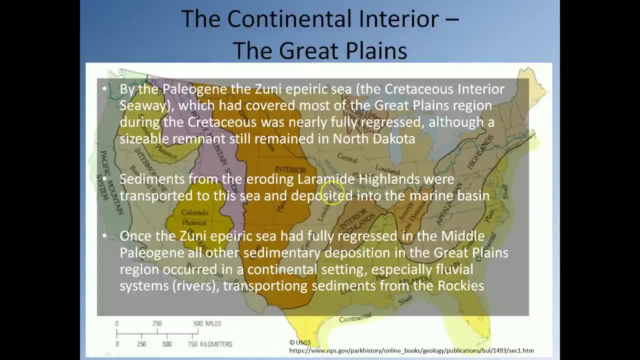 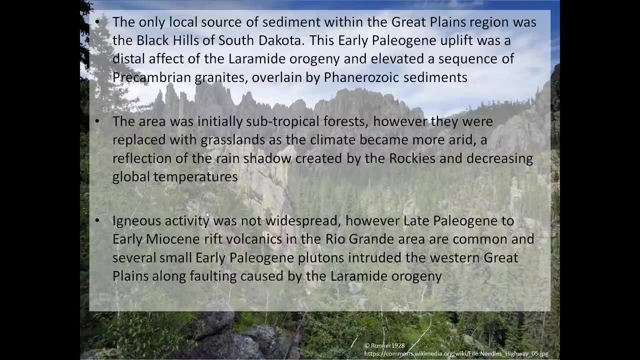 like the Missouri and the Mississippi across the Great Plains region. So this entire area here is now dominated by these very, very large fluvial systems. The only local area of sediment within the Great Plains region is the Black Hills of South Dakota, which you might know if you've ever been on a field trip. 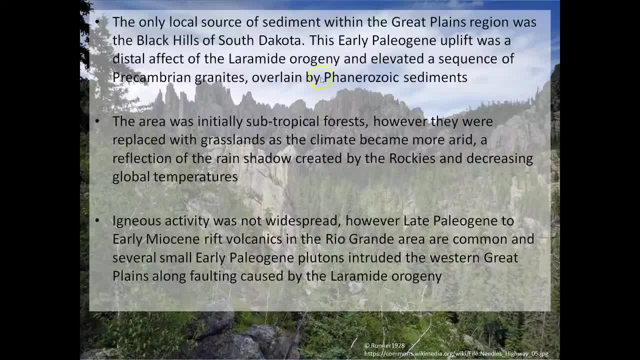 to go to Mount Rushmore. So this early Paleogene uplift was a distal effect of the Laramide Orogeny. So this area was pushed up by the Laramide Orogeny. It was a very, very, very, very distal effect. 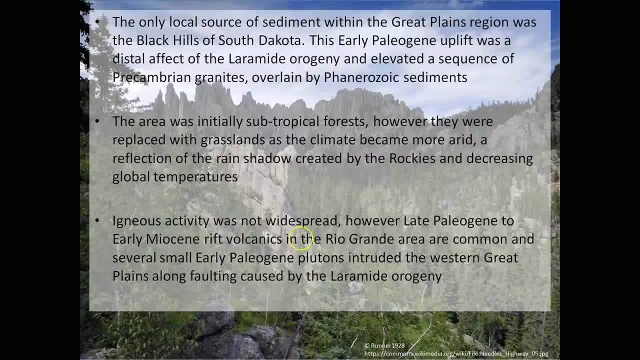 So it was right on the edge of the Laramide Orogeny. The Laramide Orogeny caused this area of granite to be pushed upwards. And so what happened? because the granite got pushed upwards, all the sediment on top of it got eroded away. 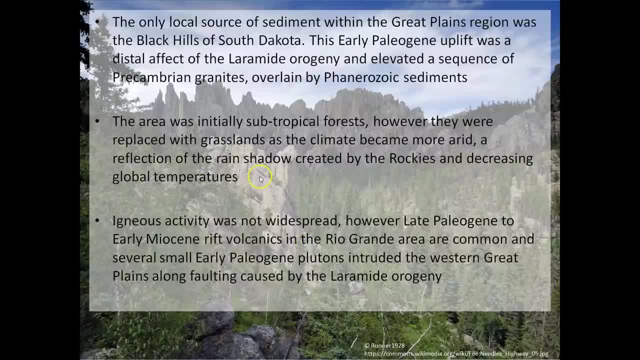 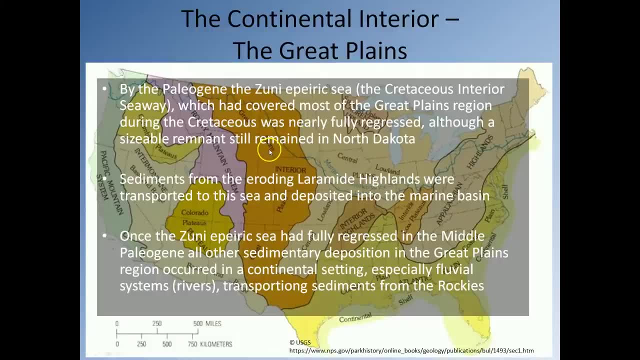 and the granites eventually became exposed. So you can just see it right here. So here's South Dakota. So this is right on the extreme edge of the Laramide Orogeny, But even so, the Laramide Orogeny still managed. 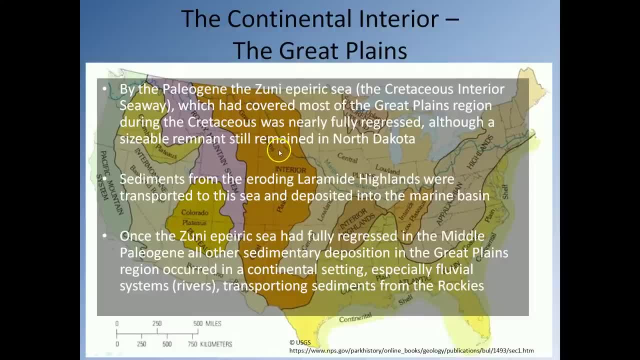 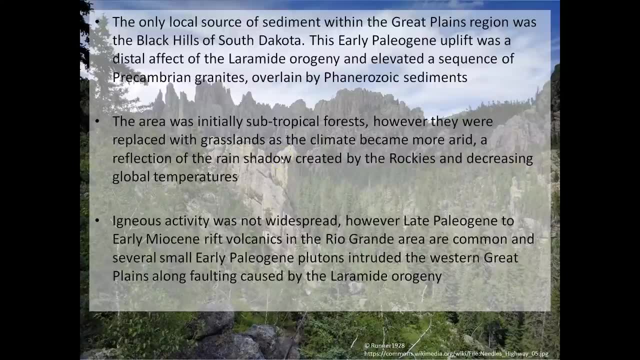 to cause a big block of granite to be pushed straight upwards due to deformation, So the area was initially subtropical forests. However, as you remember, in the early Cenozoic the climate was a lot warmer, a lot wetter, And so the Great Plains region would have been 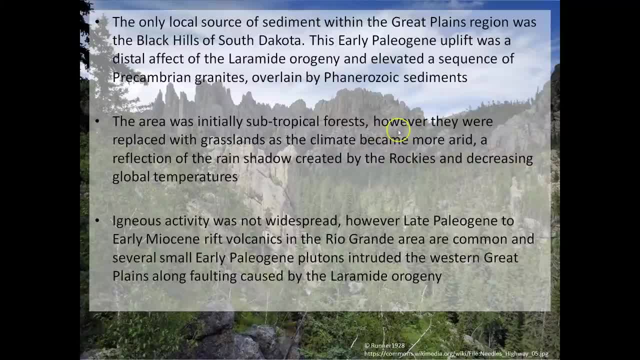 you know, let's say subtropical. However, these subtropical rainforests were replaced by grasslands as the climate became more arid And essentially that's also a reflection of the rain shadow that's produced by the Rockies and also, to some degree, by the Sierra Nevada. 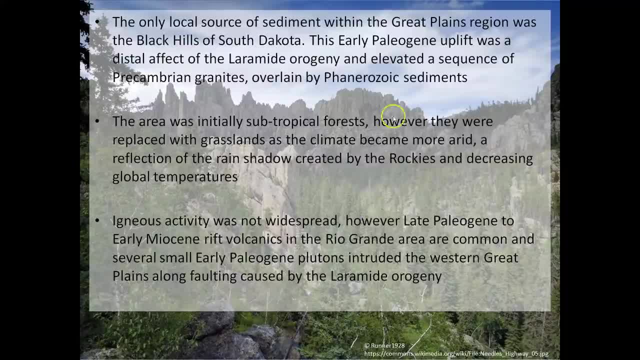 And of course we also have the decrease in global temperatures. So as the Rockies get bigger, that means less rainfall arrives, And as the global climate begins to cool down, that also means the area has lower rainfall. It becomes a lot drier. 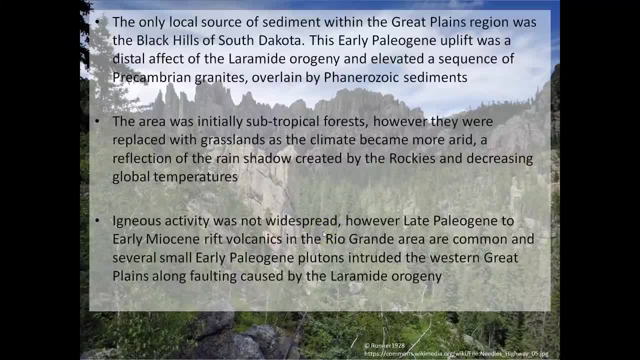 So igneous activity within this region was not widespread at all. There were very few sources of volcanic magma in this area at that time. However, there are late paleogene and early Miocene rift volcanics in the Rio Grande area, which we just discussed. 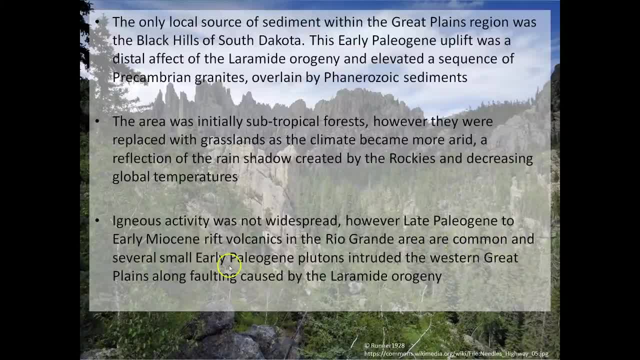 And there are also several small early paleogene plutons- intruded the western Great Plains along the fault caused by the Laramide Orogeny, So the only volcanic activity in this area due to the Rio Grande rifting and plutonic igneous rocks. 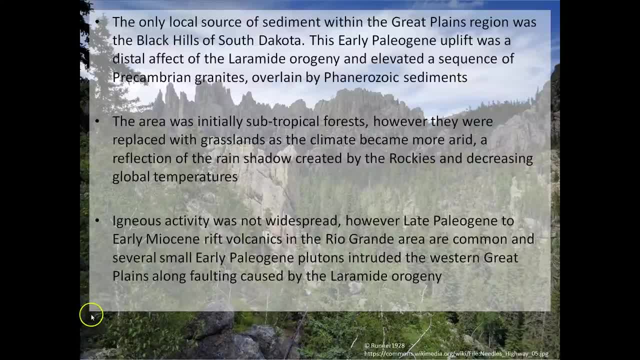 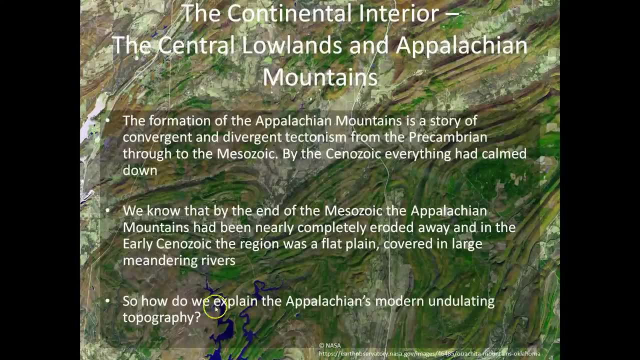 so magmas exploiting large faults along the western margin of the Great Plains. those large faults were produced by the Laramide Orogeny. So what's happening in the continental interior and the continental lowlands, in the Appalachian Mountains. So what's happening? 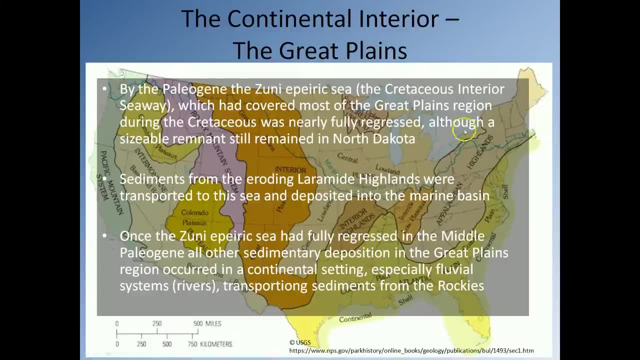 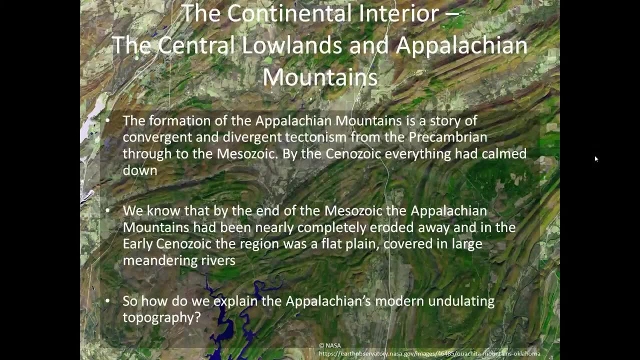 as we go back up here. what's happening over here in the central and eastern portion of North America? Well, the formation of the Appalachian Mountains is a story of convergent and divergent tectonism, from the Precambrian all the way. 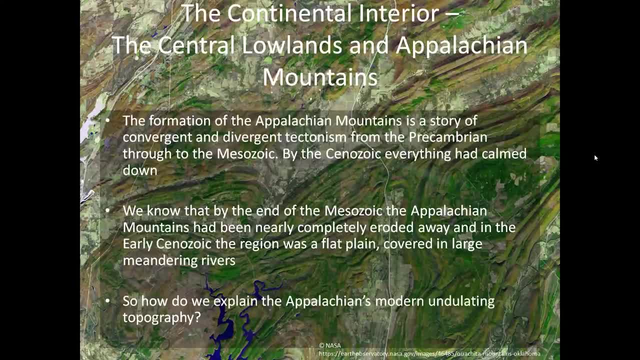 through to the Mesozoic. So, if you guys remember, during the Paleozoic we had the Taconic, Acadian, Acheatan and the Gahenian Orogenies. That all leads to the formation of the Appalachian Mountains. 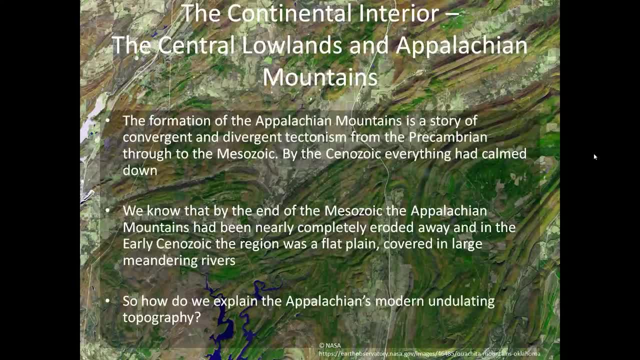 And as we move into the Mesozoic, in the Triassic, we have the area undergoing extension, the formation of a large rift valley that obviously eventually went to go and form the North Atlantic. So we have initially convergent tectonics changing into divergent tectonics. 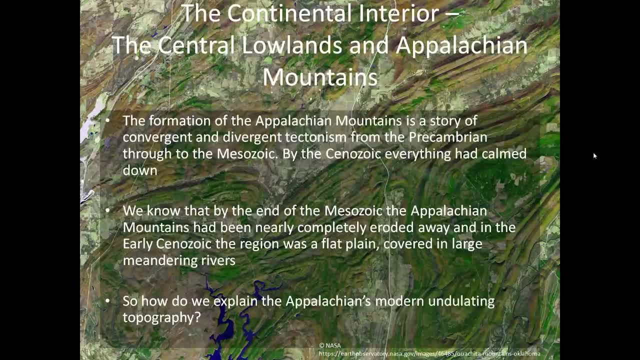 So we know that by the end of the Mesozoic the Appalachian Mountains had been more or less completely eroded away. So by the end of the Mesozoic the area was essentially a flat floodplain. There was no terrain there whatsoever. 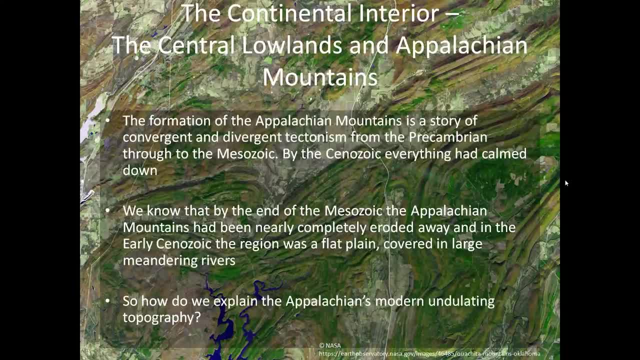 It would have been like the area around Houston, very, very flat. In the early Cenozoic, however, the region was a flat floodplain covered by large mountain rivers. The problem is, if you look at the Appalachians now, 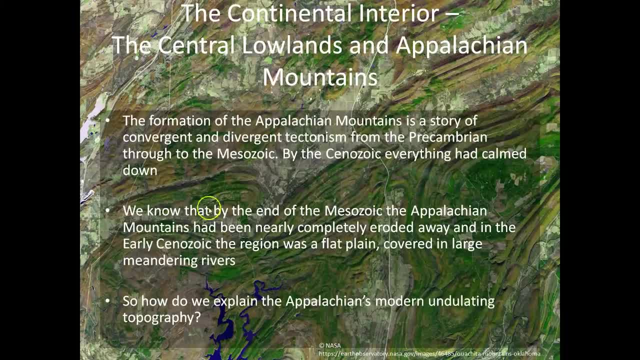 and we can look at the Appalachians. there's a picture behind what we see is we see the area is absolutely covered with masses of terrain, Hills and valleys everywhere. So the question becomes: what happened between the end of the Mesozoic? 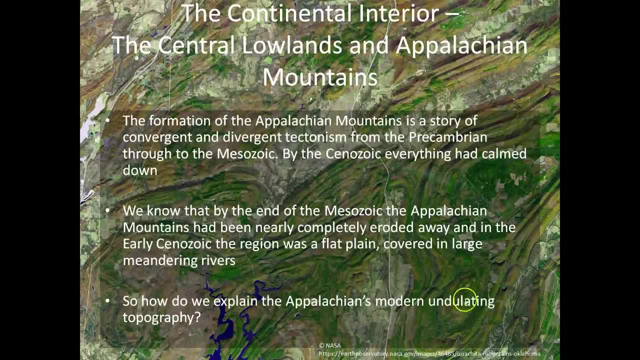 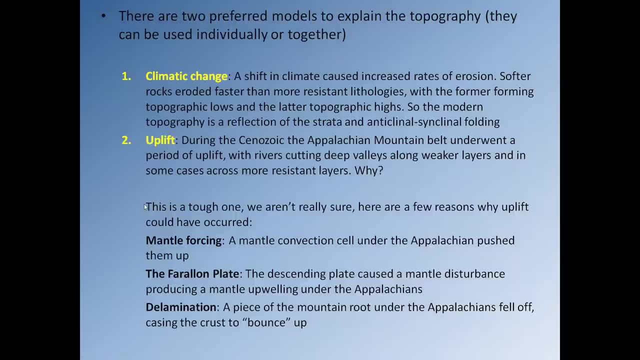 and now Because we have to try and explain why we have all this topography. So there are two preferred models to explain the topography that we see, And you can use them individually or you can combine them together. So the first one is simple. 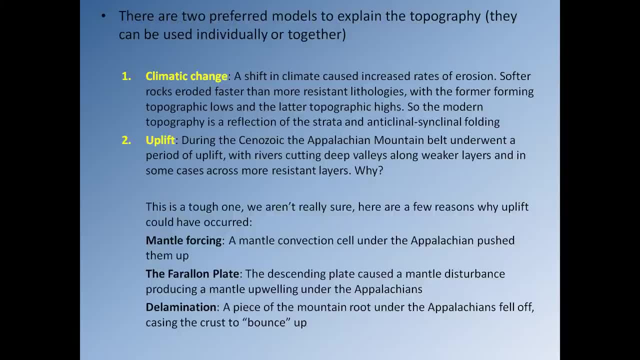 It's a climatic change, So we see a shift in climate causes, increases erosion, So this means that the area got wetter. As the area gets wetter, that means there's obviously bigger, more powerful rivers, And those bigger, more powerful rivers. 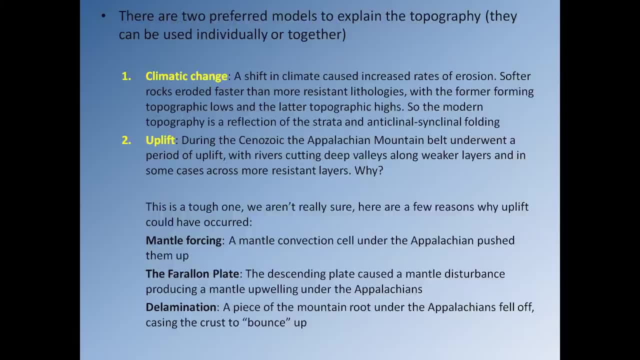 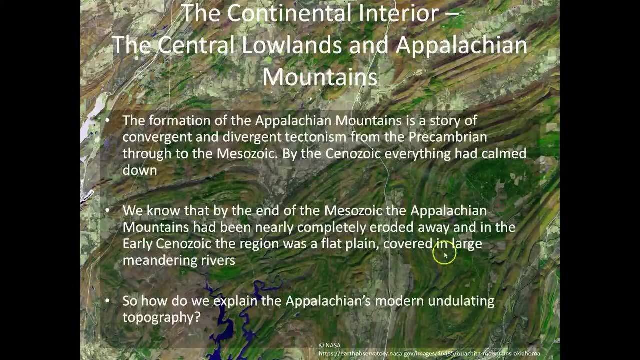 will erode faster, And obviously those rivers will erode the softest rocks most easily. Now, as I'm sure you remember, this area is very heavily filled. There's lots of anticlines and synclines, And so that means the same layers of rock. 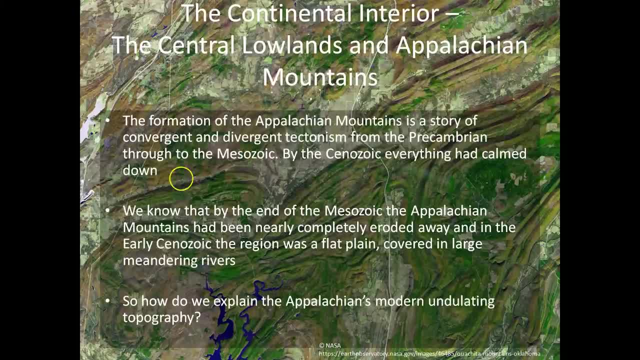 appear again and again, and again. And so this means if a layer of rock- that's repeating itself again and again and again- is relatively soft, it means it will easily erode, And so that will lead to the formation of river valleys. And obviously, if you're forming valleys, 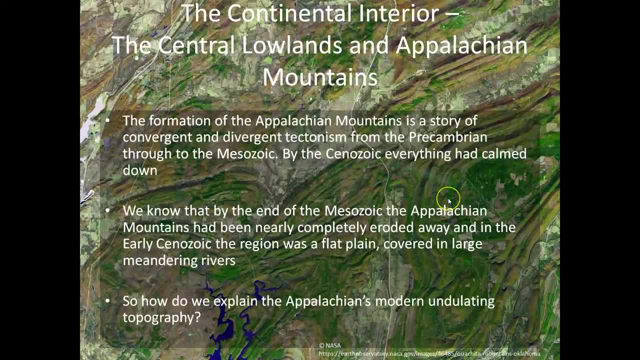 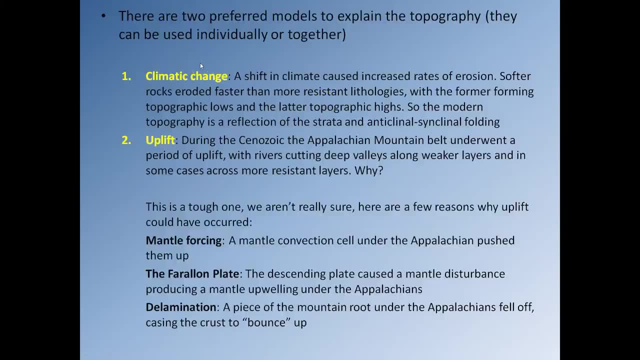 then, either side of the valley, you're going to have areas of raised ground, You're going to have topography. So that's the first possibility. It could just be due to climatic change. The other possibility is that the entire area is currently going up. 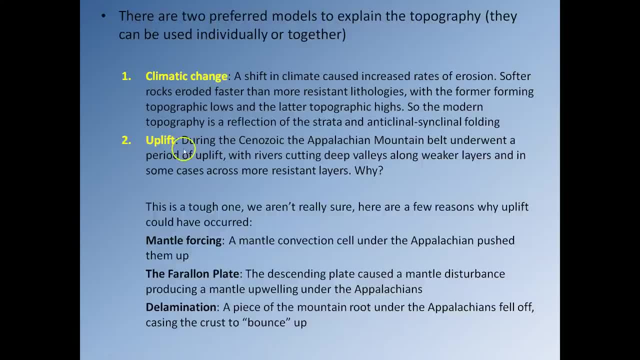 like the western United States. So that suggests that during the Cenozoic, the Appalachian mountain belt underwent a period of uplift, with rivers cutting deep valleys along weaker layers of rock, which goes back essentially to the same basic model as the climate change model. 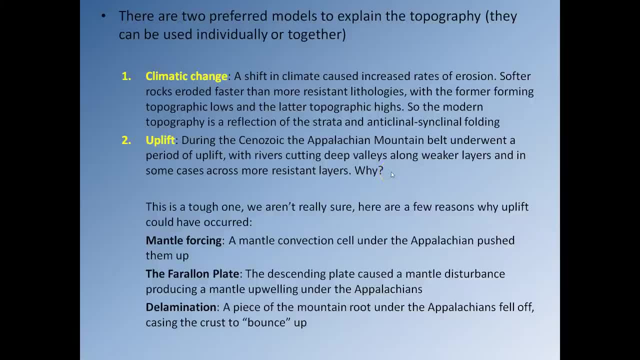 So the question then becomes: why would the area be going up? Well, it's a difficult one, We're not sure, But there are a few possibilities that could explain it. The first one is something called mantle forcing. So if there's a mantle convection cell, 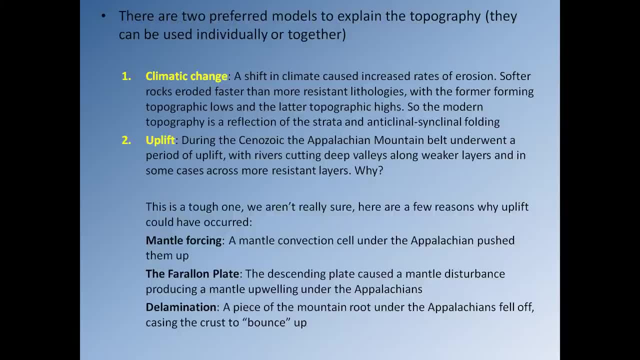 underneath, essentially the eastern United States, and that mantle convection cell is causing mantle rocks to go up. well, obviously, as those rocks, as mantle rocks go up, it causes the lithosphere above to be pushed up slightly, And so one of the suggestions is: 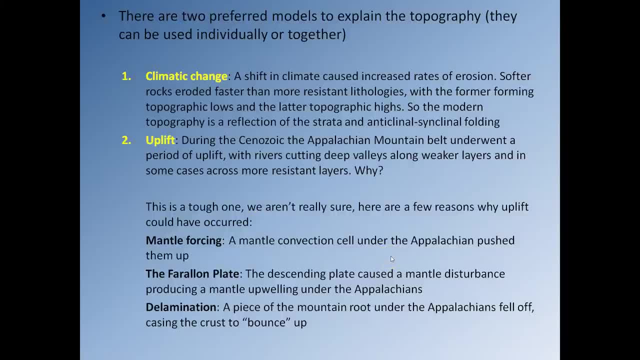 is that, because the mantle rocks are going up, it's causing the eastern side of the United States to be pushed up just a little bit, and that's sufficient to cause the uplift required to produce the topography that we see. Another possibility is that it's due to the Farallon Plate. 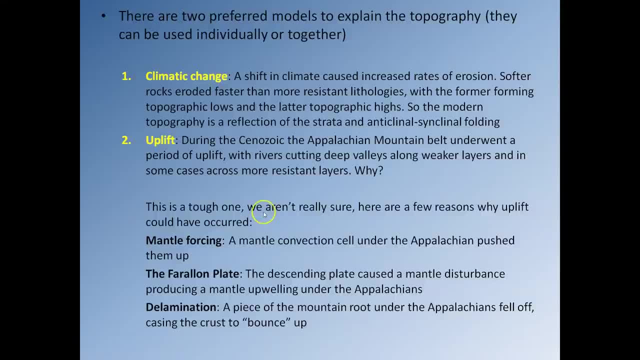 So this piece of oceanic crust that's subducting down into the mantle is causing a mantle disturbance and that once again produces a mantle upwelling, causing the crust in the Appalachian region to be pushed upwards, And the final possibility is a process called 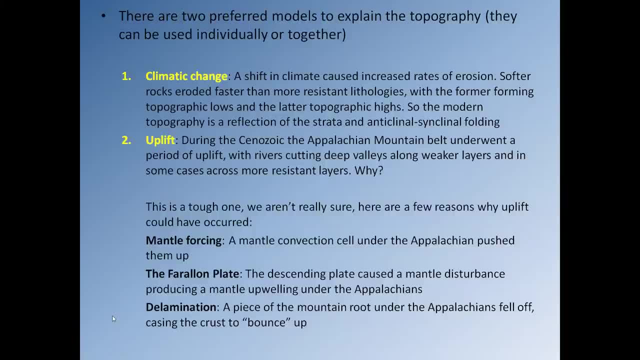 delamination, And that's when a piece of the lithosphere essentially falls off the bottom of the continental crust. Well, that causes the continental crust to suddenly weigh less, and so it bounces up, And once again that would lead to uplift. 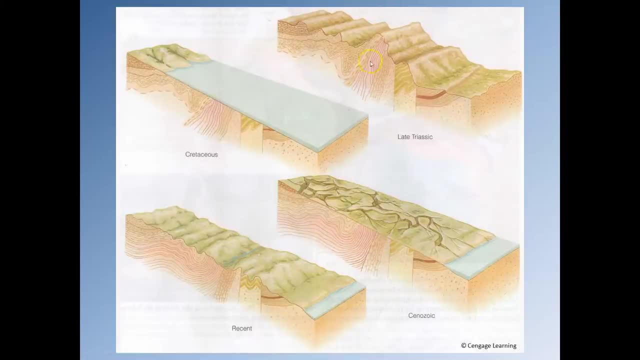 And so this is the situation. During the late Triassic we have topography By the Cretaceous it's completely flat. By the Cenozoic it's covered in rivers, And very recently we have this sudden increase in topography. 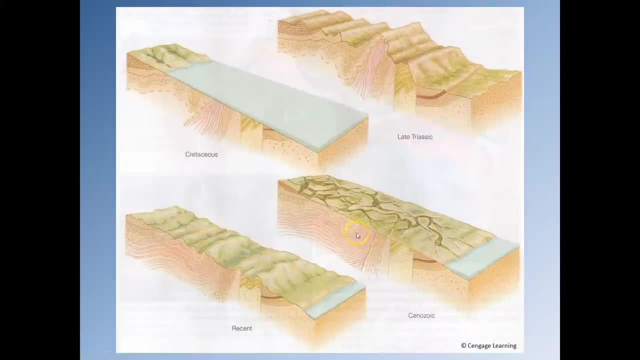 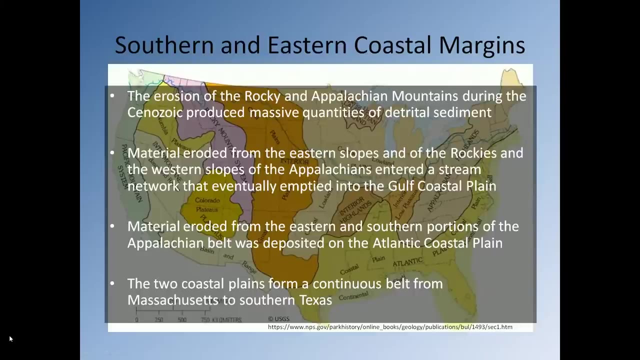 which is either probably due to climatic change or uplift, We're not really sure which. Okay, it's a good place to stop for a minute. So get up, have a walk around and please come back in a few minutes. So the next region we need to deal with. 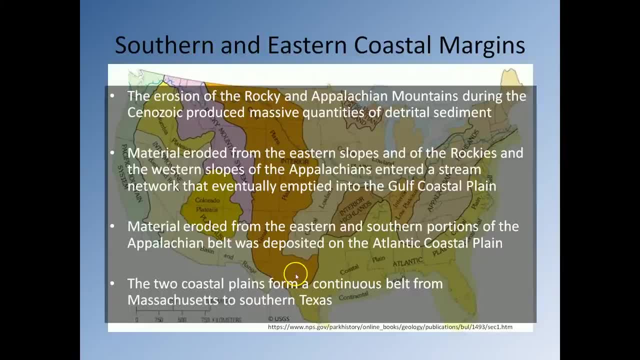 is the southern and eastern coastal margin, So this area down here otherwise referred to as the Atlantic Plain. So obviously the erosion of the rocky and Appalachian Mountains during the Cenozoic produced huge quantities of detrital sediment. So in the case of the Appalachians, 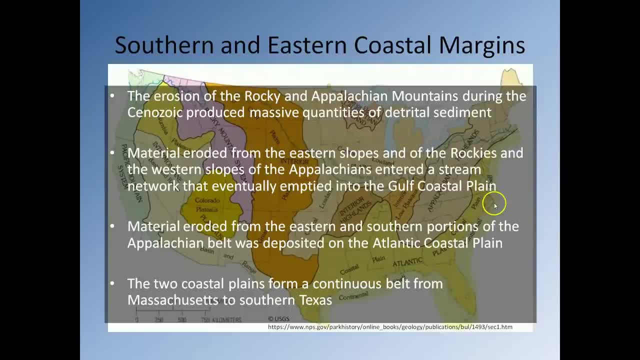 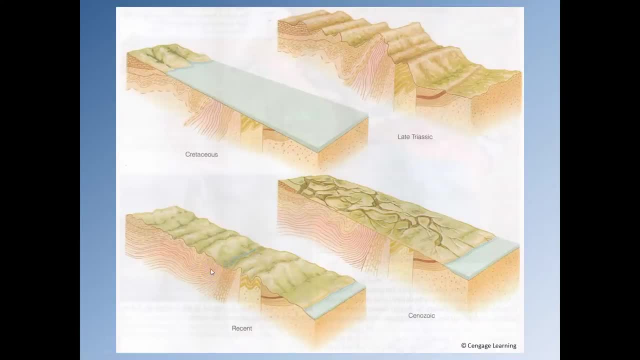 well, they're obviously right here, But obviously that all this- you know, topography that's being produced, as we saw during the more recent times, produces lots of sediment and that sediment has to be deposited somewhere. At the same time, 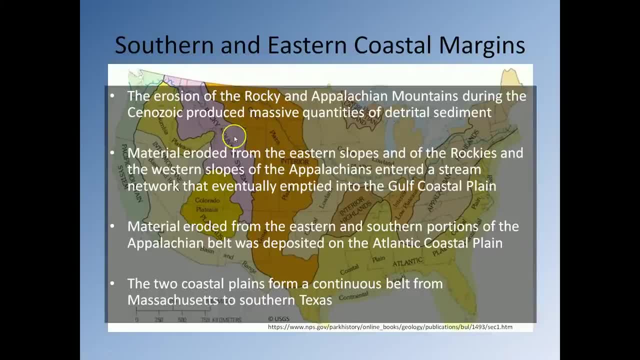 we have lots of rock being eroded over here in the Rockies and it's being transported by these large rivers across the Great Plains and that sediment is going to be deposited in this region around here, either on the Atlantic Coast or over here in the Gulf. 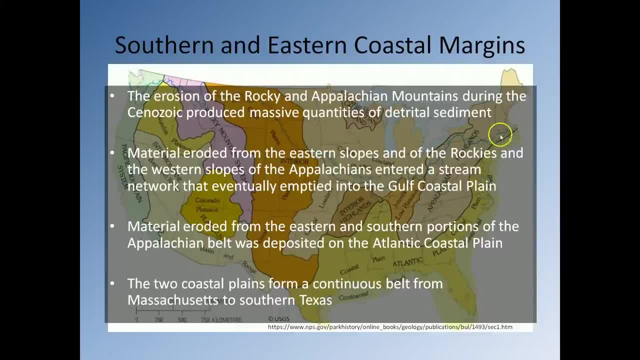 So typically, the material eroded from the eastern slopes of the Rockies and the western slopes of the Appalachians will essentially be focused into rivers that will empty into the Gulf of Mexico. down here, Material eroded off the eastern side of the Appalachian Mountains will typically be deposited. 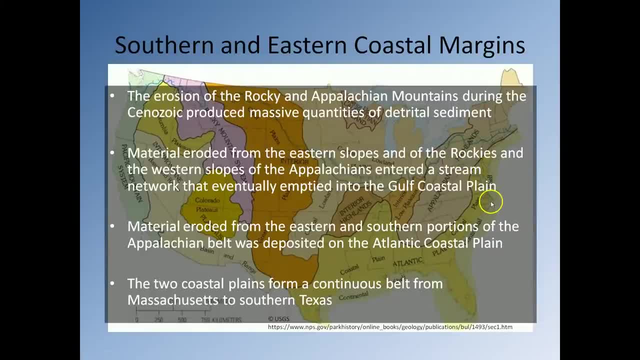 on the Atlantic Coast over here, So the two coastal plains form a continuous belt that stretches from Massachusetts up here, all the way down to southern Texas, And essentially it's a region of deposition. This entire area has been steadily building outwards over time as new sediment is deposited. 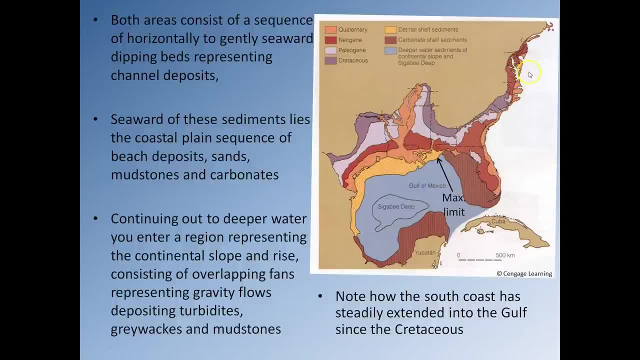 So just to give you some idea, so this is the area essentially along the east coast. So here's Florida, obviously, Here's the Louisiana, Texas coastline over here, And you can see that if we go from the Cretaceous, which is in the deep purple. 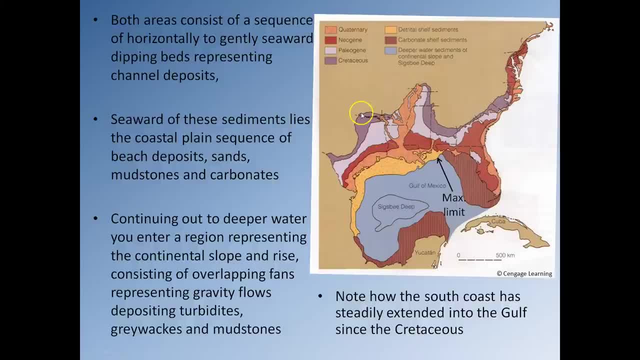 into the Paleogene, into the Neogene and into the Quaternary. we can quite clearly see that the coastline has been steadily building out as sediment is deposited, And this sediment is coming from the erosion of the Rockies and the erosion of the Appalachians up here. 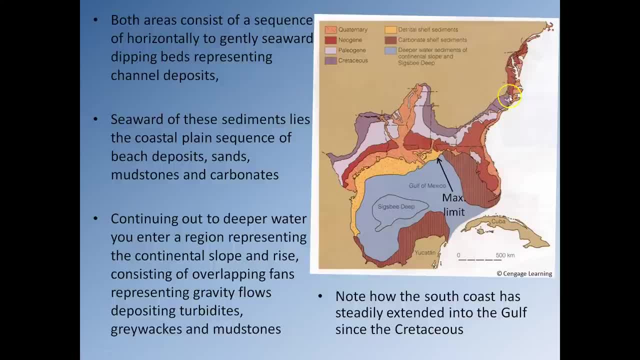 And so this entire eastern seaboard has been building outwards into the Atlantic and into the Gulf of Mexico, And this area here marked out in yellow, that's the region of detrital shelf sediments. Essentially, this area here represents the maximum possible extent. 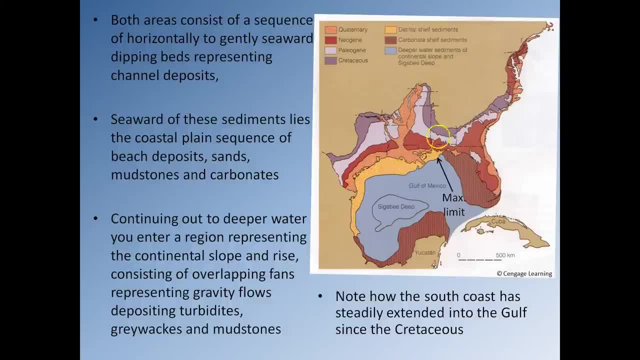 to which the coastline could build out. Essentially, this edge here represents the maximum edge. So over time the coastline could keep building out, out, out, out out until it gets to here, and that's about as far as it can go. 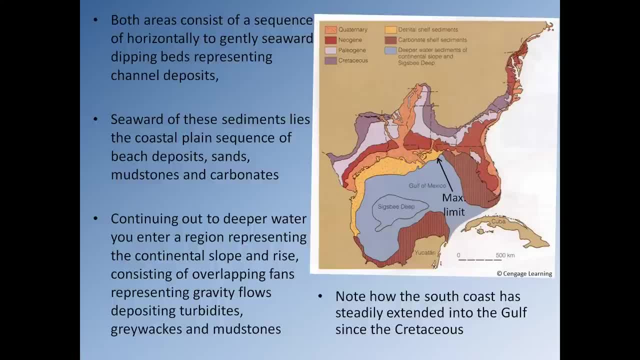 So there's still room for Texas to grow. So both areas consist of a sequence of horizontally to gently seaward dipping beds representing channel deposits. So we have lots and lots of material here that's being deposited into the coastal region by very, very large rivers. 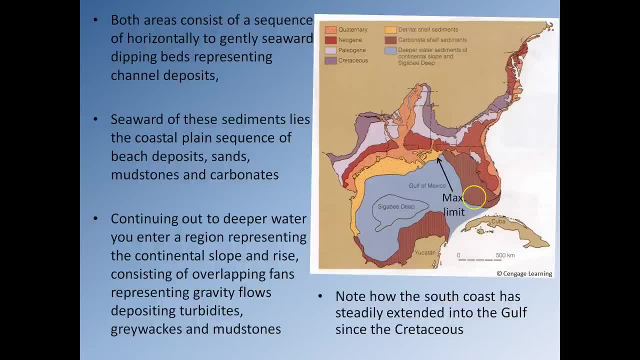 So seaward of these sediments lies the coastal plain. That's essentially the continental shelf, And we get a sequence of beach deposits, sands, muds and carbonates. That's the marine sequence, So the sequence of rocks that we have on land. 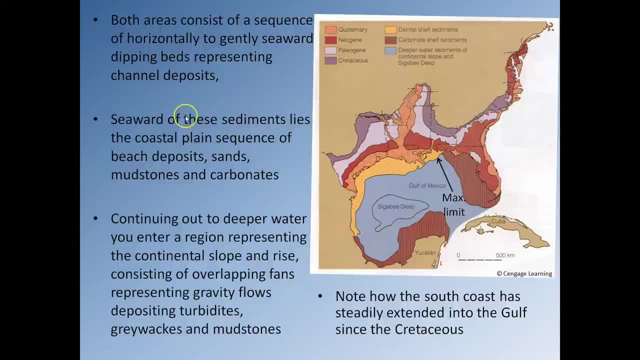 represent rivers And then off the coast we have the classic passive marine sequence: sands, muds and carbonates. So when we continue out into deeper water, we obviously enter a region representing the continental slope. As you come down the continental slope, 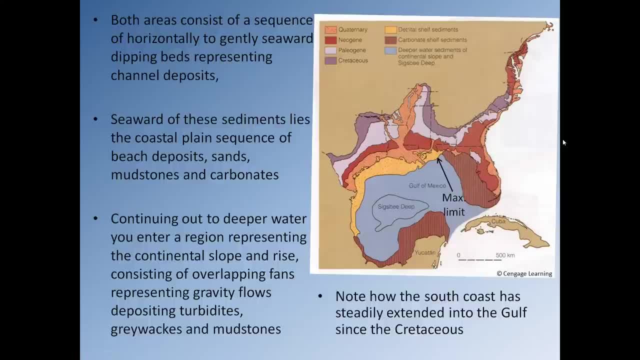 you hit the continental rise And then obviously, as you go past the continental rise, you go onto the abyssal plain. So essentially, these areas here are going to build out as far as they can as long as there is a constant supply of sediment. 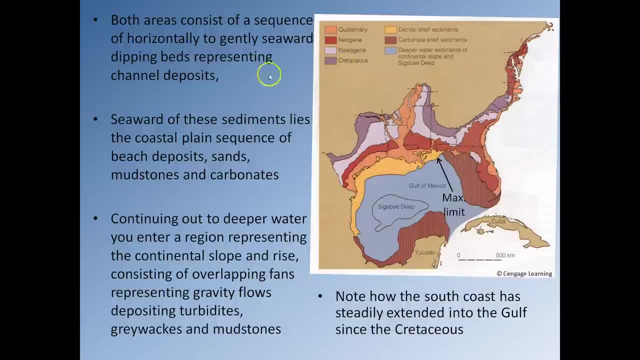 coming in. So as long as the Appalachians are eroding and as long as the Rockies are eroding, producing sediment, the coastline of the east coast of the United States is going to keep building out. So we're going to spend just one second. 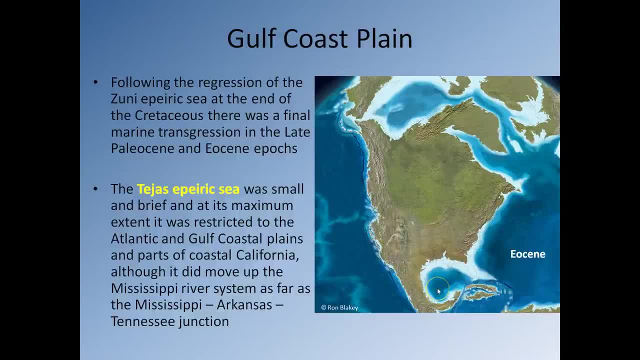 to think about just the Gulf Coast region for a minute. So following the regression of the Zunia Pyrrhic Sea at the end of the Cretaceous, there was a final, relatively small marine transgression in the late Paleocene and early Eocene. 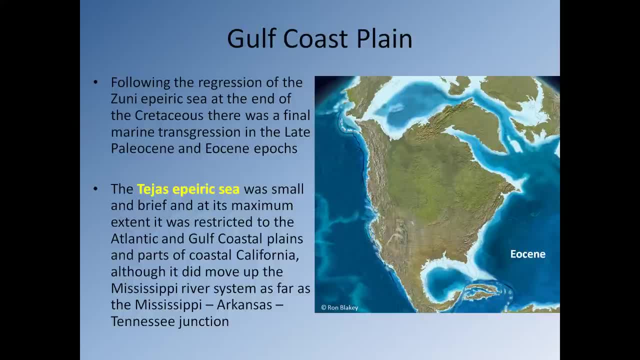 So this is the Tejas Pyrrhic Sea and it was small, it was brief and at its maximum extent it was restricted to the Atlantic and Gulf Coast plains, mostly the Gulf Coast. Also there was a little bit of inundation. 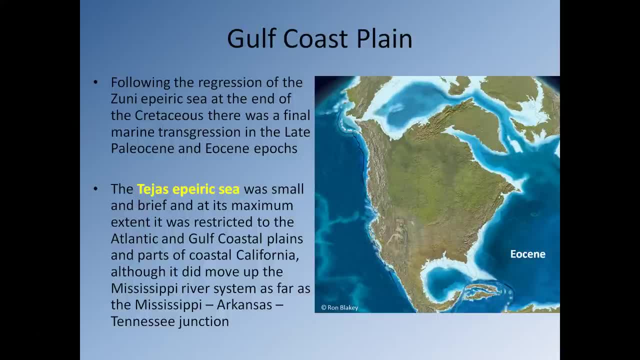 in coastal California, although you know not very much, The most extreme area of inundation is here, so the water moved up the Mississippi Valley and it made it as far as the Mississippi-Arkansas-Tennessee Junction, So a relatively small marine transgression. 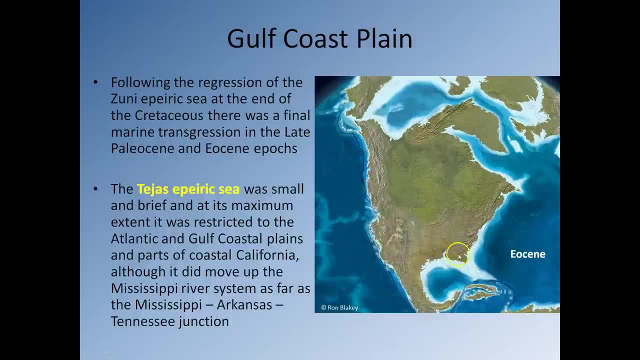 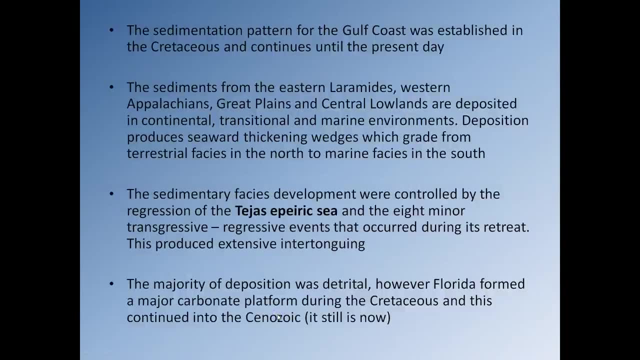 Only really affected the Gulf Coast, a little bit of the Atlantic Coast and a small area over here of California. So the sedimentation pattern for the Gulf Coast was established in the Cretaceous and it continues until the present day. So essentially since the Cretaceous. 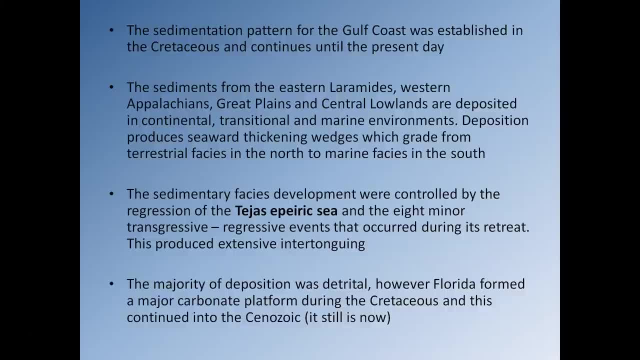 the area's been a passive continental margin, with huge amounts of sediment being deposited from the erosion of the formation of the Rockies and the erosion of the Appalachian Mountains. So the sediment from the eastern Laramides and western Appalachians, Great Plains, central lowlands. 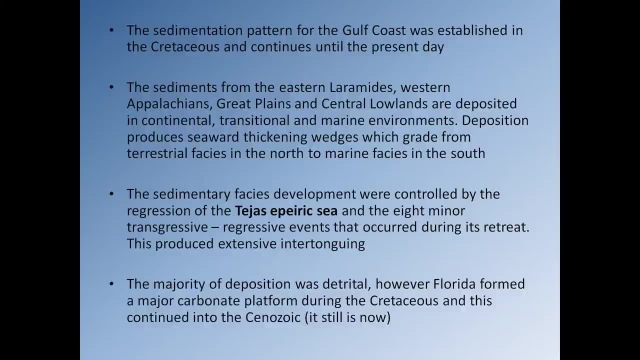 are deposited in continental, transitional and marine environments. Deposition produces seaward thickening wedges which grade from terrestrial fasces to the north and marine fasces to the south. Essentially, that means that if we were to take a line going from essentially 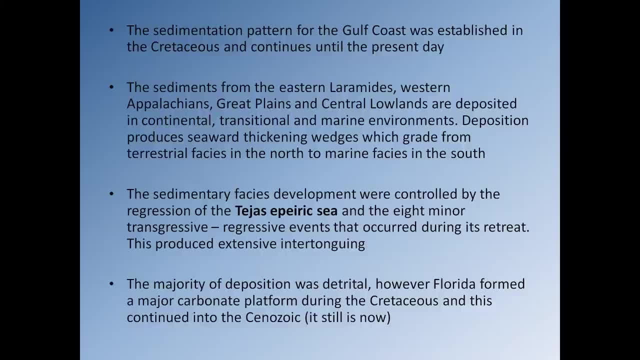 let's say, just north of Houston, going out into the Gulf of Mexico, we would obviously see a sequence of continental sediments, then a sequence of transitional beach sediments and then, obviously, as we went further south, we would head out into the Gulf of Mexico proper. 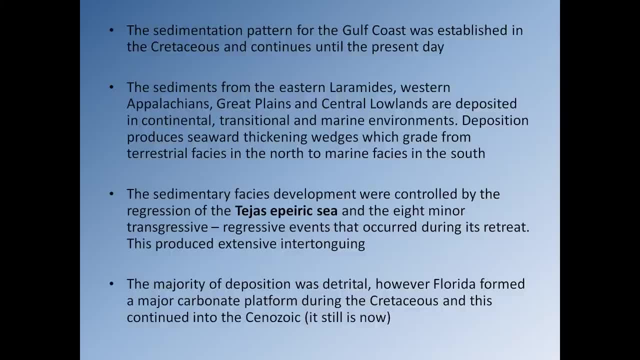 and we would see marine sediments. Makes sense, doesn't it? Also, we would see that the thickness of those layers of sediment would get bigger. so they get thicker as we went south. So, essentially, the continental layers of sediment would be quite thin. 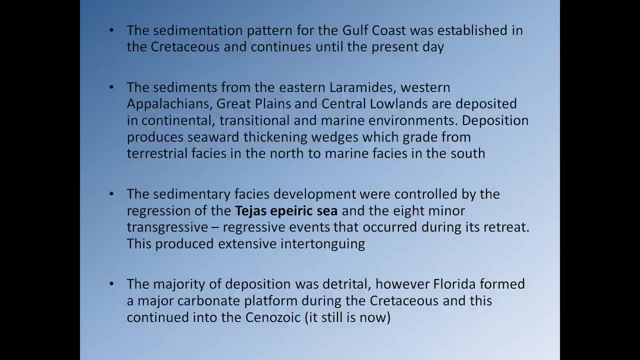 the transitional environments would have even thicker layers of sediment and the marine environment would have even thicker layers of sediment. So the sedimentary fasces developed were controlled by the regression of the Tejas-Epiric Sea and the eight minor transgressive and regressive events that occurred. 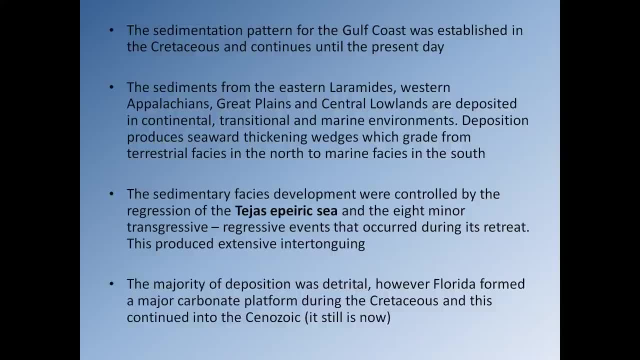 during its retreat. So the Tejas-Epiric Sea was relatively small. it undulated quite a lot. there's quite a few small transgressions and regressions and that caused these fasces to move inland or back out into the ocean. 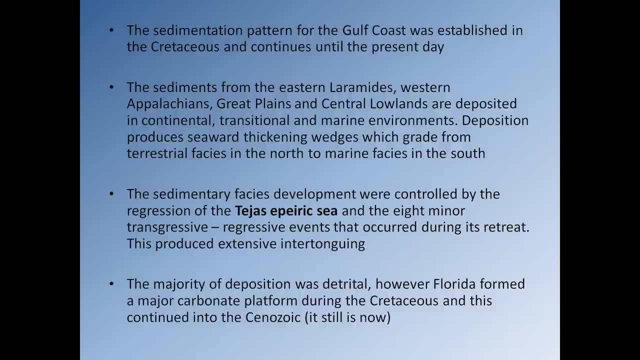 several times And that led to very, very extensive intertonguing. so essentially the contacts between these layers of rock tend to zigzag quite a bit because the coastline went in and out and in and out and in and out. So the majority of deposition. 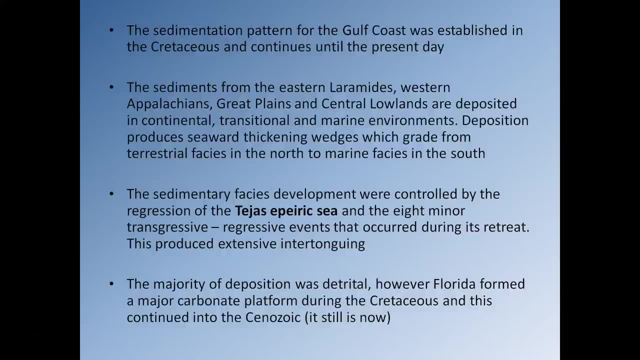 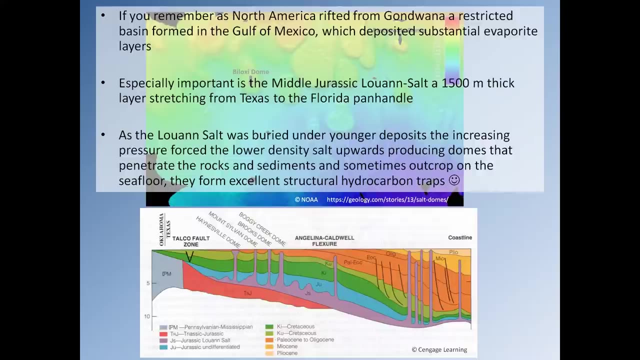 was detrital. however, Florida formed a major carbonic platform during the Cretaceous and this has continued into the Cenozoic. So, if we remember, as North America rifted from Gondwana, we formed a restricted basin. 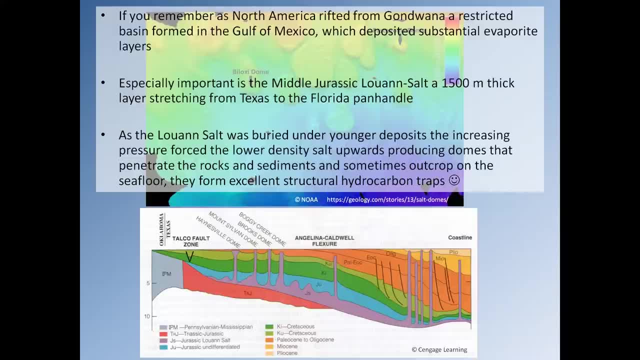 which essentially formed in the area of what is now the modern Gulf of Mexico, mostly the northern portion of the Gulf of Mexico, And this restricted basin deposited substantial quantities of evaporites, And of especial importance is the Middle Jurassic Luan Salt. So Luan Salt is about 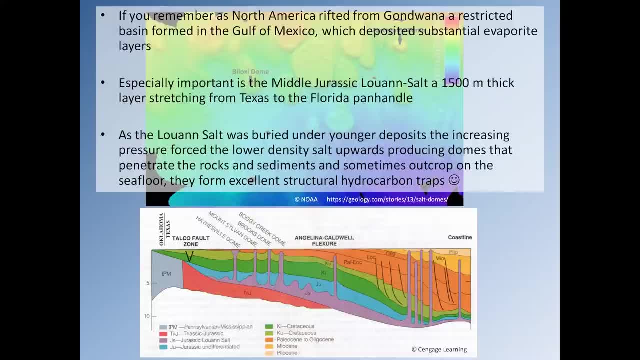 one and a half kilometres thick, and it's a layer that stretches from Texas all the way over to the Florida Panhandle. So why is the Luan Salt important? Well, as the Luan Salt is buried under younger deposits. the increasing pressure. 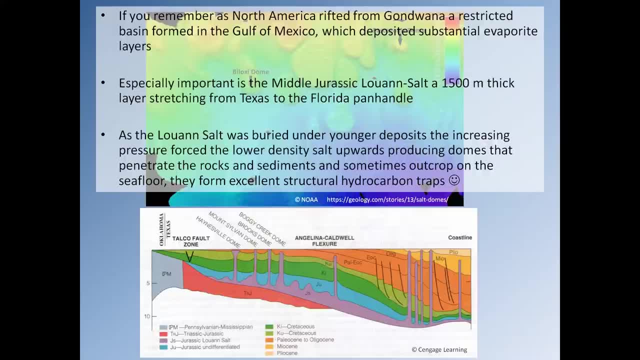 forced the lower density salt upwards. So you might not think it, but salt is actually capable of flowing. So if you take a block of salt and put it under enough pressure, it will start to flow like a liquid, And so this is exactly what's happened. 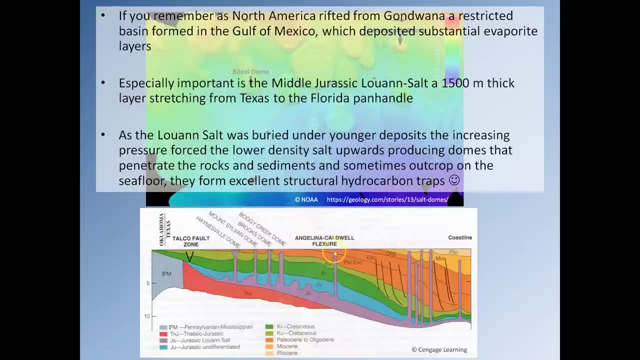 with the Luan Salt. The Luan Salt here is in purple. The weight of all the rocks above it pushing down on it has meant that it has started to flow like a liquid And every time it finds some kind of vertical weakness that it can move up. 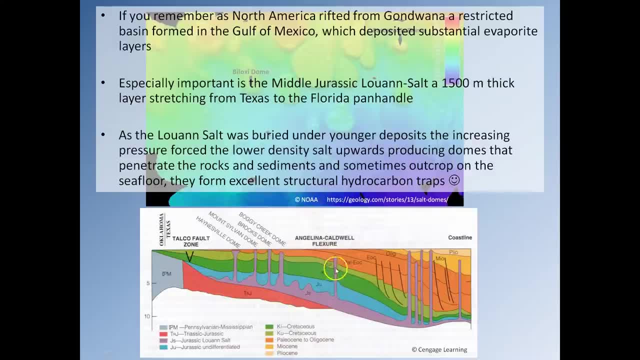 it does So, the salt will go up along any kind of vertical weakness it can find, And it produces structures called salt domes. And so these salt domes are just the result of the salt being squished, and it's being squeezed like toothpaste. 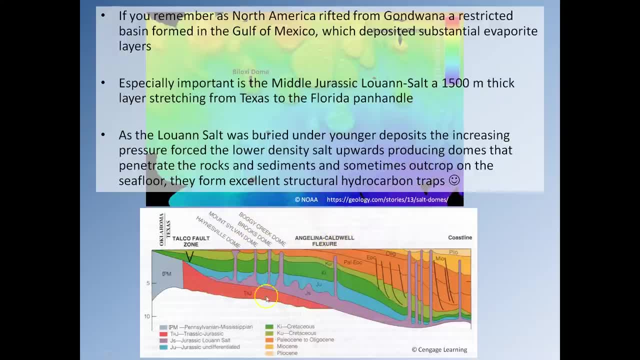 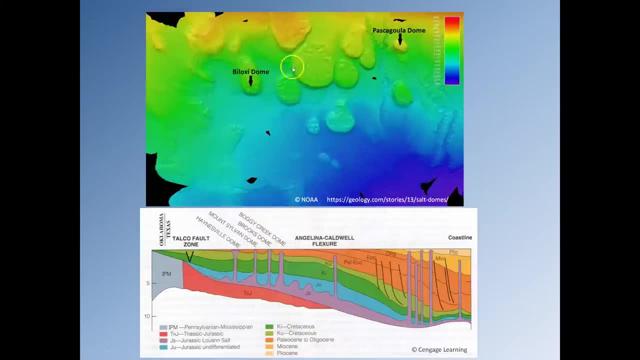 along a vertical weakness, And so we get lots of these salt domes. In that fact, if you look at this picture here- this is a picture of the sea floor of the Gulf of Mexico- you can see all of these circular features. 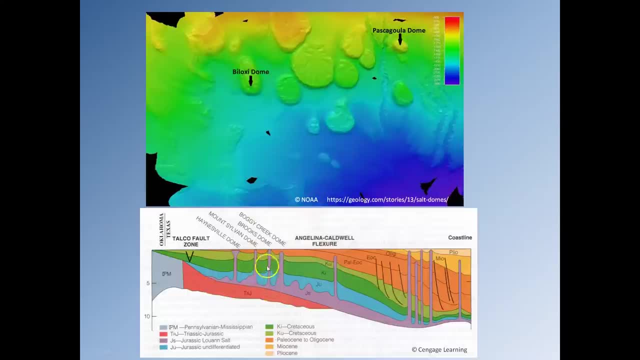 These are all salt domes produced by the Luan Salt being squeezed upwards due to the weight of the overlying rocks and sediment. Now, these salt domes are important because what happens is is when oil forms in these regions, oil will typically go up. 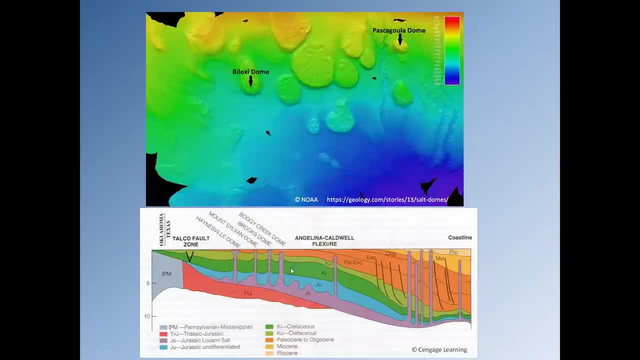 However, once it hits a salt dome, it can't go any further, And so when that happens, the salt dome acts as a trap, Stopping the oil, meaning it can't go anywhere, And so we can come along later and pump it out of the ground. 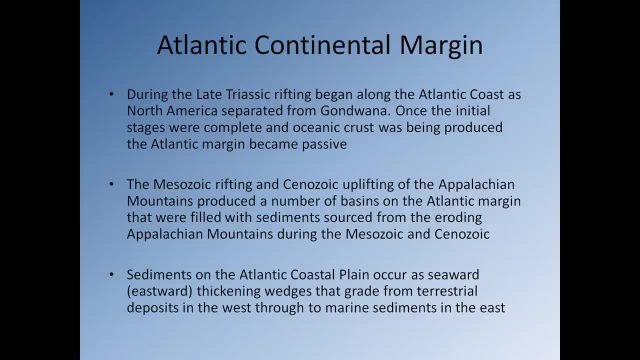 and make huge amounts of cash. Finally, let's think about the Atlantic Continental Margin. So during the late Triassic, rifting began along the Atlantic coast Once again, as North America began to rift off Gondwana. Sorry, should I say? 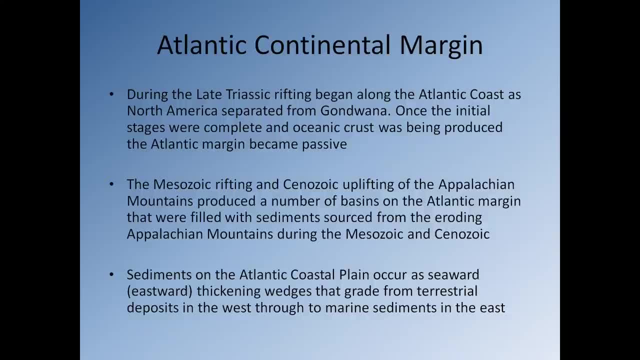 began to: yeah, rift off Gondwana. Did I get myself confused there? Yeah, So once the initial stages were complete, obviously once rifting had finished and we had a body of water in between, we had a nice passive continental margin. 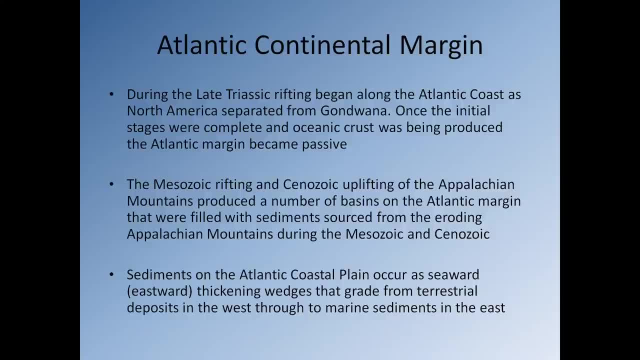 And the Mesozoic rifting and Cenozoic uplift of the Appalachian Mountains produced a number of basins on the Atlantic margin that were filled with sediment sourced from the eroding Appalachian Mountains during the Mesozoic and Cenozoic. So you know the extension. 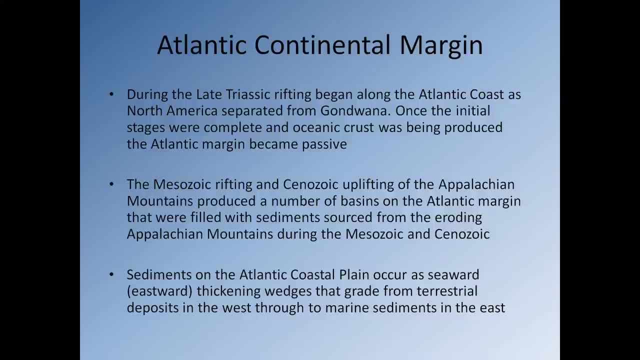 produced lots and lots of you know, a rather large set of rift basins. those filled with sediment from the eroding Appalachians And sediments on the Atlantic coastal plain occur as seaward, so eastward, thickening wedges. So just like the sedimentary layers, 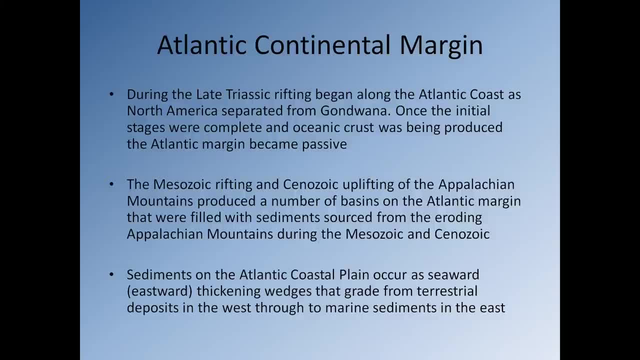 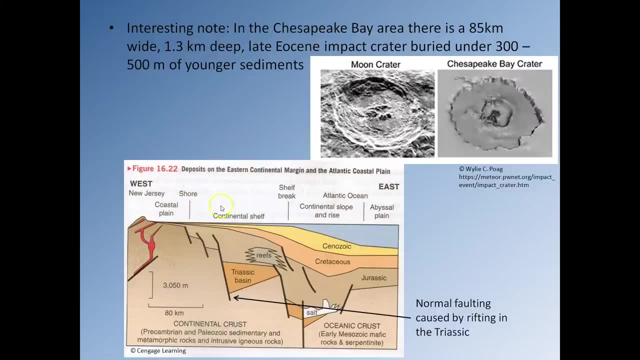 off the Gulf Coast And they grade from terrestrial deposits in the west through to marine deposits in the east. So we have terrestrial deposits over here on land grading through transitional deposits into marine deposits And we can see the layers of sediment start off relatively thin. 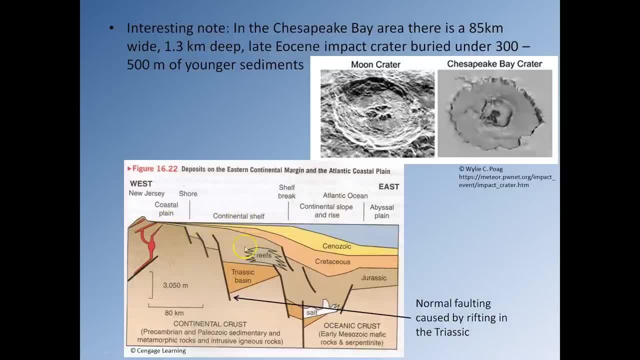 and they get thicker as we head out into open water. So we have essentially a thickening sequence of sedimentary rocks which produces a kind of roughly triangular shape. So the triangle's very, very thin over here and it gets broader as we come out over here. 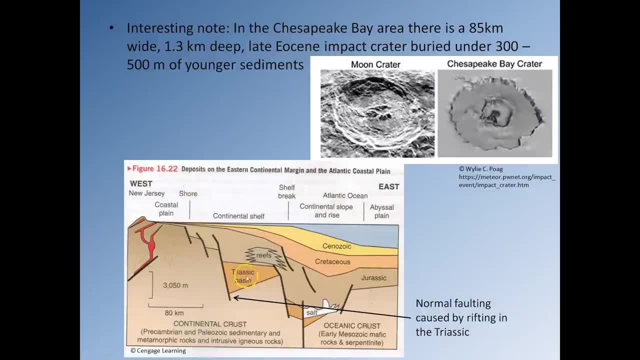 So we can also see that the entire area has got lots and lots of big normal faults cutting it. Those are related to the Triassic rifting which separated North America from Gondwana. One final interesting fact before we call it a day.